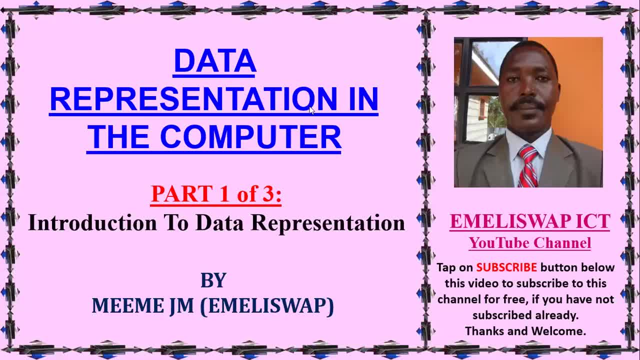 Hello, my dear students and the rest of the learners, Welcome to this presentation in which we are going to be discussing, or learning about, data representation in the computer. This is part one of a three-part series of presentations in this topic. The title of this presentation is Introduction to Data Representation. 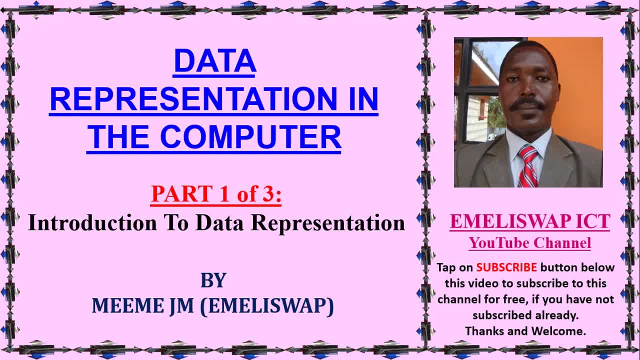 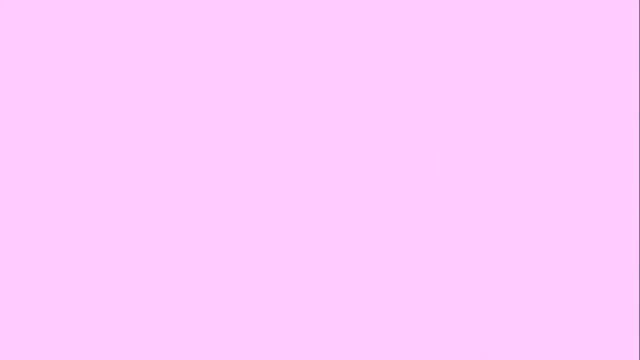 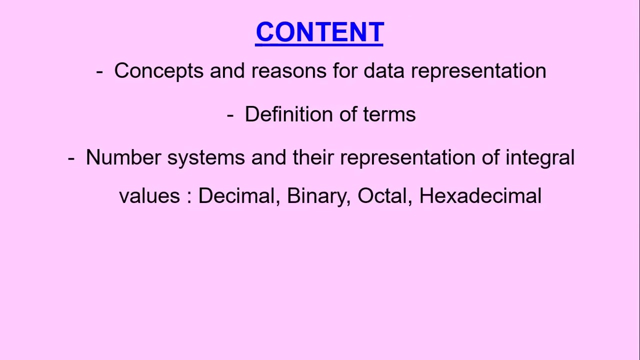 My name is Mehmet YM, or you can simply call me Emily Swap. In this presentation we shall look at the concepts and reasons for data representation. Then we shall look at definition of terms that are used in data representation. Then we shall look at number systems and their representation of integral values. 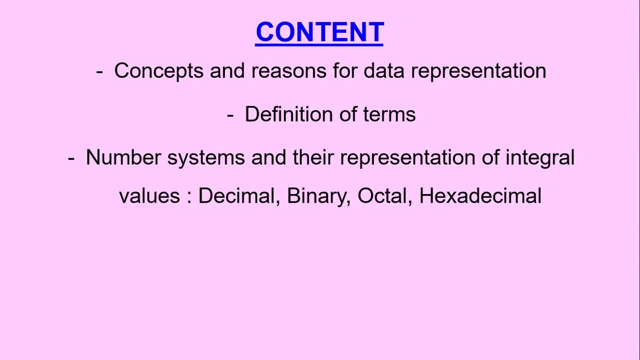 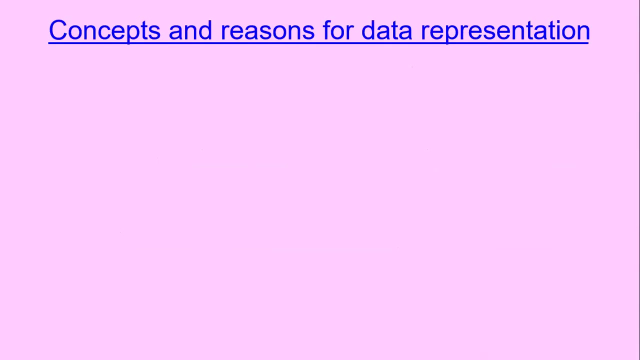 And our focus will be on the decimal, Binary, octal and hexadecimal. We shall also look at symbolic representation, with our focus being on BCD, FC-DIC and ASCII. Let's now look at the concepts and the reasons for data representation. 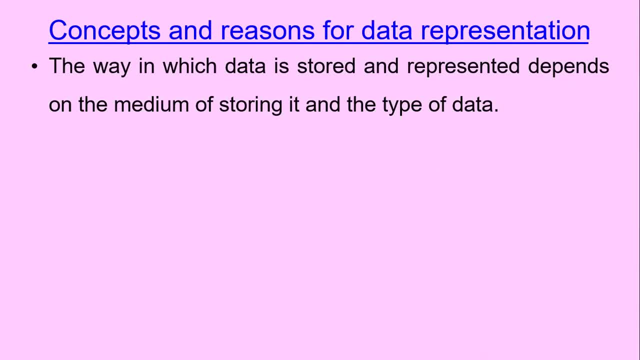 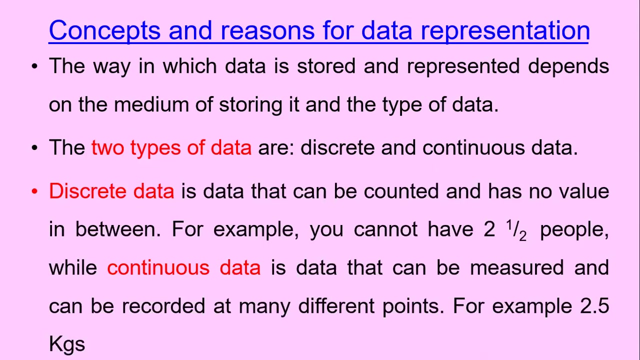 The way in which data is stored And represented in the computer Depends on the medium of storing it and the type of data. The two types of data are discrete data and continuous data. Discrete data is the data that can be counted and has no value in between. 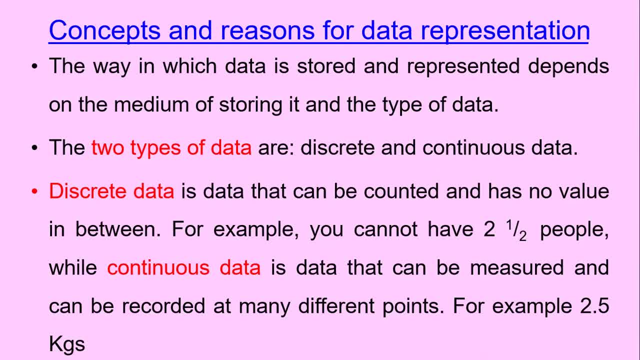 In other words, This is data, data that does not have any fractions or any decimal points. For example, you cannot have two and a half people, You can't have 2.5 people, While continuous data is data that can be measured. 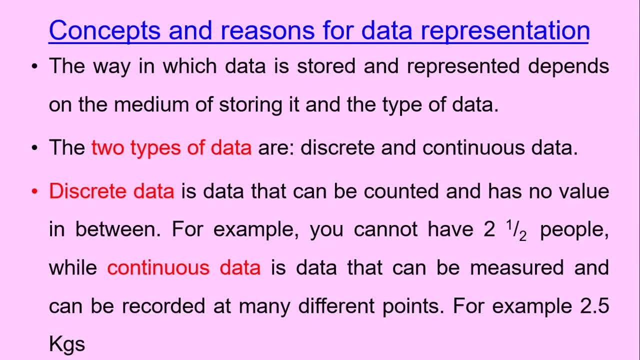 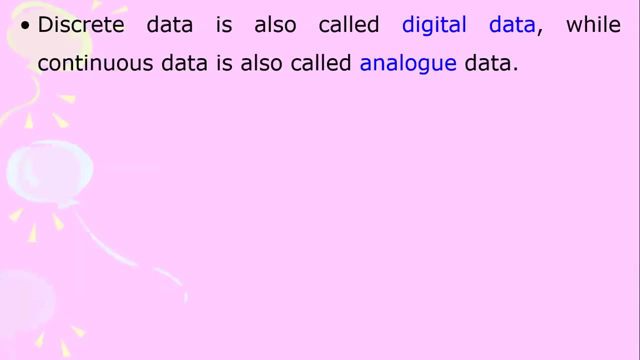 and can be recorded at many different points, For example, 2.5 kilograms. In other words, continuous data is data that contains decimal places or fractional parts. Discrete data is also called digital data, while continuous data is also called analog data. 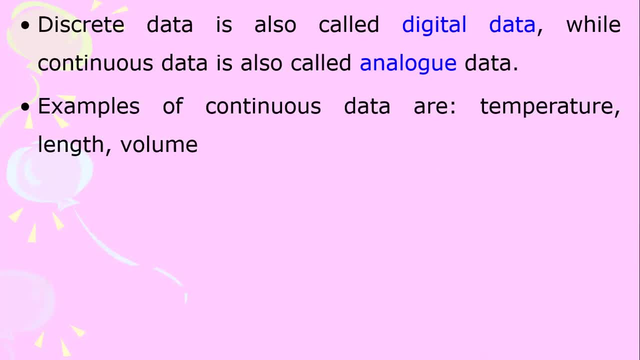 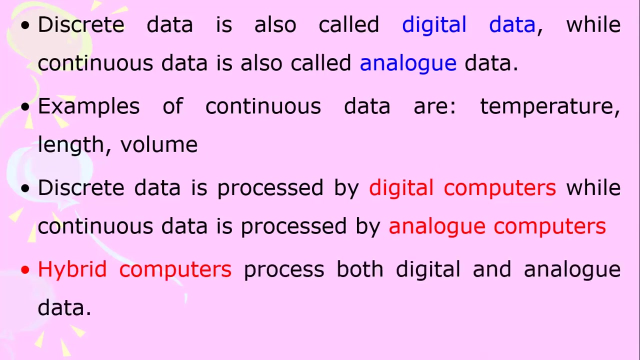 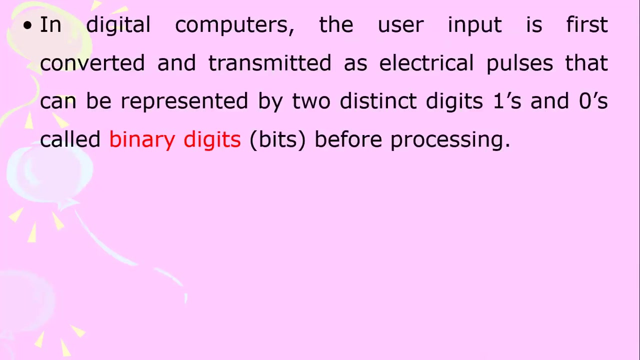 Examples of continuous data are temperature, length, volume, among others. Discrete data is processed by digital computers, while continuous data is processed by analog computers. However, hybrid computers process both digital and analog data. In digital computers, the user input is first converted and transmitted as electrical pulses. 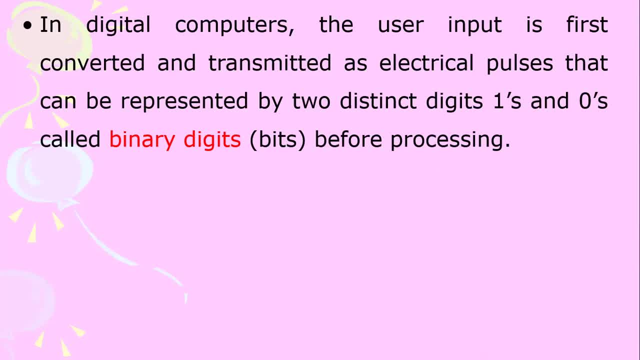 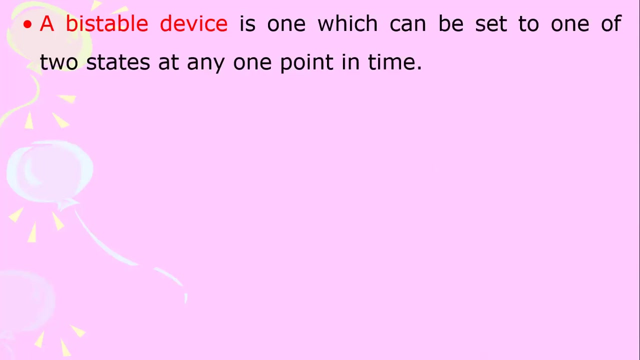 that can be represented by two distinct digits, ones and zeros, which we normally call the binary digits, or bits. before processing, A computer consists of a number of two states, or bistable devices that process and store the data. A bistable device is one which can be set to one of two states at any one time or at any one point. 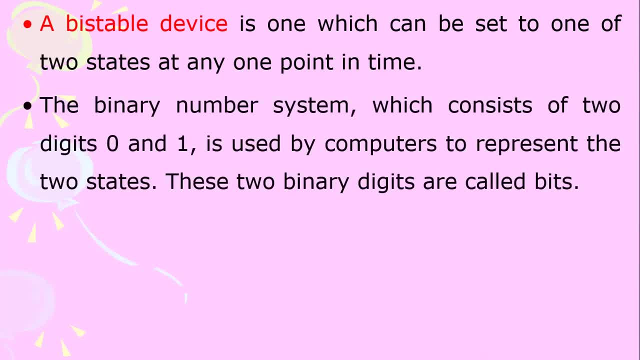 in time. The binary number system, which consists of two digits, zero and one, is normally used by computers to represent the two states. These two binary digits are called bits. therefore, the term bit is an acronym or a short form for binary digits. 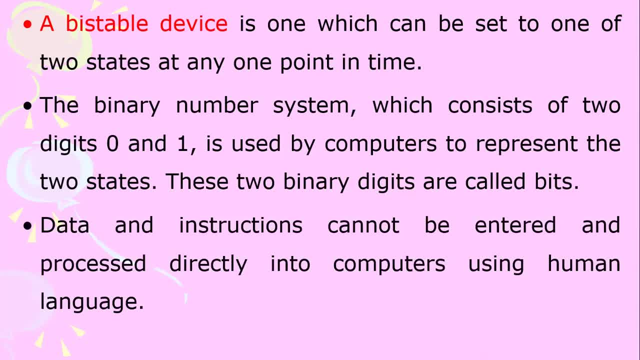 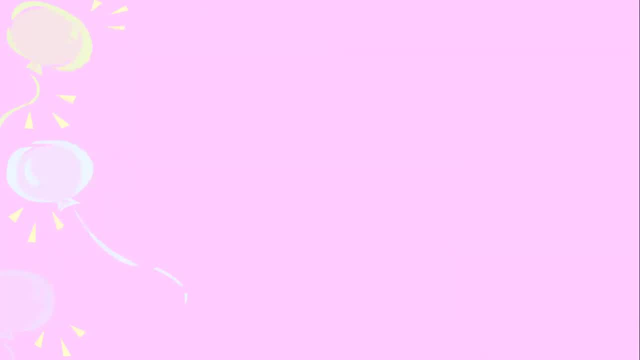 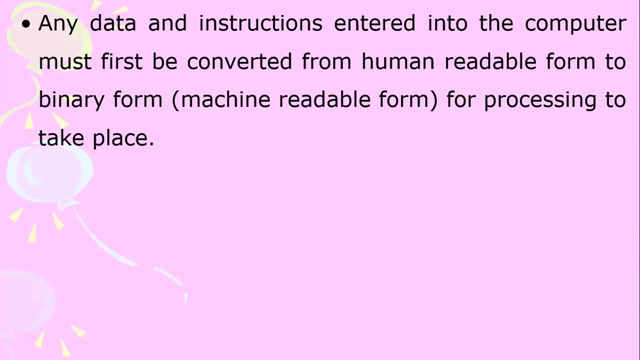 Data and instructions cannot be entered and processed directly into computers using human language, And for that reason any data and instructions that are entered into the computer must first be converted from human-readable form to binary form, or what we call the machine-readable form, for processing to take place. 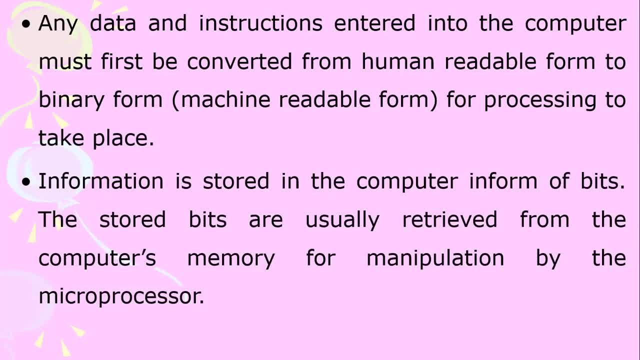 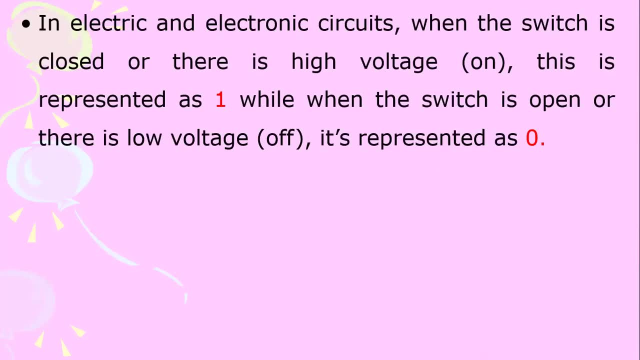 Information is stored in the computer also in form of bits. The stored bits are usually retrieved from the computer's memory for manipulation by the microprocessor In electric and electronic circuits. when the switch is closed or there is a high voltage, that is, the socket is on, this is removed. 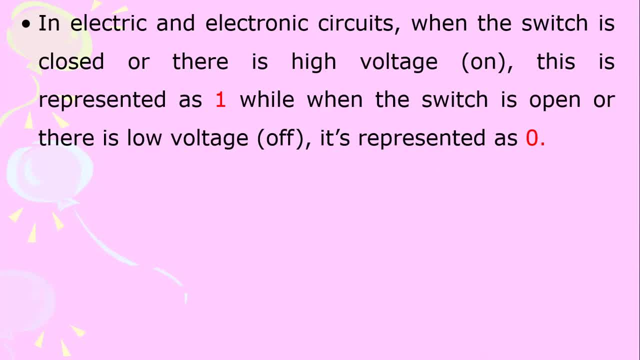 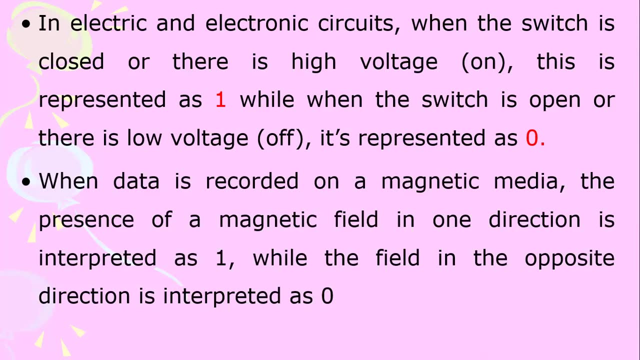 Likeставляp twoopa as one. the i그� Ricky a squ oriental context: Mā Heat. When the switch is open or there is low voltage or no voltage flow, that state is represented as a zero. When data also is Earth-condon on a magnetic media. 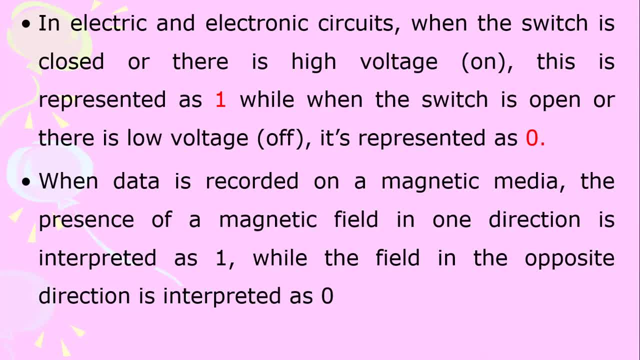 the LEGO of a magnetic field in one direction is represented as a one, while the field in the opposite direction indicates zero. William's dé Jr, which is directly scattered between billion and pupils, is the colocal portion is represented as a Europe, while the 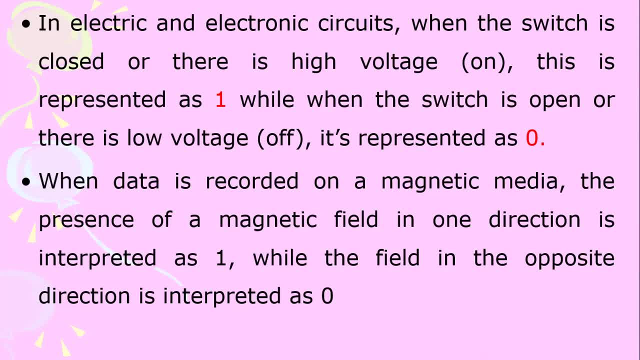 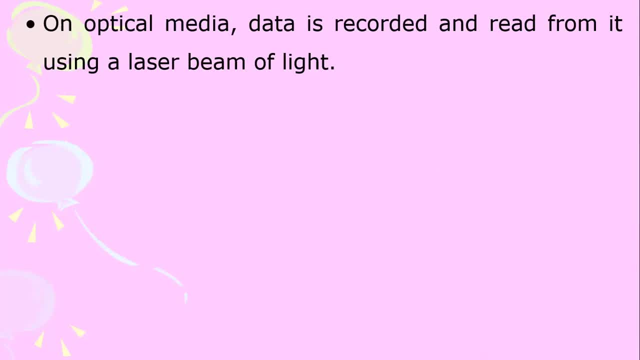 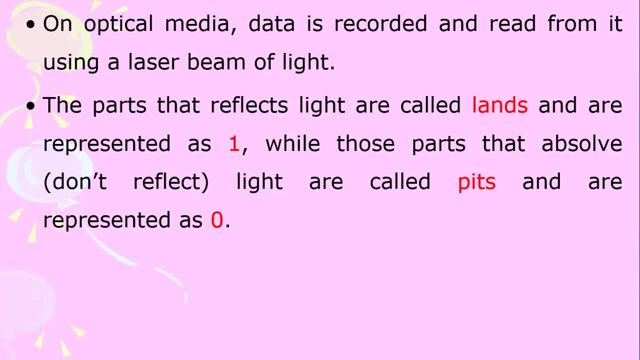 beam is represented as zero On optical media. data is recorded and rendered from it using a laser beam of light. The parts that reflect light are called lines and are represented as one, while those parts that absorb or don't reflect light are called pits and are represented as zero. 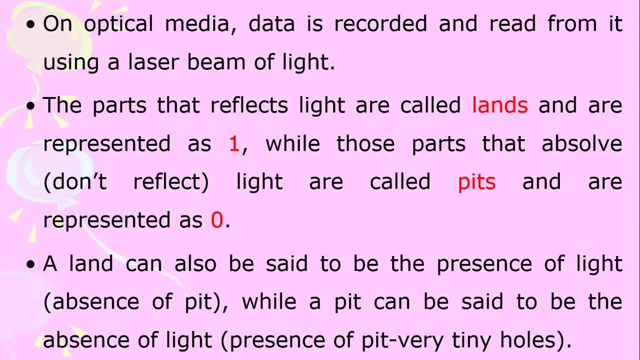 A land can also be said to be the presence of light. that is, or absence of light or absence of pit. I repeat: a land can also be said to be the presence of light. That is absence of light. A land can also be said to be the absence of pit, while a pit can be said to be the 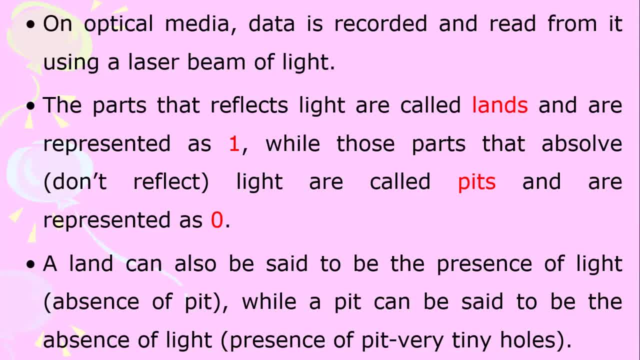 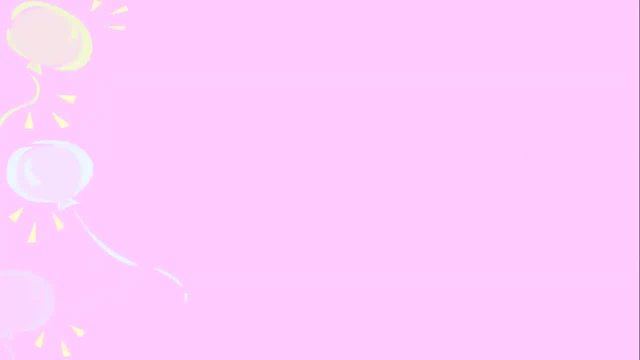 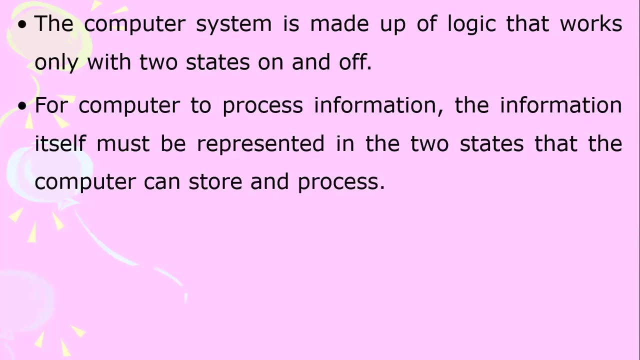 absence of light, That is, presence of pit, very tiny holes. The computer system is made up of logic that works only with the two states on and off. For computer to process information, The information itself must be represented in the two states that the computer can store. 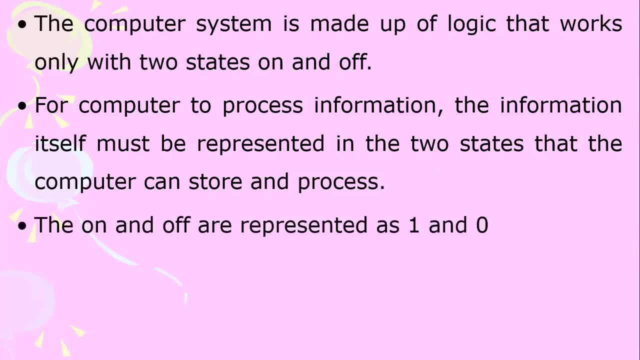 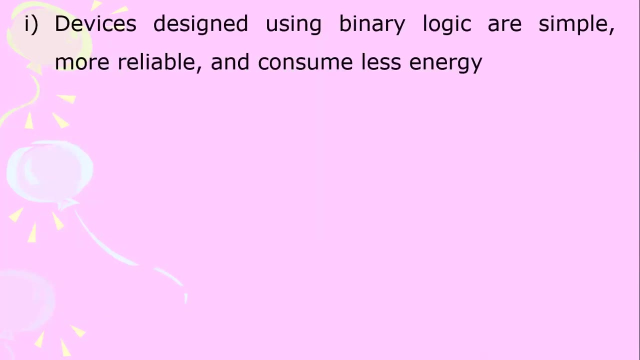 and process. The on and off are represented as one and zero. So some reasons as to why binary systems are used in computers and in other fields in digital technology. Number one: devices designed using binary logic are simple, more reliable and they consume less energy. 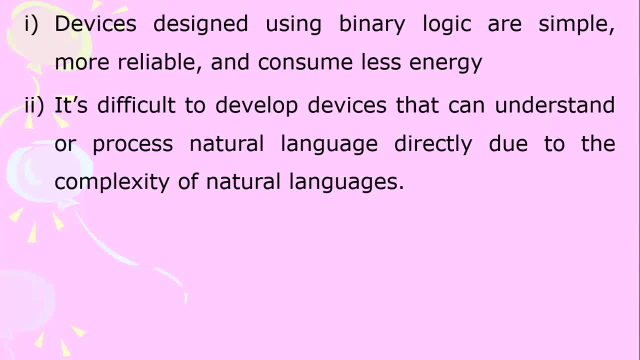 Number two: it's difficult to develop devices that can understand or process natural language directly, due to the complexity of natural languages. Number three: devices that read, process and process are not the same as the devices that read, process and process. 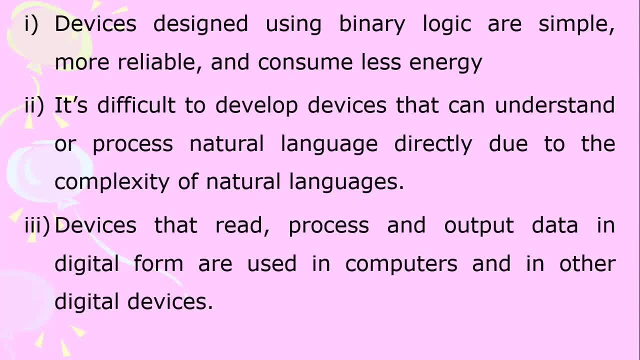 Number three: devices that read, process and process are not the same as the devices that read, process and process, Or operations and output data in digital form are used in computers and in other digital devices. My dear students and the rest of the learners, 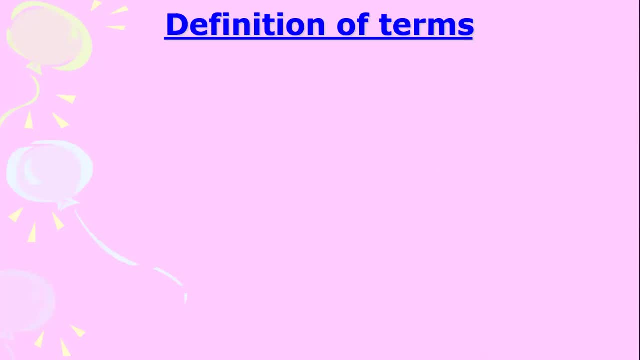 That is why number systems of data representation in the computer is key and you have seen the importance of binary digits. when you know how to read the data in the digital environment, you know how to read the data in a digital environment. This is why binary systems and data are used in a computer. 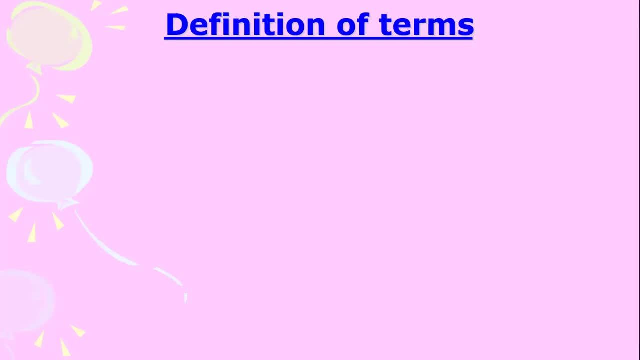 what we are calling the on and off, presence or absence of electricity or electrical signals, pits and lands, ETC. Let's now look at some of the terms that we use when we are talking about or referring to data representation in computing. We commence with the term. 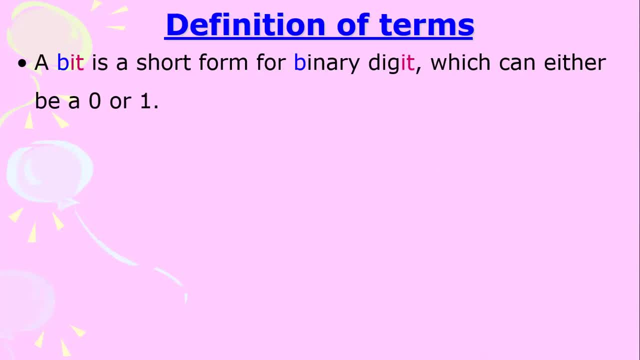 that I have already mentioned several times in this introductory section, which is bit A bit just. as I have said, is a short form for binary, B for binary digit, IT for digit, which can either be a zero or a one. 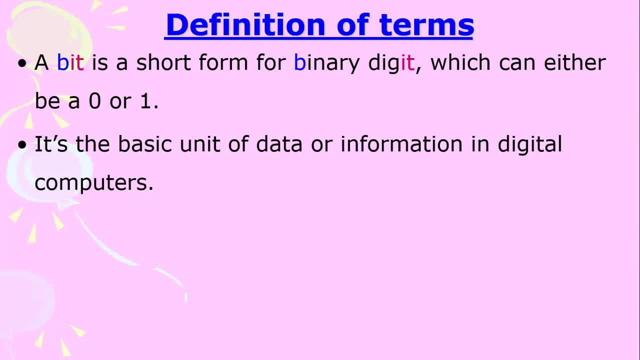 It's the basic unit of data or information in digital computers. A nibble, on the other hand, is a group of four bits, which is normally a half of a byte. An example is one, one zero, zero. These are four bits and this series. 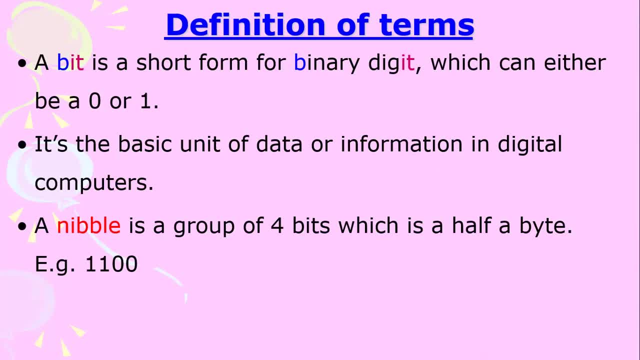 or this representation contains one ones, and that is, two ones and two zeros. A byte is therefore a group of eight bits used to present a character. An example is one one zero zero, One one zero, zero, zero, zero, zero, one. 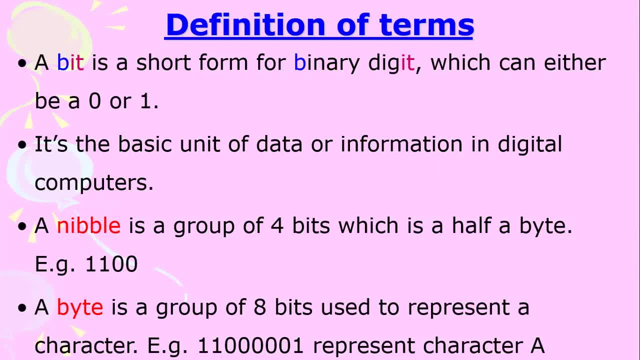 This represents a character which is, in this case, character A. Many MPO students and rest of the learners may encourage you not need to worry about how we arrive at these bits, because you are going to discuss in depth and I will demonstrate and illustrate how we arrive at various numbers. 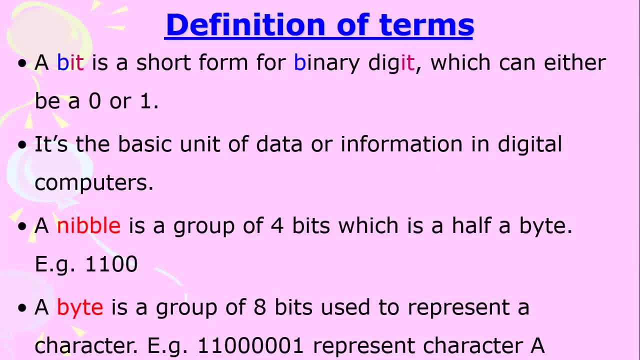 in my next presentations, which are data representation in the computer, part two of three and part three of three. Therefore, make sure that you have visited the YouTube channel by the name MLSwap ICT to access the part two and the part three of presentations in this series. 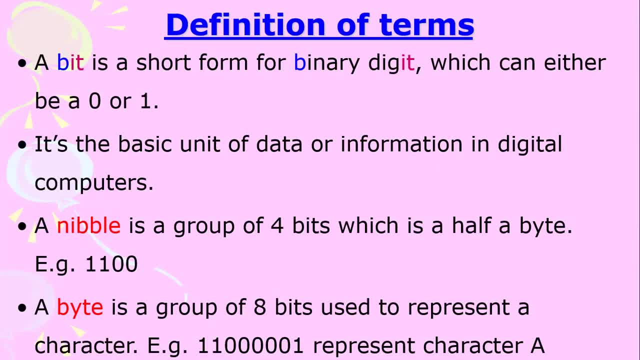 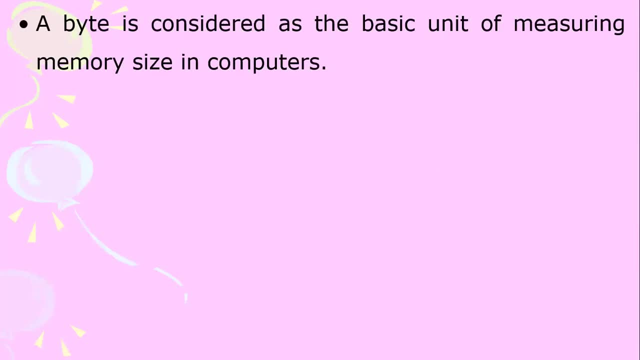 so that you can gain better understanding of the concepts. in addition to data representation in the computers, A byte is considered as the basic unit of measuring memory size in computers. A WAND is a group of either one or more bytes and is the largest amount of memory that the computer can handle. 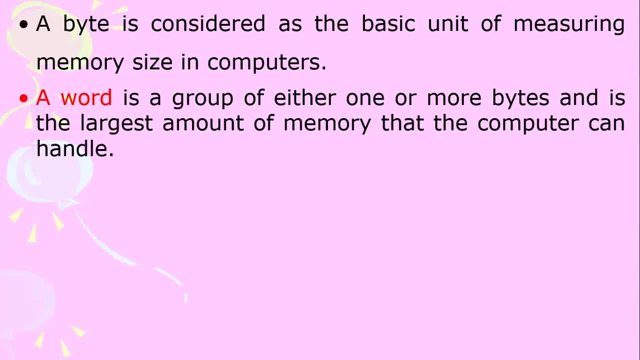 Hopefully you have found the information to beас Shadowsky. You can refer to a byte as a character, while a group of characters can form a WAND returns To a WAND. returns Zum Beispiel, Z Killer Z, Similar to Z-permanent. 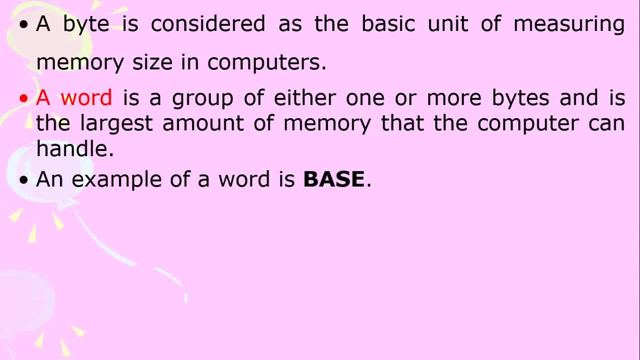 The word is base Base. Base is a word composed of four characters: Character B, character A, character S, character E, Or for those modern kings we can say it is character B, character A, character S and character E Base. 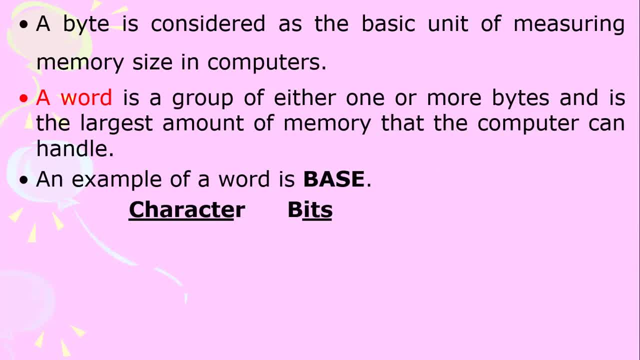 Let's look at each of these characters and its respective bits. Character B is represented In form of binary digit as 1, 1, 0, 0, 0, 0, 1, 0.. A is 1, 1, 0, 0, 0, 0, 0, 1.. 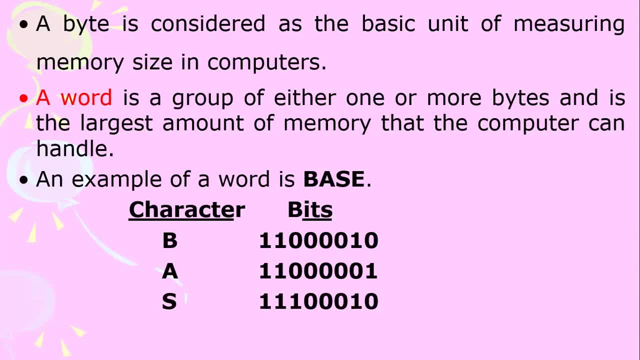 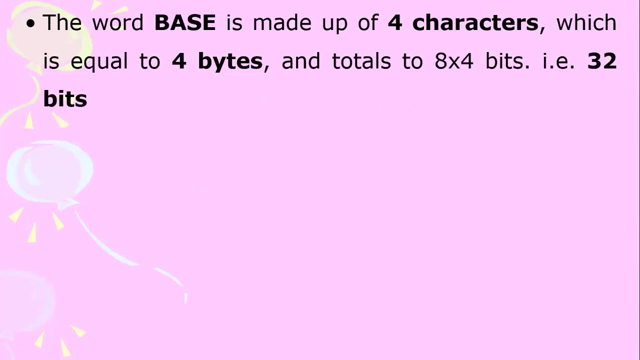 S is bits 1, 1, 1, 0, 0.. E is 1, 1, 0, 0, 0, 1, 0, 1.. The word base is therefore made up of four characters, which is equal to 2,, 2, 4 bytes. 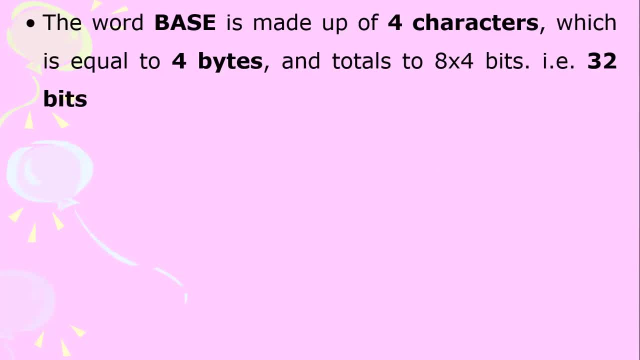 Why. I have already said that a single byte, a single byte is equal to a single character And therefore byte and character are one and the same thing. Byte One byte is equal to one character And therefore four characters: 1.. 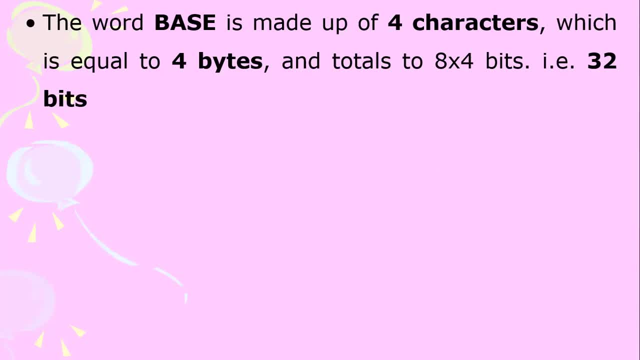 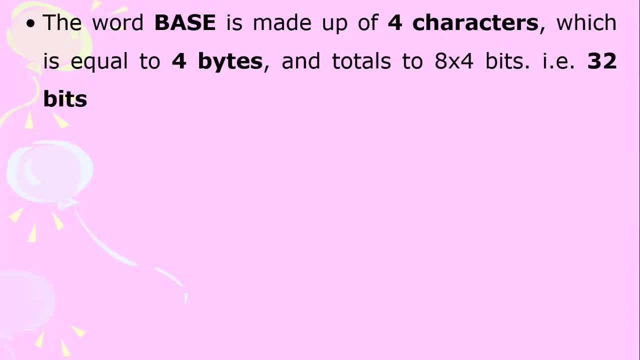 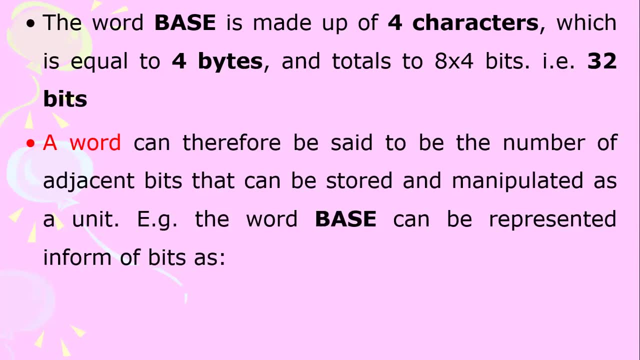 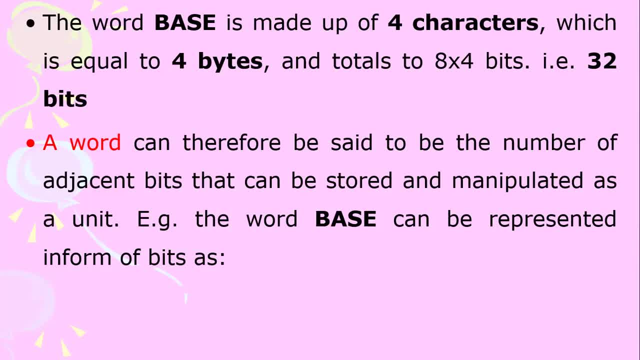 example, the WAND base can be represented in the form of bits as: 1 1 0 0 0 0, 1 0 1 1 0 0 0 0 0, 1 1 1 1 0 0 0, 1 0, 1 0 0 0 1 0 1. 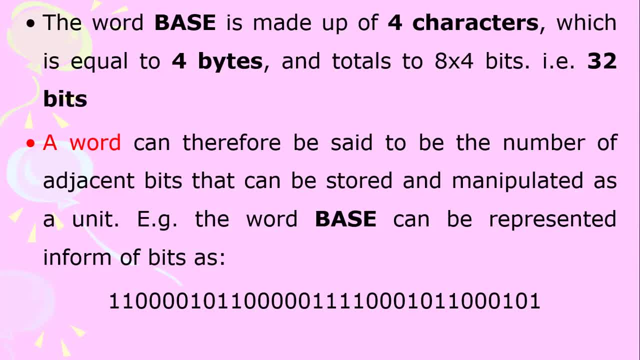 0.. Those are a series of that, two bits, organized based on the arrangement on the WAND base. Therefore, in the series of bits we have the first eight bits representing BOO or BEE. The next sequence of eight bits represent AEE Or the next. 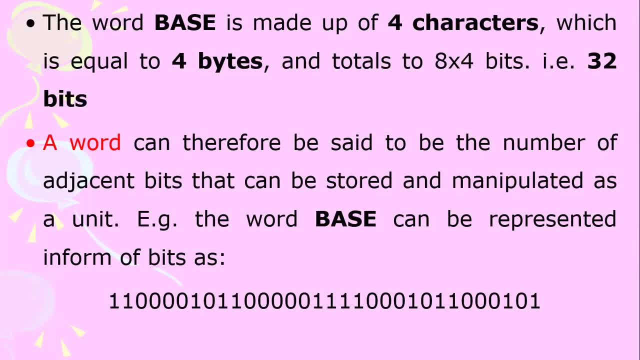 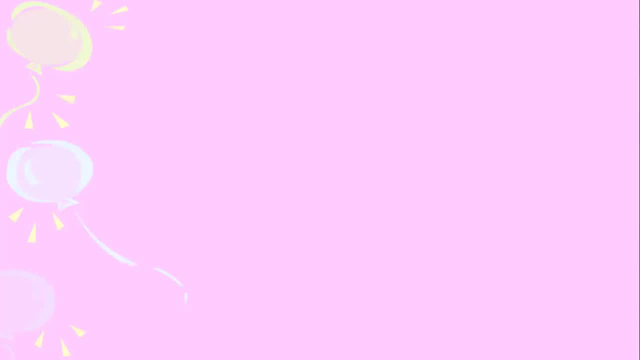 sequence of eight bits represent S And the last series of eight bits represent EEE. A WAND length is therefore the measure of the number of bits in each WAND. For example, the WAND length for the WAND base is the meter for each No and atom. What if I go back to right side? 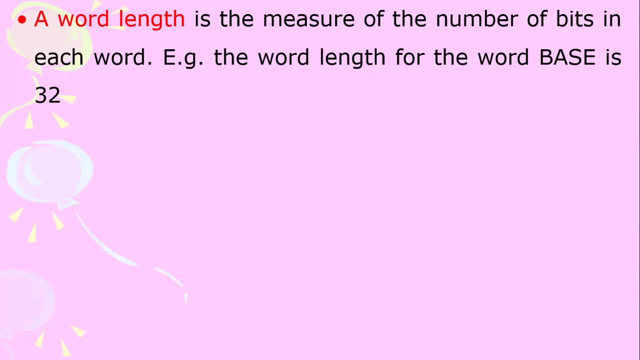 That is, in the center绝. And then the limited space that we have already looked at is useful for us to count and mountains. Therefore, when we defer to want lane, we are simply referring to the total number of B Blockchain, its total number of bits that represent the full WAND. 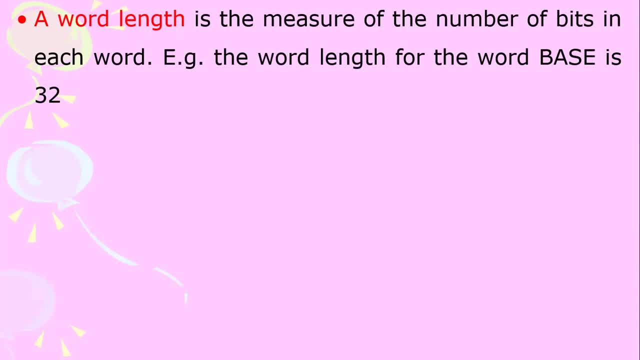 of bits that represent the full WAND of the data, of the data, of the data, computing, even a space. A space is a character and therefore it also consists of one byte, which is equal to eight bits. Complex data is represented using strings or streams of. 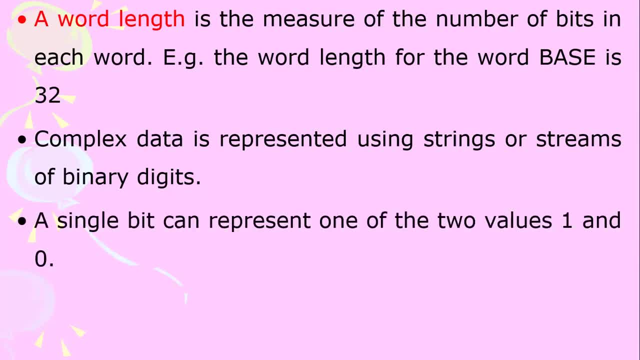 binary digits. A single bit can represent one of the two values, one and zero. A group of two bits can be used to represent one of four, which is of course two, two representing the number two, Then race two values. that means a series of four combinations of zeros and one or a. 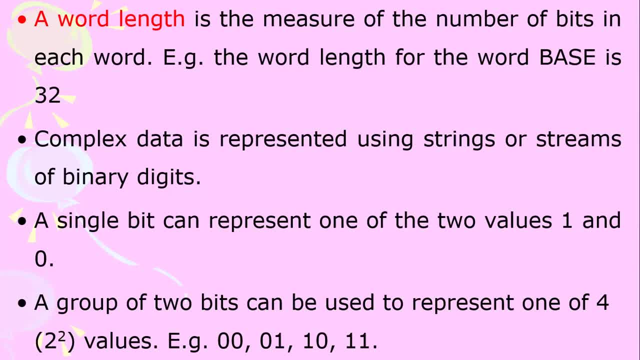 four pairs off two bits each. that is 0, 0, 1, one zero. I repeat, a group of two bits can be used to represent one of four, that is two, two values. In other words, a group of two bits that is zero and one combination. 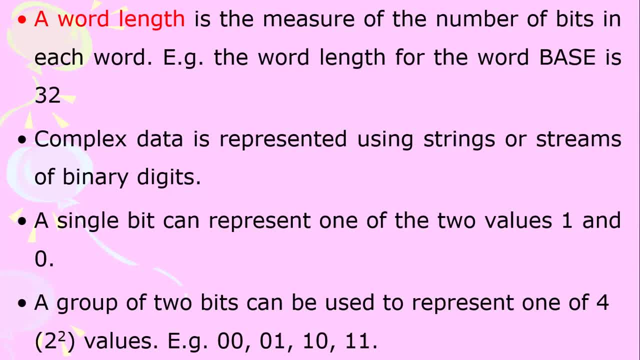 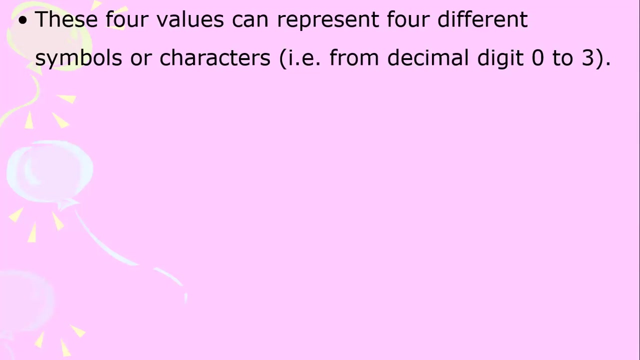 can form four arrangements of zeroes and ones, And those four combinations of two bits is 00, 01, 10, 11.. 00, 01, 10, 11.. values can represent four different symbols or characters, that is, from decimal digit zero to three. 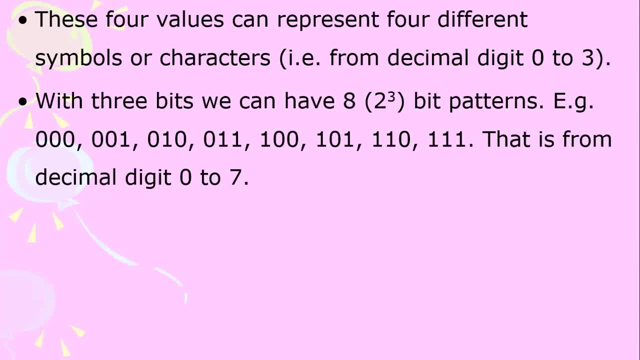 With three bits we can have eight. that is two for the two states raised to power, three, For example. all that is zero, zero, zero, then zero, zero, one, zero, one, zero, zero, one, one, one, zero, zero, one, zero one. 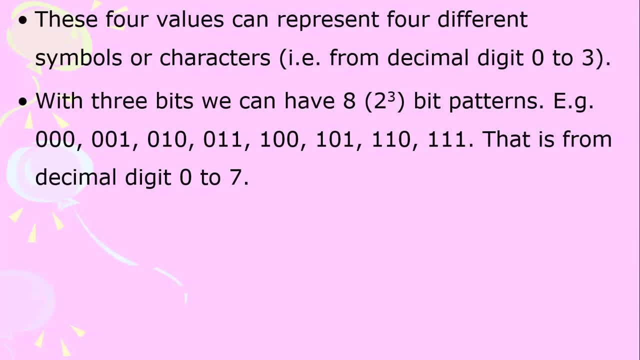 One, one, one, one, one, zero. I repeat, the arrangement of the three bits can be in the following order: Zero, zero, zero. In fact, that is decimal digit zero, Then zero, zero, one for decimal digit one. 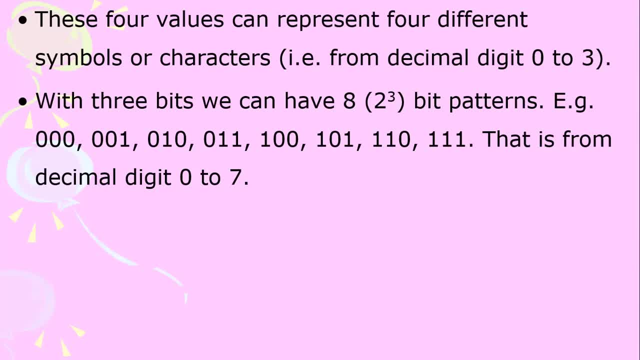 Zero one zero For decimal digit two: Zero one one For decimal digit three: One zero zero For decimal digit four: One zero one For decimal digit five: One one zero For decimal digit six. 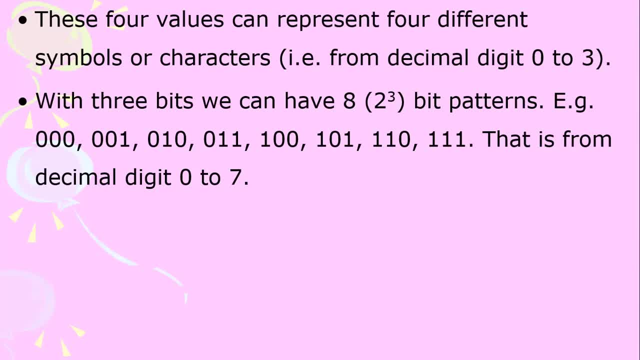 One one: one For decimal digit seven. We are going to discuss in depth on how we arrive to this series of bits, when we are going to be looking at the number conversions And attention being on decimal to binary number conversions. Therefore, look for my part two and part three of presentations in this series or in this topic, and data representation from MLSwap ICT YouTube channel. 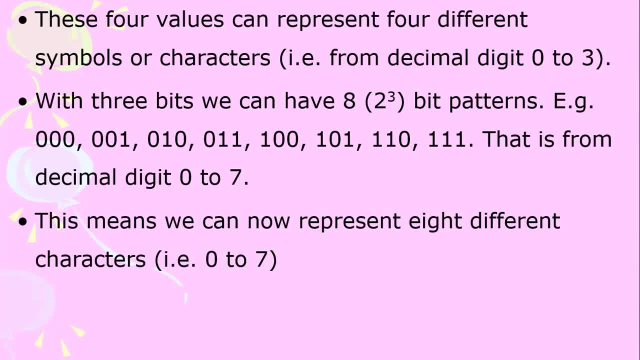 This means we can now represent eight different characters, That is zero or character zero two. character seven using three bits, combinations or patterns. With the four bits we can represent sixteen, That is two to power, four characters two. 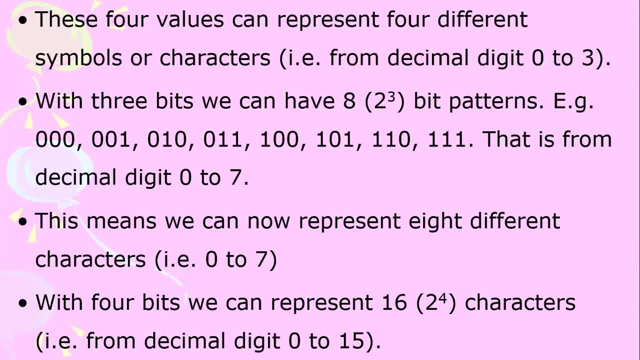 For the two binary states, zero or one Four for the number of bits. So with the four bits we can represent sixteen. That is two to power, four characters ranging from decimal digit zero to fifteen. Remember, zero is also counted because it is a number in computing. 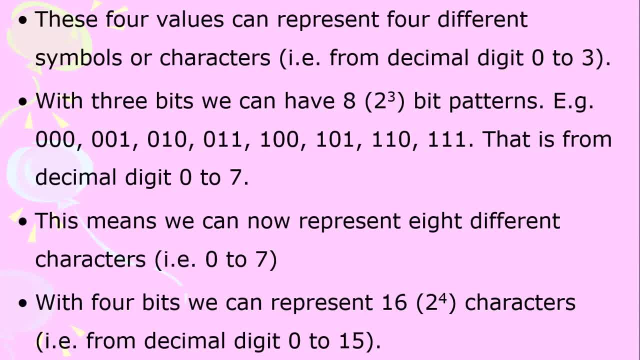 It is a valid number, This is a significant number And therefore, from decimal digit zero to fifteen, We have sixteen characters And those can be represented with the four bit patterns or four bits. In other words, I repeat, With sixteen characters, or to arrive at sixteen characters, we can have four bit patterns. 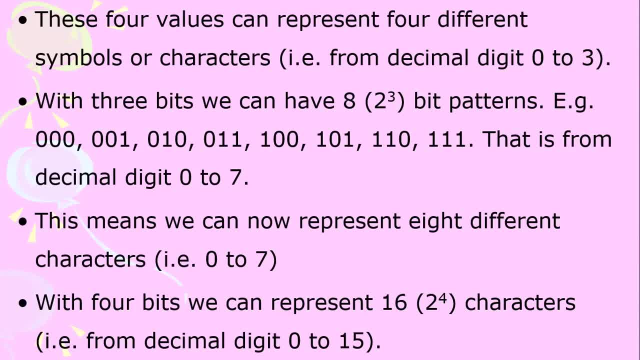 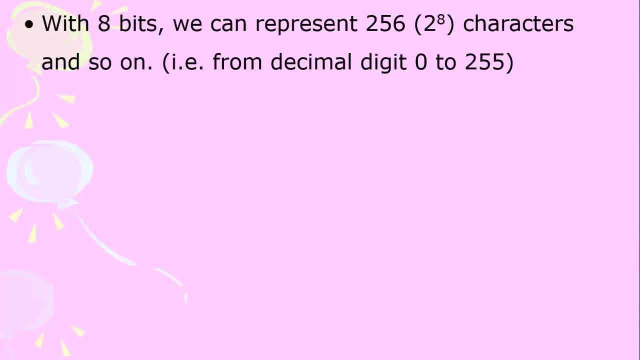 Composed of zeros and ones, While with eight bits we can represent two. fifty-six, That is, two raised to eight characters, and so on. That is from decimal digit zero to two fifty-five, My dear students and the rest of the learners, 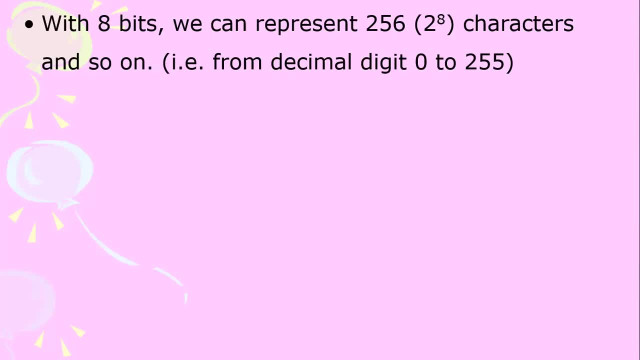 In fact, when I talk about eight bits to forming two fifty-six characters, I mean eight bits. the first bit pattern would be a series of zero, eight bits Zero. In other words, simply put, Eight bits Forming two hundred fifty-six characters. 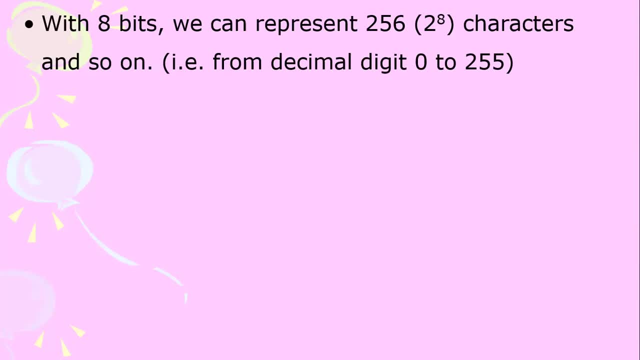 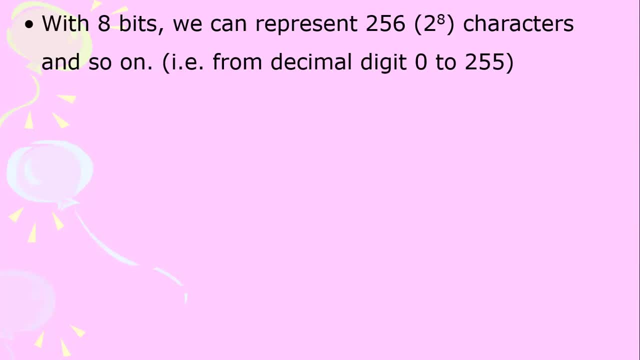 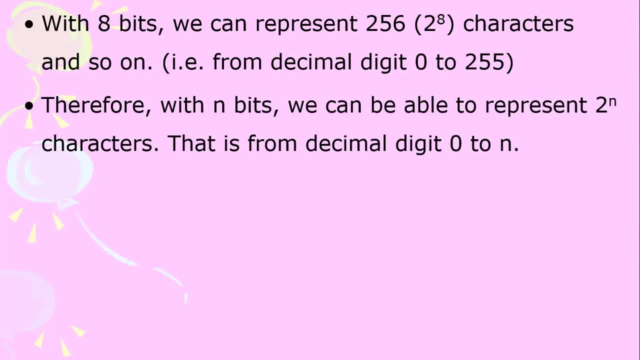 Therefore, with any bits We can be able to represent Two raised to power n characters, Two for the two states On and off, While n is the number of bits. So You just need to replace n in your computation To be able to know the number of characters. 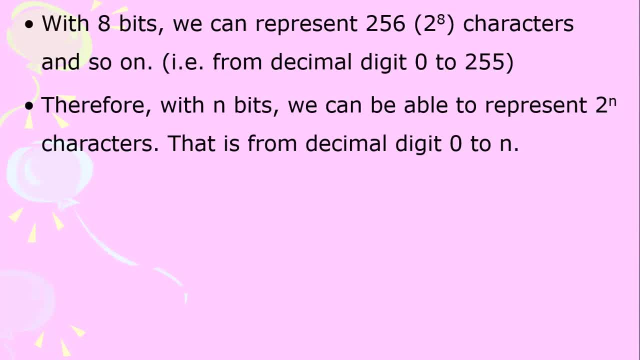 That can be Formed Using a certain number Of Binary digits, If The number Of bits Is, for example, 10.. That means A series of Beat patterns Spanning from Ten zeros To 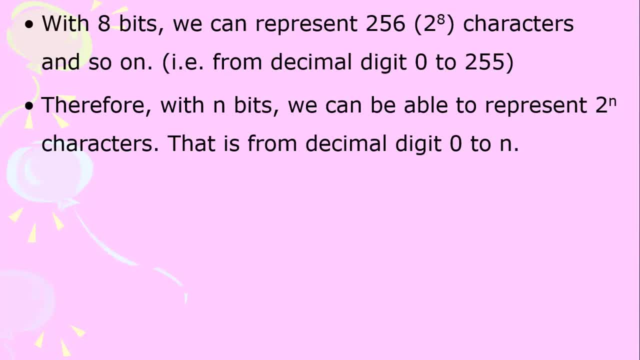 Ten ones, Then For you to be able to know The total number of characters That those ten bits Will be able to represent, You just need to Pick Two And raise it To The number of bits. For example, 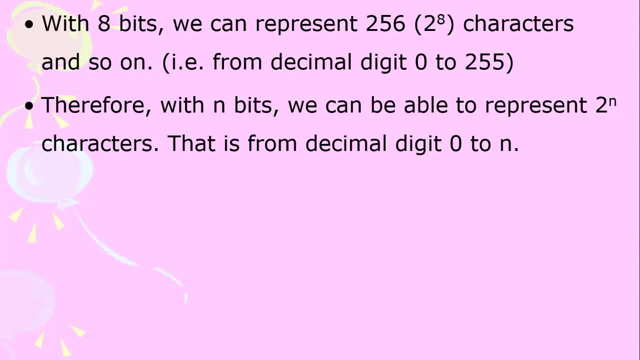 If the number of bits are ten, Then you say Two Raised To Ten, That is Two To power ten, And you get The respective Number Of Characters And therefore With N bits We can be able to represent. 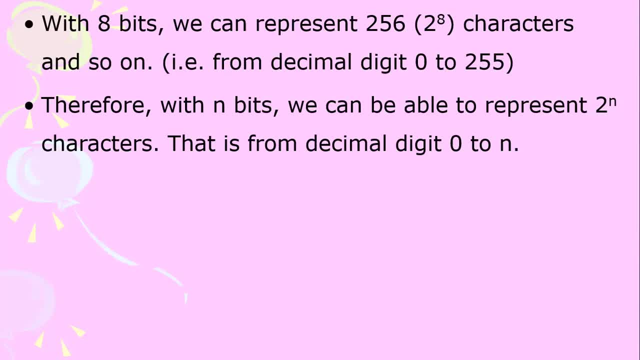 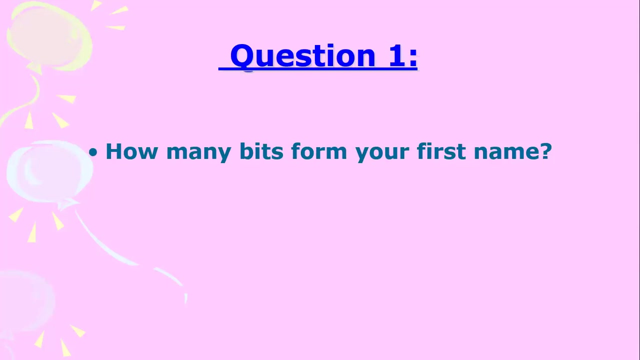 Two Raised To Ten Or Two Raised To N. Characters, That is, From decimal digits To N Characters, From decimal digit zero To N. Let's Challenge Our brains a little. 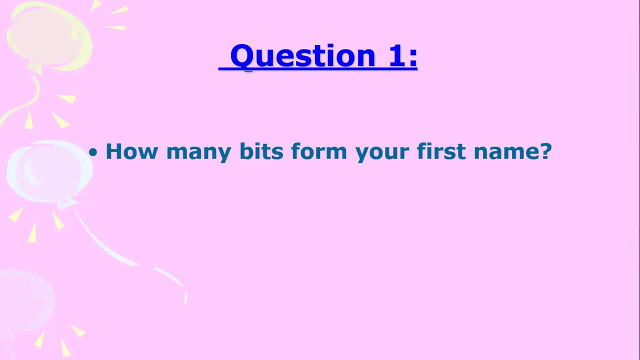 Let's see Whether you have understood What we have already learned. How many bits Form Your first name? How many Binary digits Form Your first name? You have one minute To Count them. One Minute. 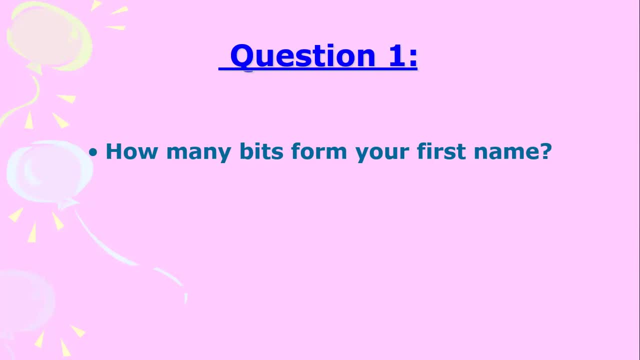 To Count Them One. Let's now see if you've been able to compute the number of bits for your first name. I'll use my example. This is how you proceed. First of all, write down your first name. My first name is Meh-meh. 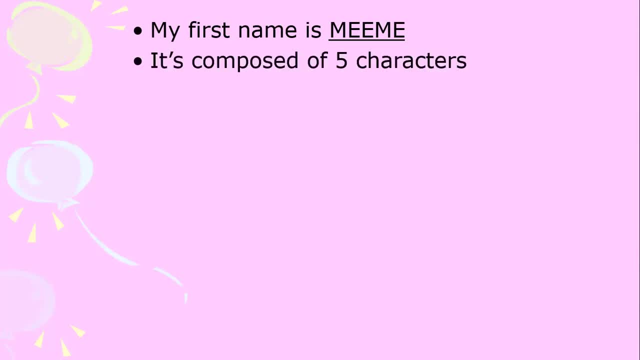 Then the next step is count the number of characters that form your first name. My first name is composed of five characters. That is, M E E M E, Or M E E M, Or you can simply say M double E, M E. 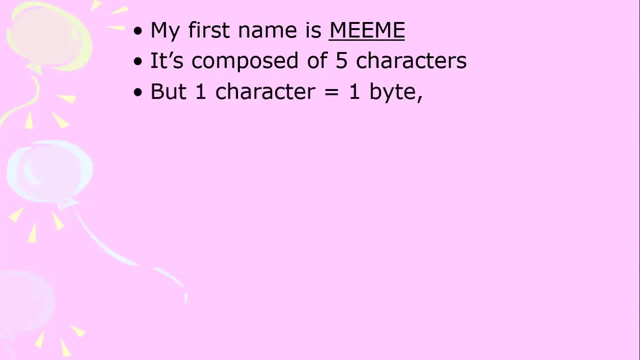 Those are five characters. Then count the number of bytes that form your name. Remember, one character is equal to one byte, And therefore five characters, Which, for my name, will be equal to how many bytes. What you do? you multiply the number of characters, with one byte divided by one character. 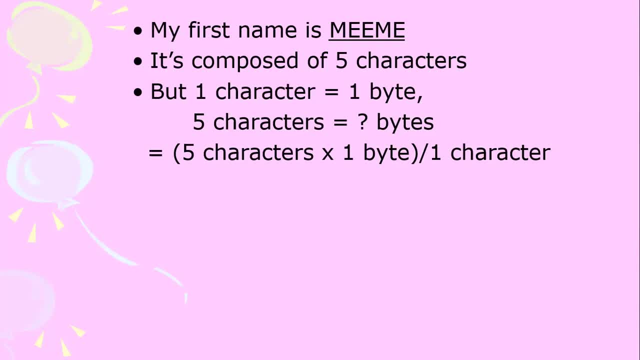 In this case, for my case, it will be five characters times one byte, divided by one character. The character and the character will cancel each other And therefore we shall be left with five bytes. However, we have already said that one byte is equal to eight bits. 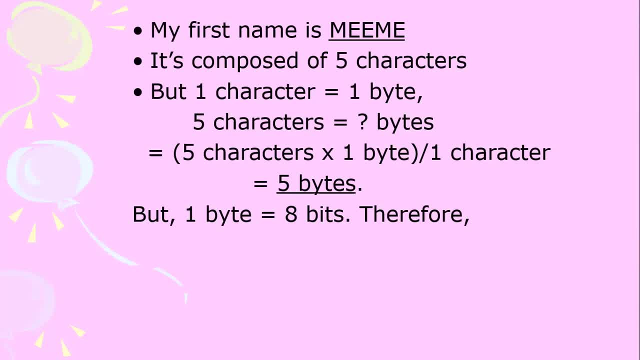 So how do we compute the number of bytes? How many bits will form or will be formed from our five bytes? Therefore, five bytes will be equal to how many bits It is five bytes times eight bits. divided by one byte, The term byte and byte will cancel each other and therefore we shall be left with 40 bits. 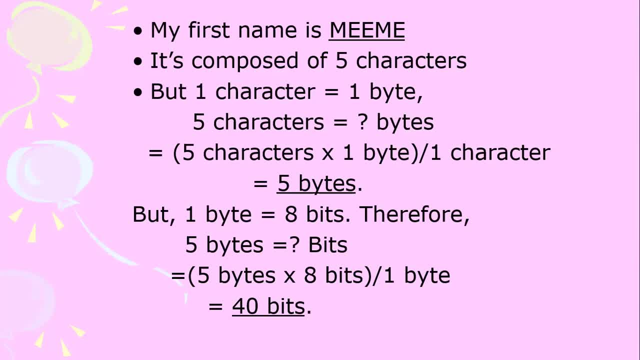 Therefore, my first name, M E M, is composed of 40 bits. Therefore, my one length, one length for my first name long, one length for my name long, and therefore a basically two bits remarak-. 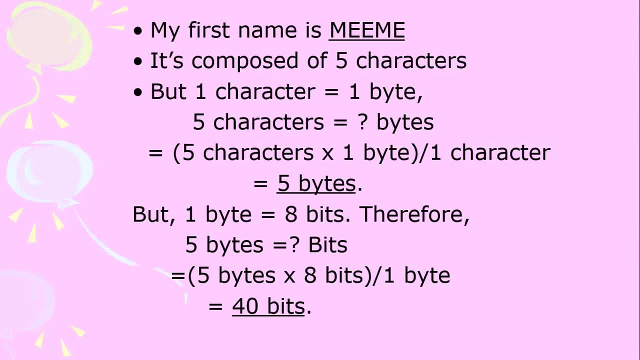 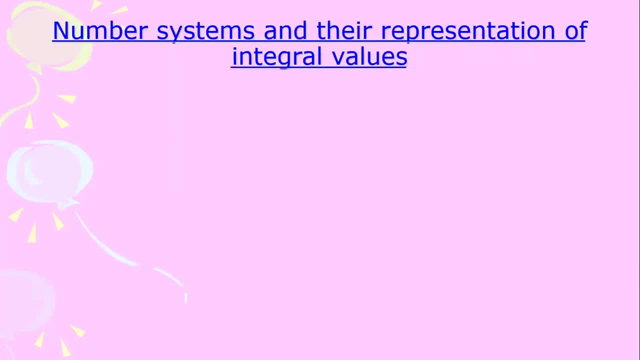 First name, meh-meh, is equals to 40 bits. Let's now focus on number systems and their representation of integral values. Number systems and their representation of integral values. Complex types of data, such as sound and pictures, take a lot of memory and processor time when coded in binary form. 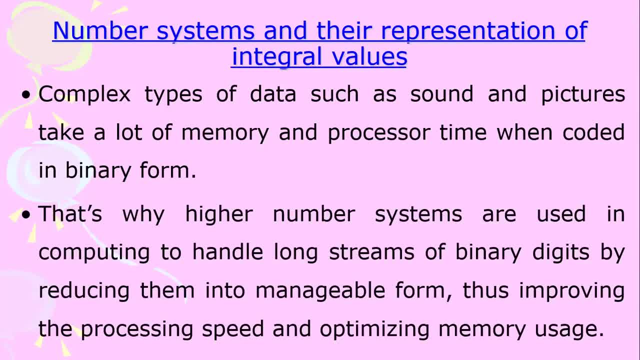 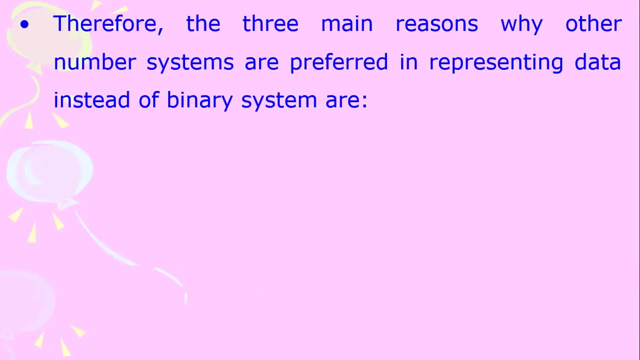 That's why higher number systems are used in computing to handle long streams of binary digits by reducing them into manageable form, thus improving the processing speed and optimizing memory usage. Therefore, the three main reasons why other number systems are preferred in representing data instead of binary system are: 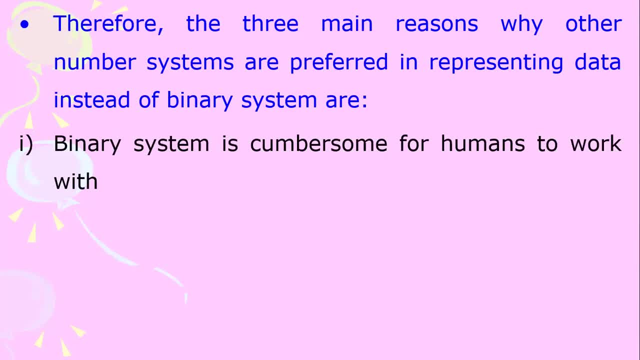 Number one binary system is cumbersome for humans to work with and you have seen this from our tabulation For just the number of bits that form your first name and therefore you can imagine if you are dealing with volumes of pages of once. that would be very cumbersome. 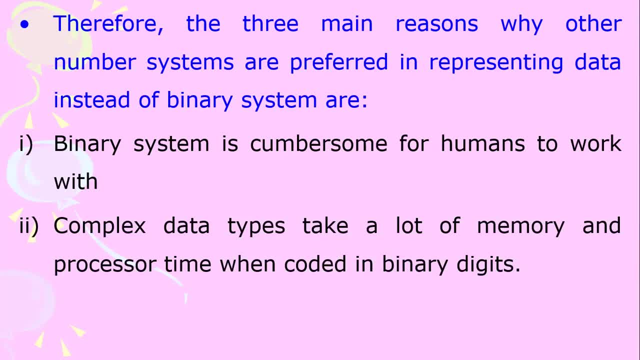 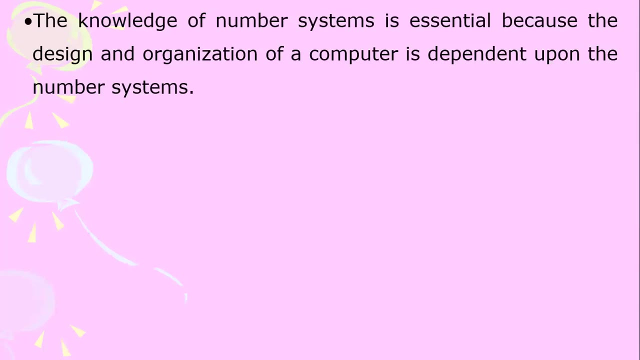 Number two: complex data types take a lot of memory and processor time when coded in binary digits. Number three: higher number systems reduce streams of binary into manageable form. So the knowledge of number systems is essential because the design and organization of a computer is dependent upon the number systems. 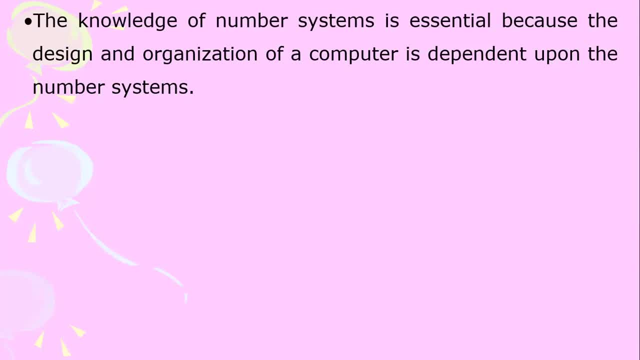 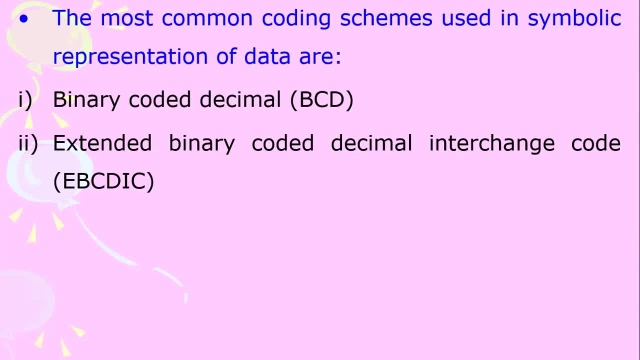 Therefore, the number systems is a very important topic or area or field in computing. Therefore, the number systems is a very important topic or area or field in computing. Number three: American Standard Code for Information Interchange. American Standard Code for Information Interchange as key. 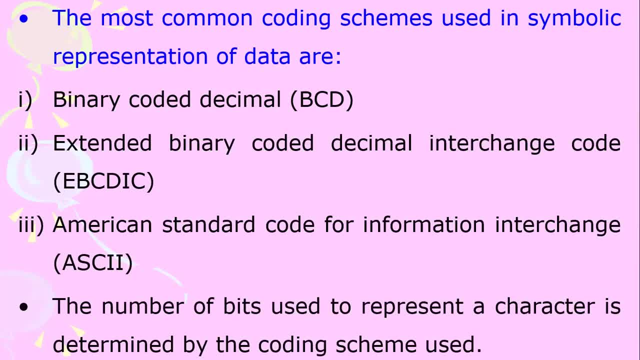 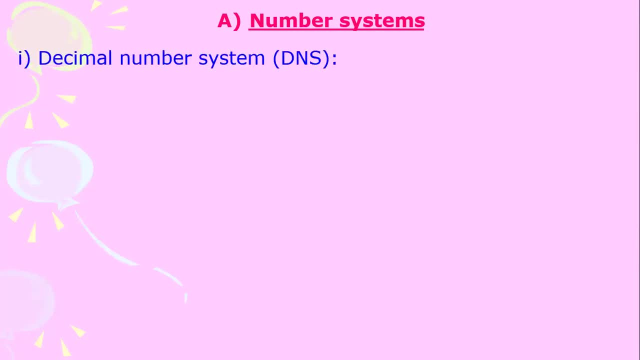 The number of bits used to represent a character is therefore determined by the coding scheme used. Let's look at number systems. We commence with decimal number system, DNS. This is a system of representing numbers with the use of ten digits, symbols zero to nine. 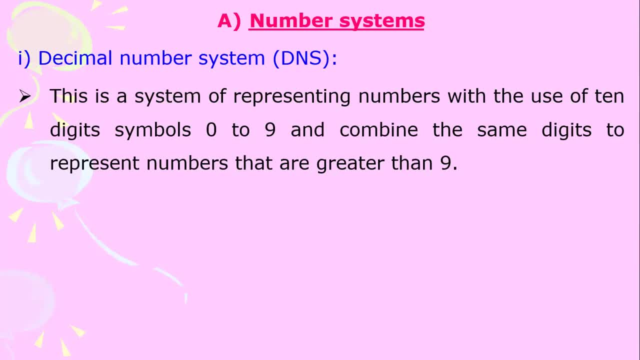 and combine the same digits to represent numbers that are greater than or equal to zero. So it's called base-ten number system or binary number system, because it is composed of ten digits spanning from digit zero to nine, which may be represented as x to base-ten. 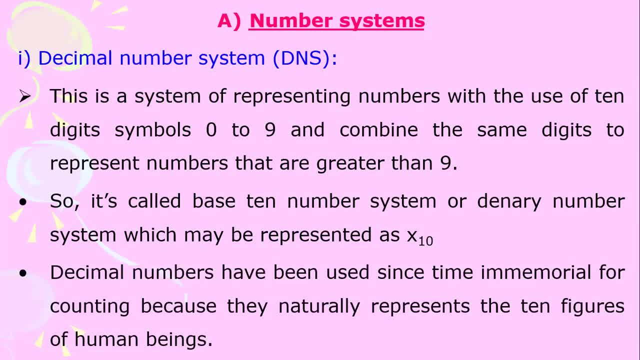 Okay. Decimal numbers have been used since time immemorial for counting, because they naturally represent the ten figures of human beings. Talk of ten fingers for the hand. Talk of ten toes for the feet. Talk of ten commandments. It is C. 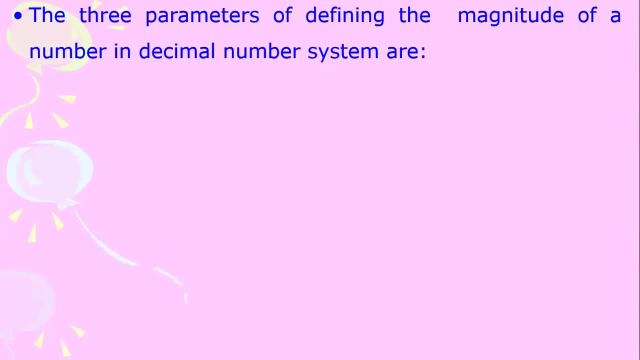 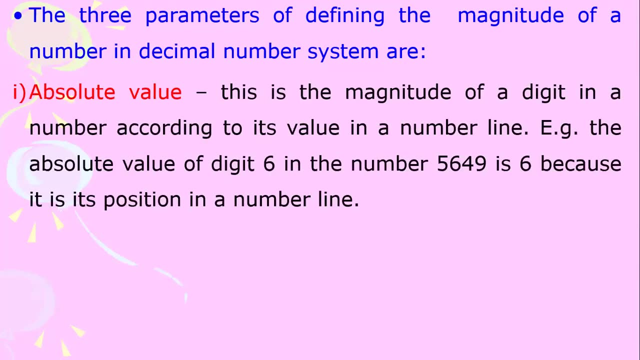 Okay, The three parameters of defining the magnitude of a number in decimal number system are therefore number one: absolute value. This is the magnitude of a digit in a number according to its value in a number line. For example, the absolute value of digit six in the number 5649 is the absolute value of. 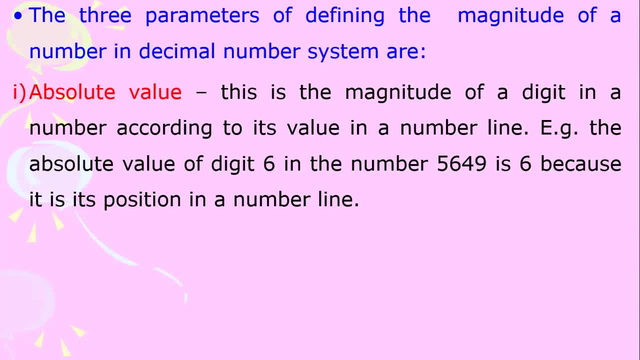 a number. Okay, The absolute value of a digit in a number line is six because it is its possession in a number line. So if you have a number line from zero to nine, then six will be the possession of digit six in the number line. 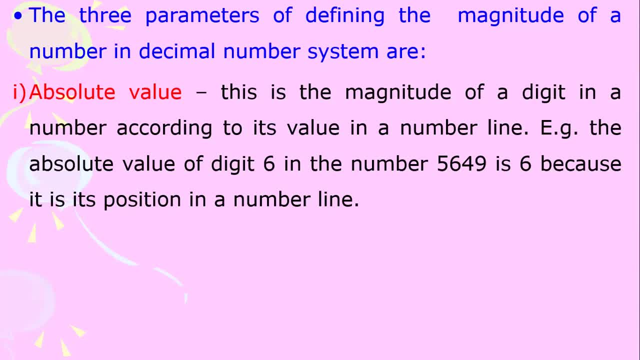 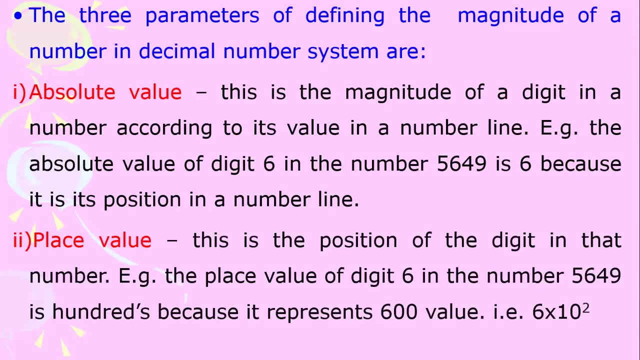 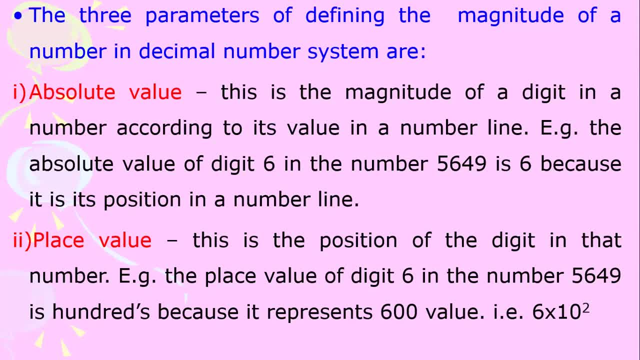 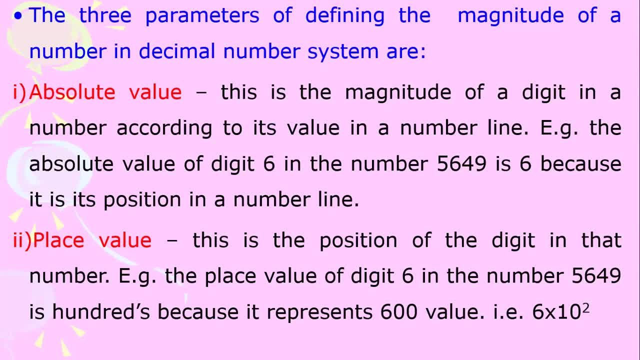 Why The position of the digit in that number, 5649, or that position of six, represents 600, that's why, if we were to read 5649 fully, it will be 5,649.. So six represents the hundreds possession. 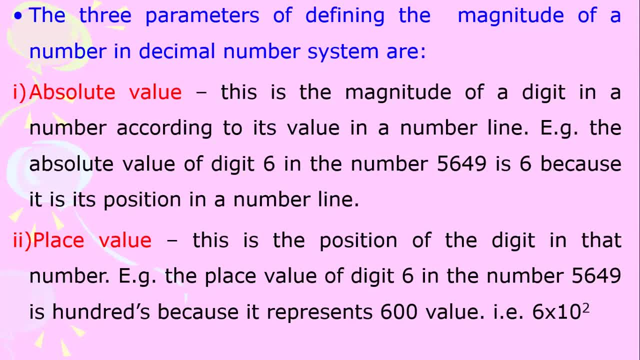 Why 5,649.. Like I said before, it means that the digit is not equal to extra or greater than its are six. So six a hundred, That is six times ten raised to power two. Ten raised to power two is a hundred. So both climb by six. Remember five in terms of position represents thousands. 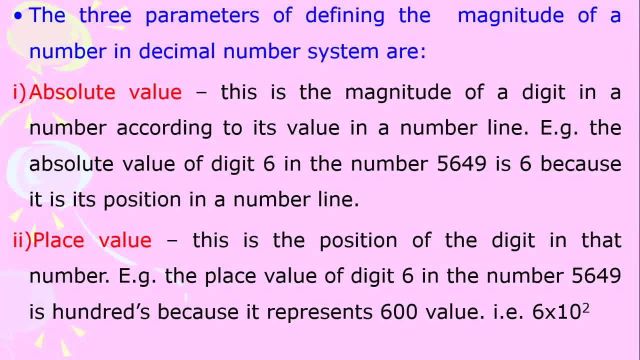 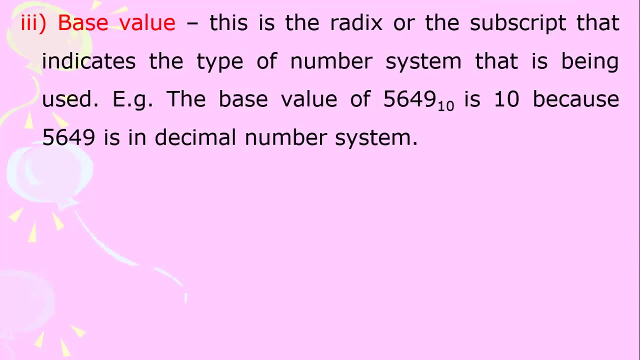 Six is a hundreds, Four is tens, While nine is ones. That's how we look. or we get or we arrive at the positional values of digits in a number. Then number three is base value. This is the radix or the subscript that indicates the type of number system that is being used. So in our case we have five. 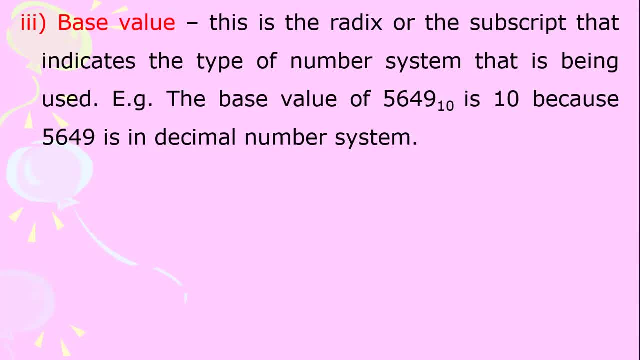 hundred six hundred forty-nine to base ten. In other words, our number is fifty-six forty-nine to base ten, And therefore ten is the subscript, And so our base value is ten. Why? Because fifty-six forty-nine is in decimal number system. 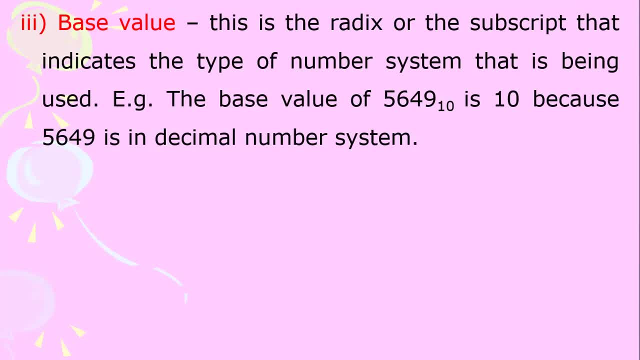 As I have said, base- the base of the number- indicates the number system that that number is in. For example, fifty-six, forty-nine two Base 10 simply means that that's a decimal number system, because the numbers span from 0 to 9,. 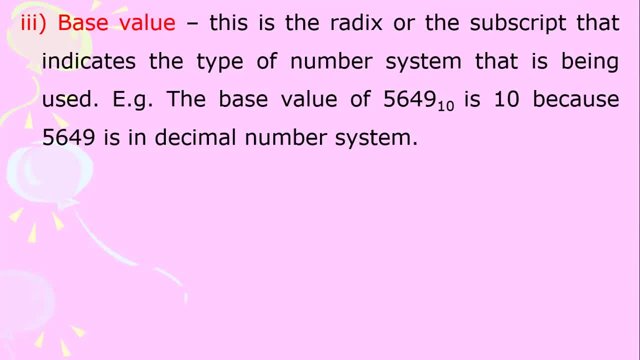 and those are 10 digits, So base 10.. 8 indicates the base value is 8, meaning it is an octal, And that also means that the octal represents a series of 8 digits, 0 to 7.. 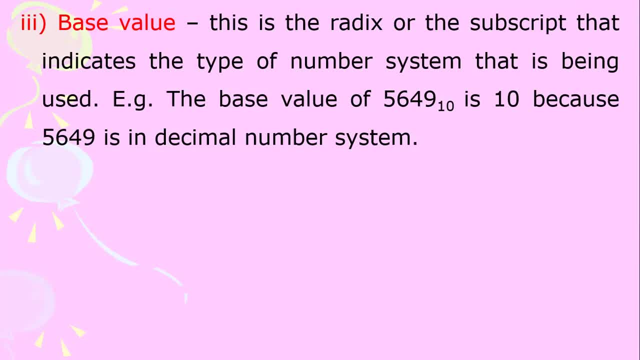 When we talk of 2 for binary, those are 2 numbers, So it's a series of 2 numbers, 0 to 1.. If we talk of hexadecimal, then that would be base 16.. 16, meaning that the numbers in that system span. 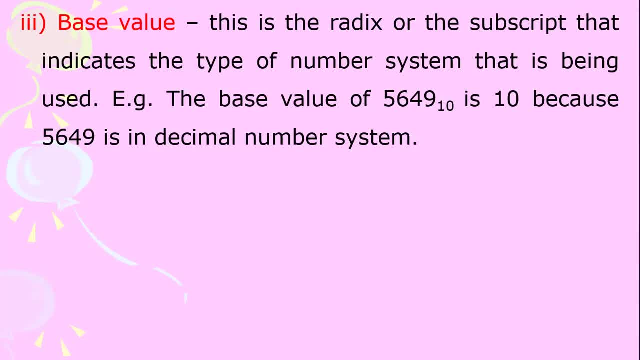 from digit 0 to 15.. But of course we are going to see how we represent numbers beyond digit 9 in hexadecimal system. The most important thing for you to note, my dear students and the rest of the learners, is how we understand. 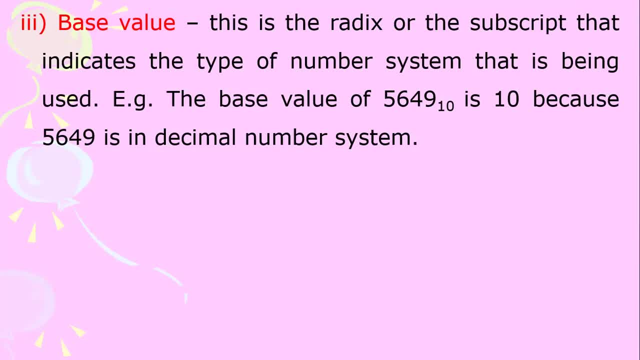 When we arrive at the base value, we always look at the subscript or the randex for the number given. If it is 10, like it is our case for 5649,, then we can be able to tell that that is a decimal number system. 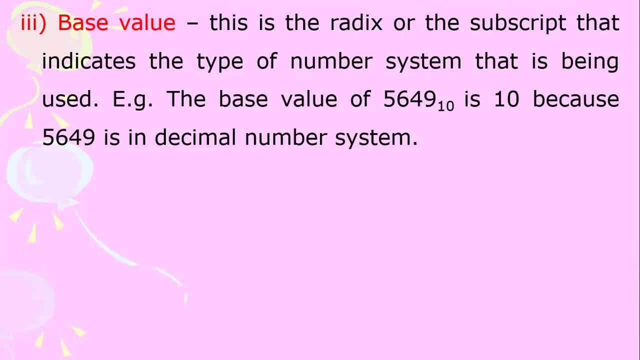 If the randex or subscript is 16,, that would be hexadecimal number system. If the randex is 8,, that is octal. If the randex is 2,, that is binary. The weight of each position is multiplied by the corresponding digit. 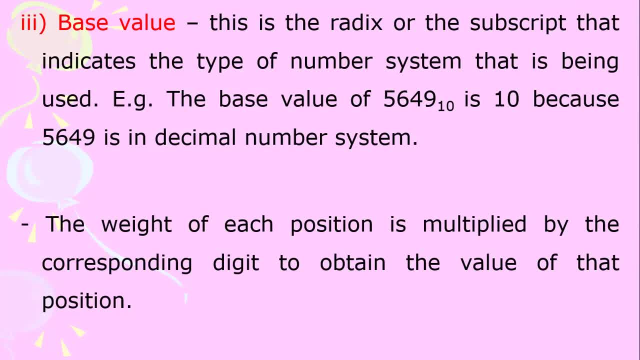 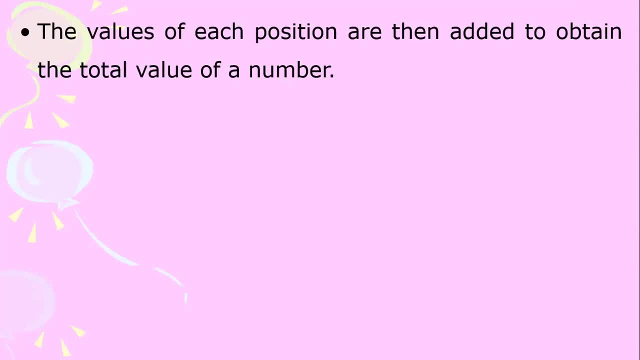 to obtain the value of that position. The values of each position are then added to obtain the total value of a number, For example, to get 5649, that is 5,649.. The values of each digit position is calculated and added as follows. 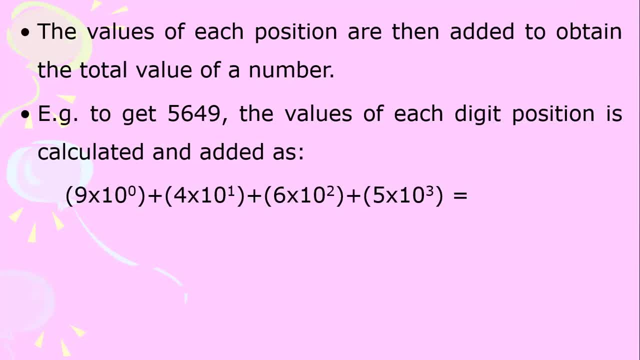 Remember we are dealing with decimal number system: dec for 10.. So how do we compute? We begin with the list of the ones In our computation, we begin dealing with the ones, That is what is on the digit on your rightmost part. 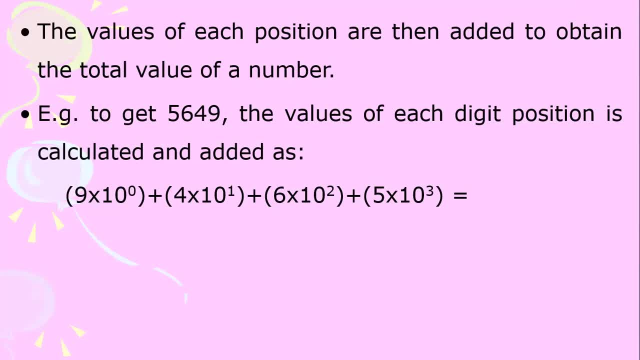 Two ones, the left. So we do the computation, the calculation, in this case, moving from the left to the right, Moving from ones to thousands: 100,000 EPC, That is, from your left-hand side to ones, That is, from your right-hand side to ones, to your left-hand side. 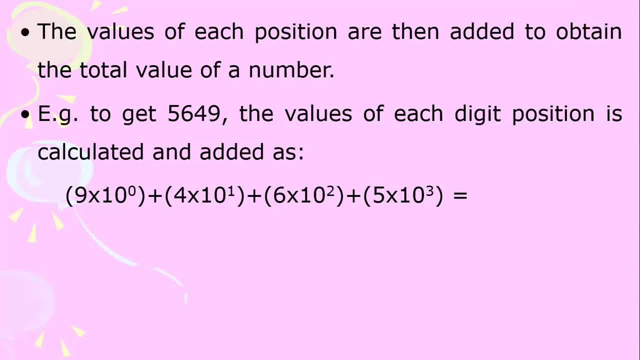 So in this case it is, and because our number 5649 is a decimal, we move as follows: 9 times 10.. That is to power zero Plus. next digit is tens, Or represents place value of tens. So it is 4 times 10 raised to power 1.. 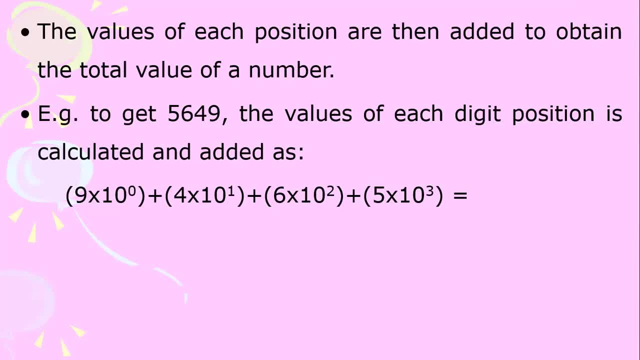 Plus 6 times 10, raised to power. 2. Plus 5 times 10 raised to power. 3. My dear students and the rest of the learners, whenever we are raising numbers, we begin raising with the zero. That is superscript zero. 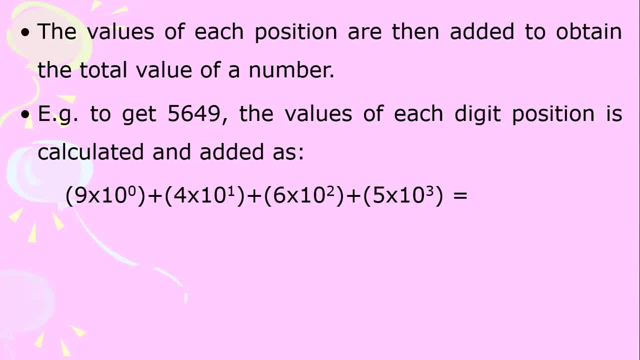 1,, 2,, 3, etc. Based on the length of the number or the number of characters forming our number. So in this case we get 9 times 10 to power. zero is 9 times 1.. So in this case we get 9 times 10 to power. zero is 9 times 1.. 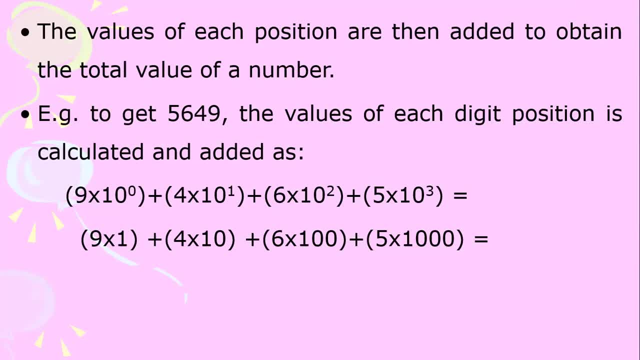 Then we have 4 times 10, because 10 raised to power 1 or n number raised to power 1, is that number. I repeat: any number raised to power zero is 1 or gives 1.. Any number raised to power 1 gives the same number. 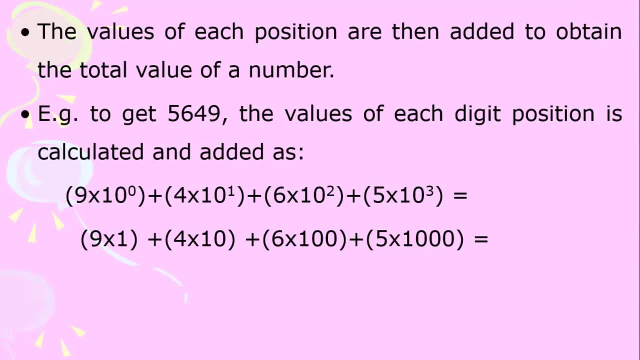 So 4 times 10.. And then 10 raised to power 2 is 100. That is 10 times 10.. 100. So it is 6 times 100.. Plus 5 times 1000.. Because 10 raised to power 3 simply means it is 10 times 10 times 10.. 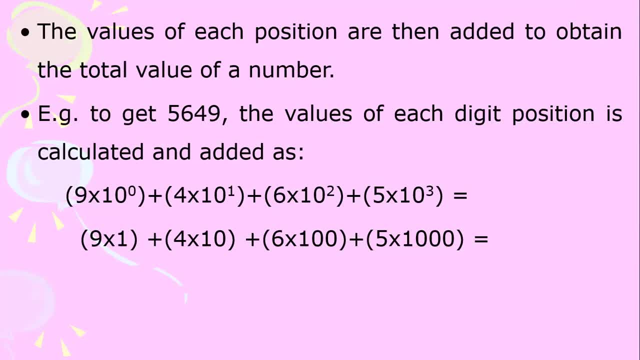 10, multiplying by itself 3 times, Giving 1,000.. So the answer is 9 plus 40 plus 600 plus 5,000, which gives 5,649 to base 10, or an extend Good In any number. 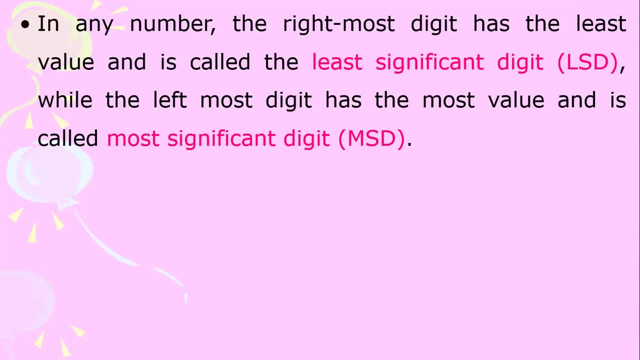 we have a number, We have a number, We have a number. The rightmost digit has the least value and is called the least significant digit, LSD. In our case it is 9.. Or the leftmost digit has the most value. 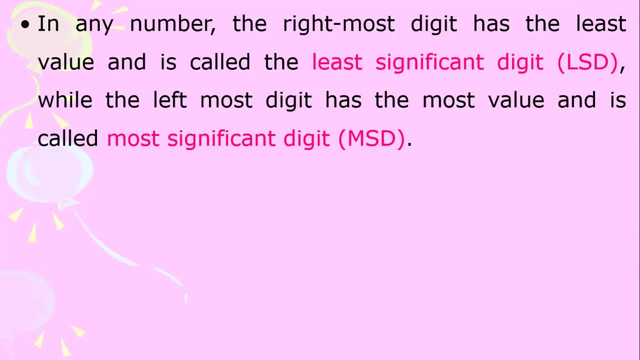 and is called most significant digit, MSD, And in our case it is 5.. So you begin a computation from the least significant digit to the most significant digit. The value of each place increases by a factor of 10 for each consecutive digit. 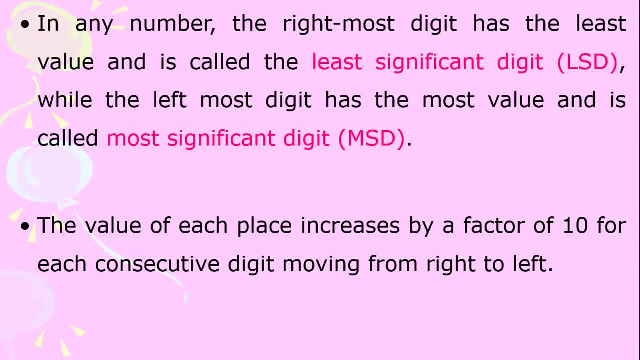 moving from right to left, And my dear students and rest of the learners, Note that we are speaking of factor of 10 because we are dealing with decimals. If it was octal, it would be factor of 8.. If it is binary, it is factor of 2.. 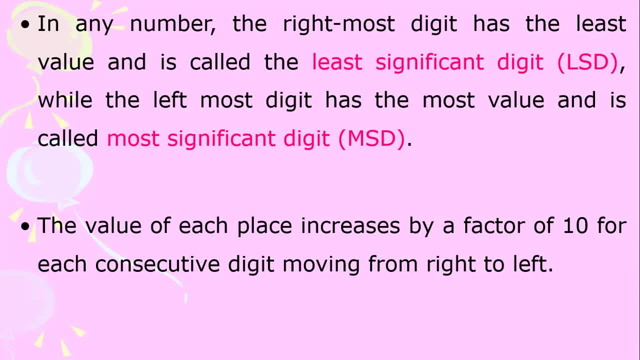 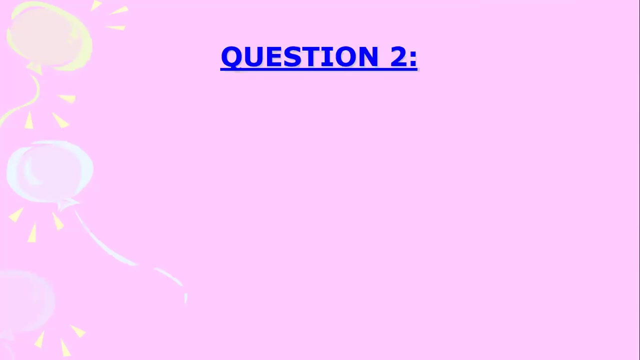 If it is hexadecimal, it is factor of 16.. So the value of each place increases by a factor of 10 for each consecutive digit moving from right to left. My dear students and the rest of the learners, remember we move from right to left of the number. 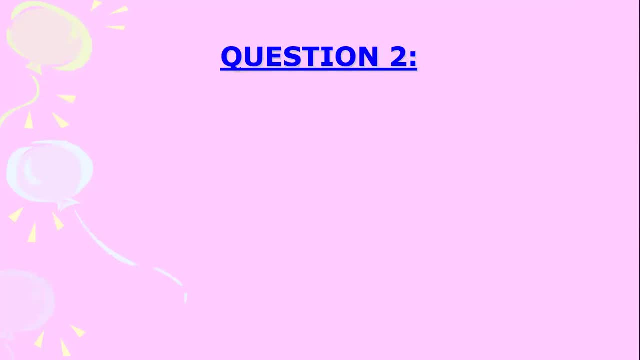 Let's now test ourselves a little to see whether you have understood what we are talking about, What we have done and said. Calculate the total value of 99999, radix 10.. Remember, each step matters, So you have one minute to execute this calculation. 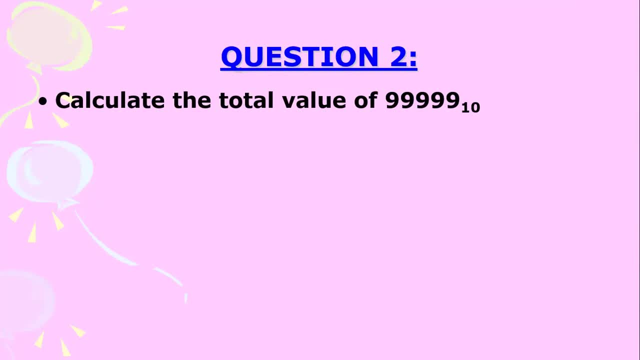 Thank you, All right, So you have a total of 99999, radix 10.. Let's go ahead and try it in classes Number 0.. Let's see what you are supposed to do. The solution is from the least significant digit. the most significant digit we have 9 times 10. 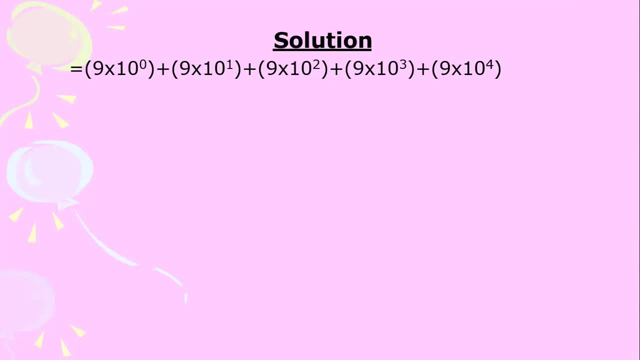 to power 0, plus 9 times 10 to power 1, plus 9 times 10 to power 2, plus 9 times 10 to power 3, and then 9 times 10 to power 4.. 10 raised to 0 is 1, so we have 9 times 1, plus 10 raised to 1 is 10, so we have 9 times 10,. 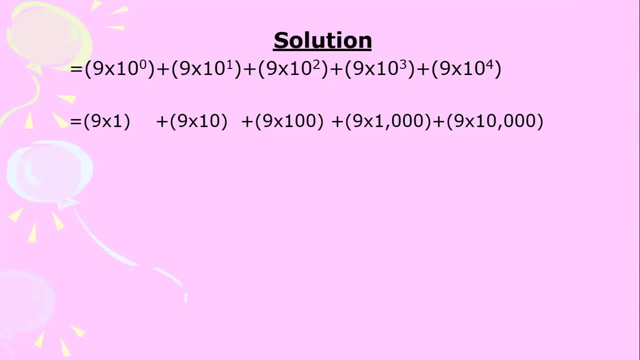 plus 10 raised to 2 is 100, so we have 9 times 10.. 10 raised to power 3 is 1,000, so we have 9 times 1,000.. 10 raised to power 4 is 10,000, so we have 9 times 10,000. 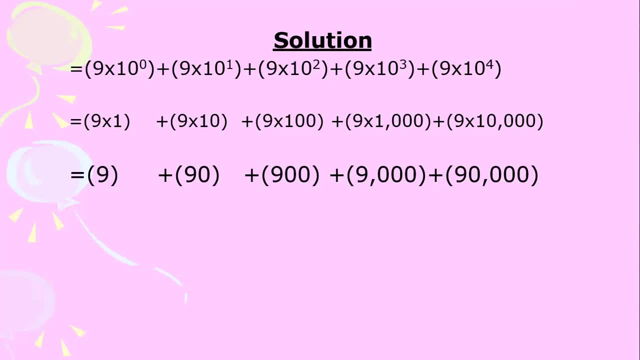 This gives us: 9 times 1 is 9,, plus 9 times 10 is 90,, plus 9 times 100 is 900, plus 4.. 9 times 1,000 is 9,000, plus 9 times 10,000, which is 90,000.. 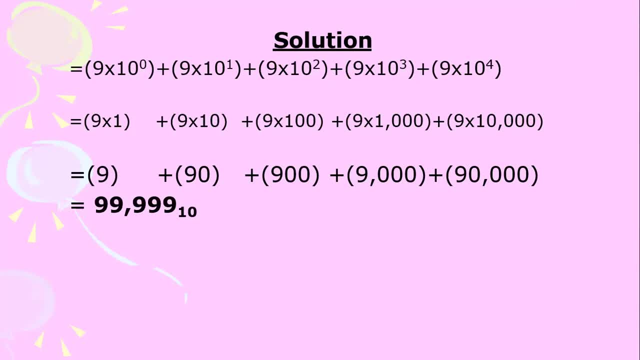 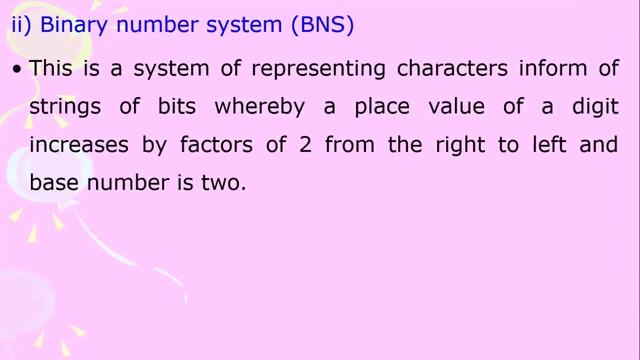 The final answer becomes 99,999 to base 10.. Let's now look at binary number systems B and S. This is a system of representing characters in the form of strings of bits, whereby a place value of a digit increases by factors of 2 from the right to left, and base number 2.. 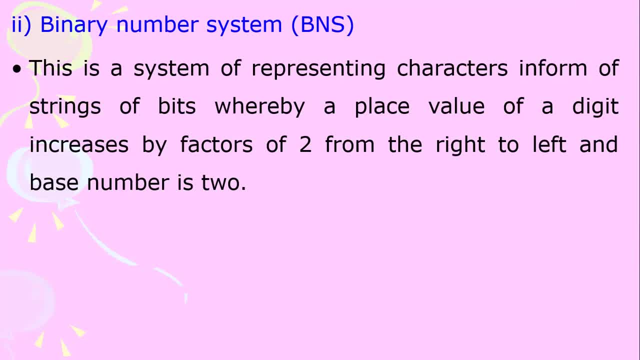 I repeat, this is a system of representing characters in the form of strings of bits whereby a place value of a digit increases by factors of 2 from the right to left and base number 2.. I repeat, this is a system of representing characters in the form of strings of bits whereby a place value of a digit increases by factors of 2 from the right to left and base number 2.. 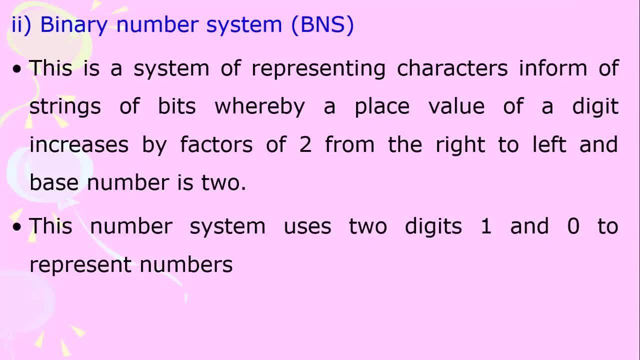 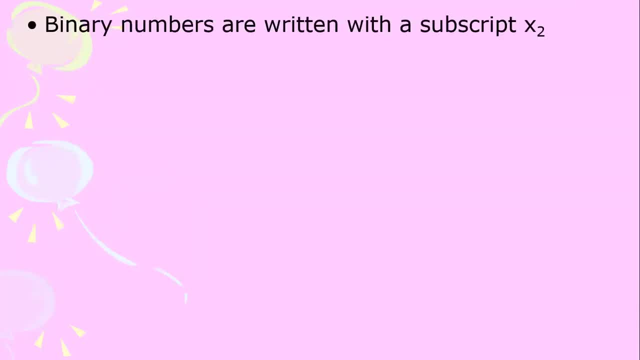 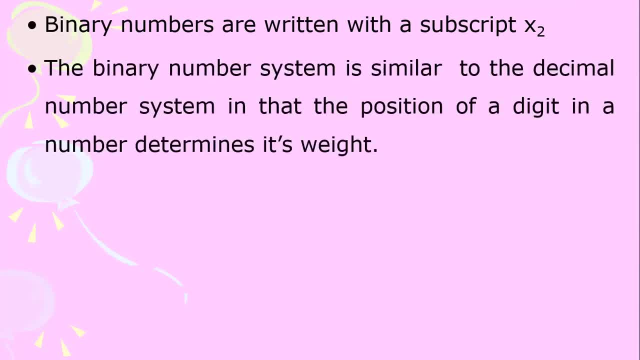 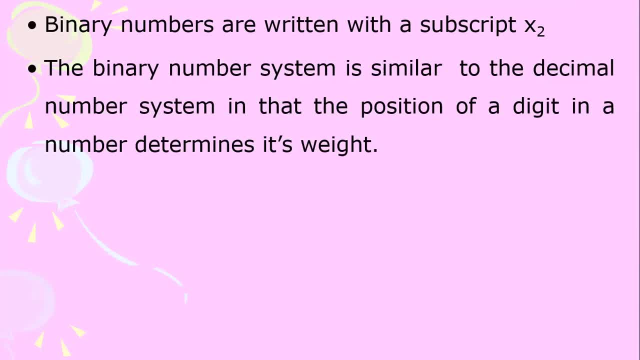 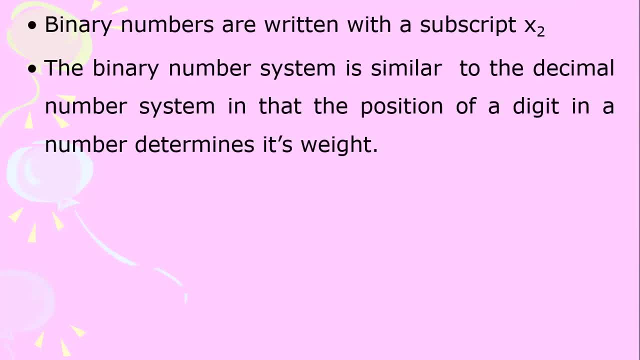 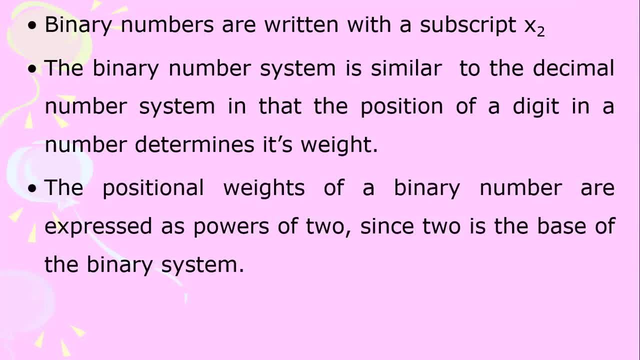 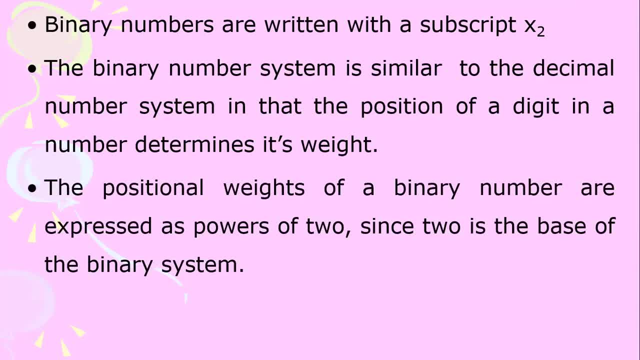 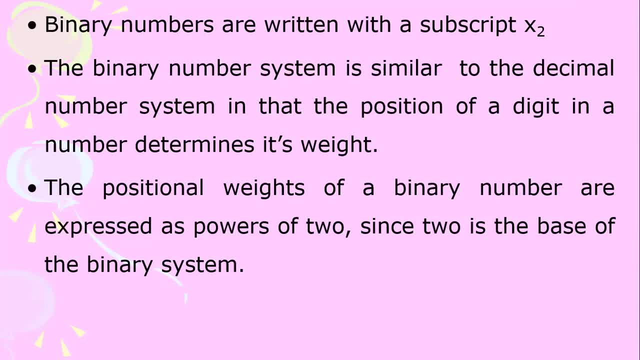 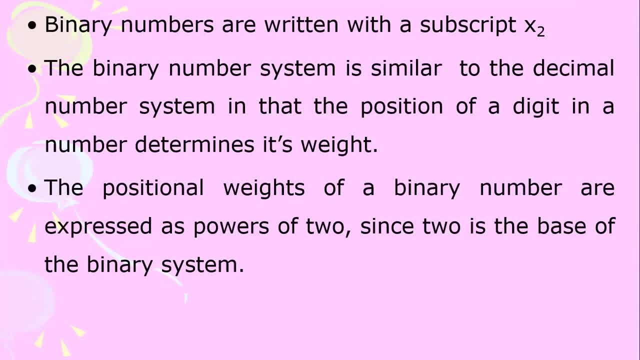 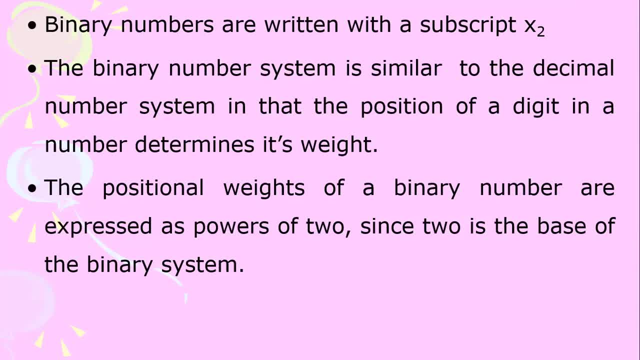 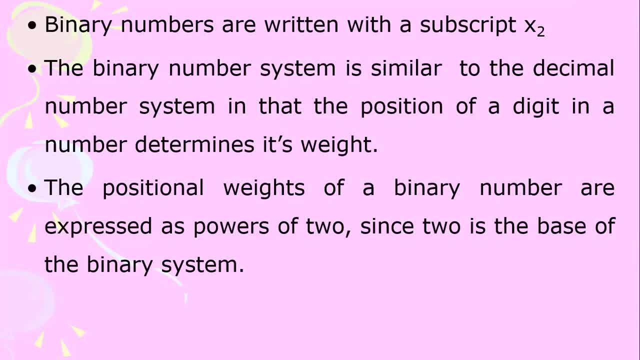 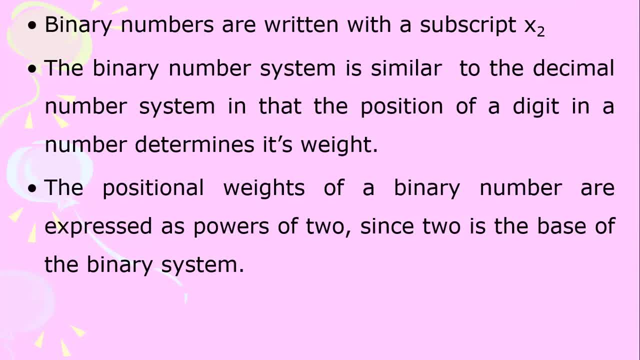 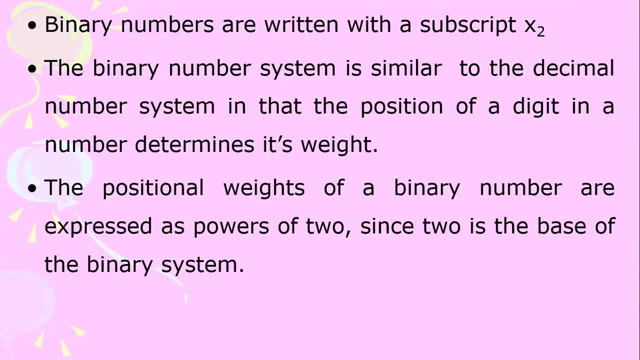 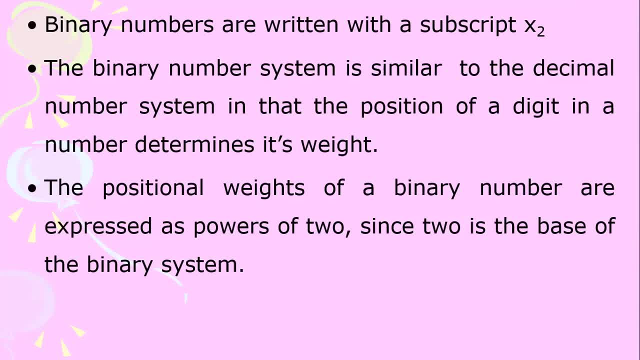 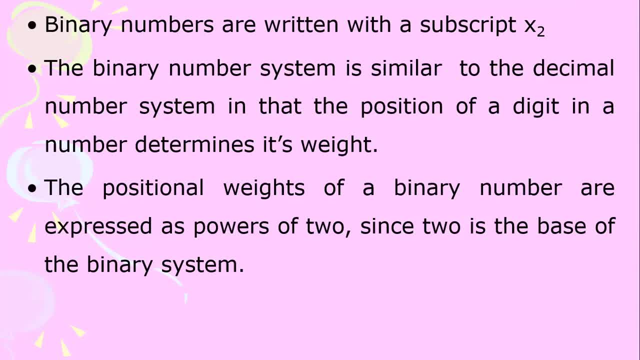 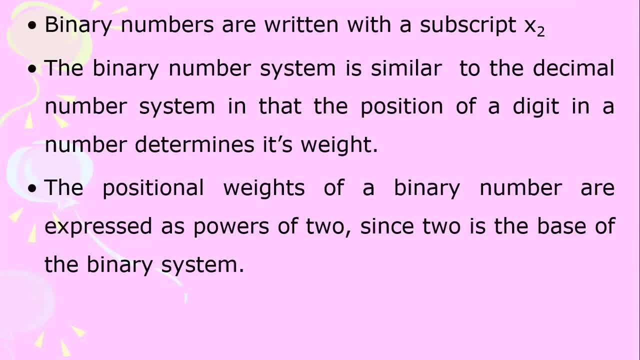 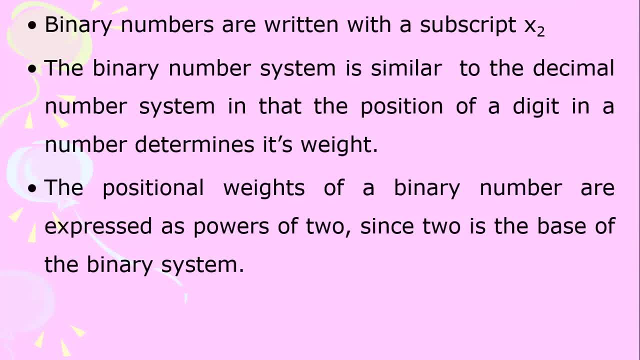 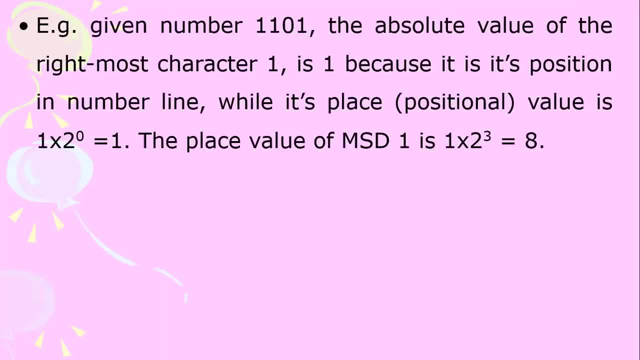 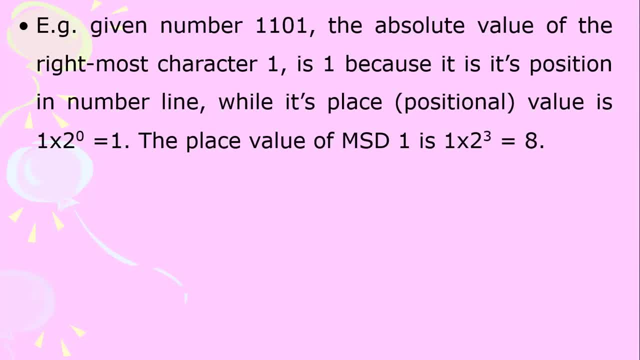 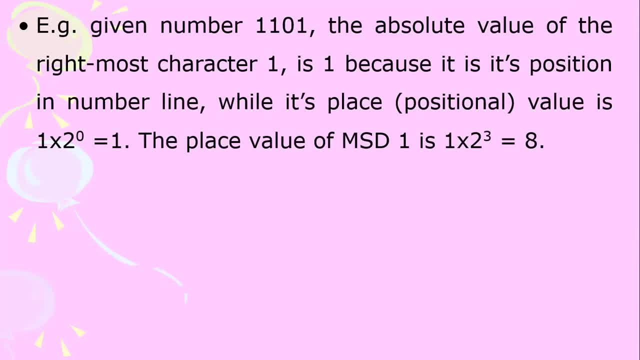 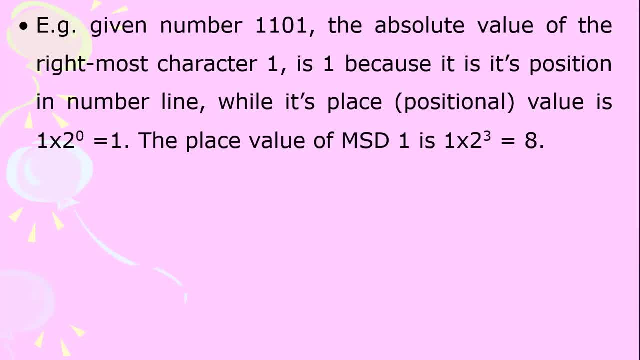 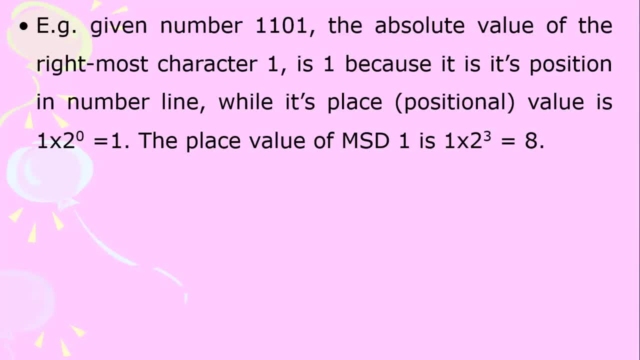 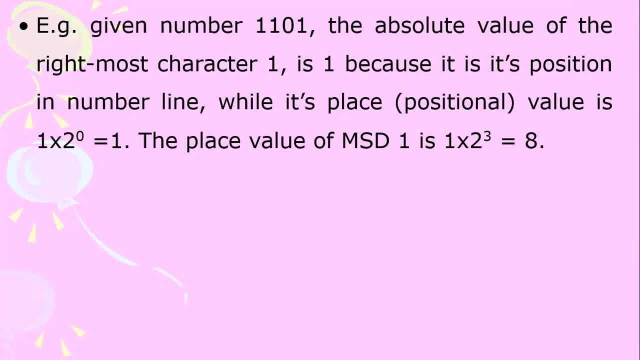 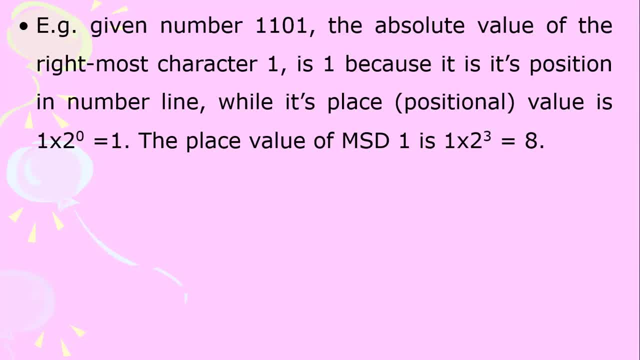 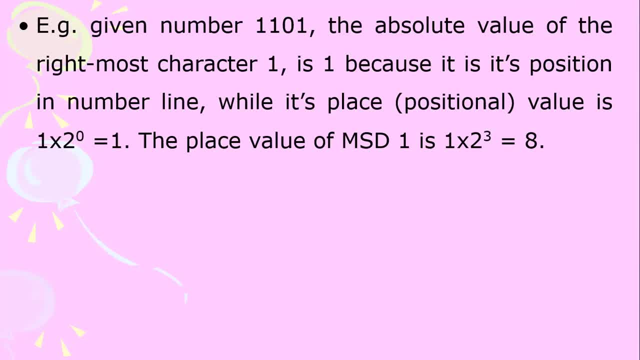 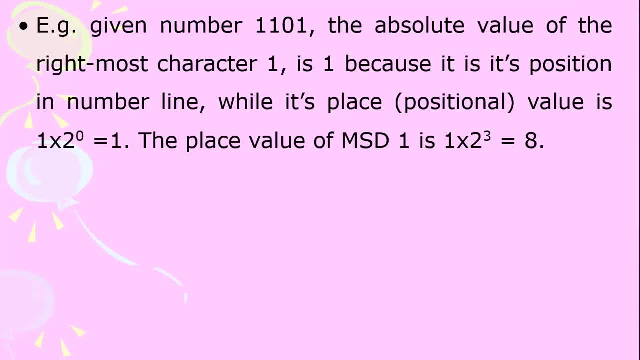 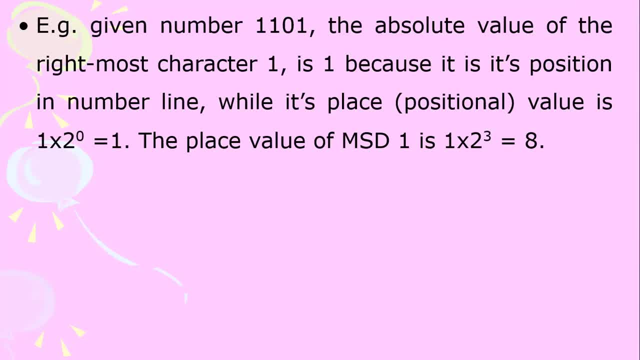 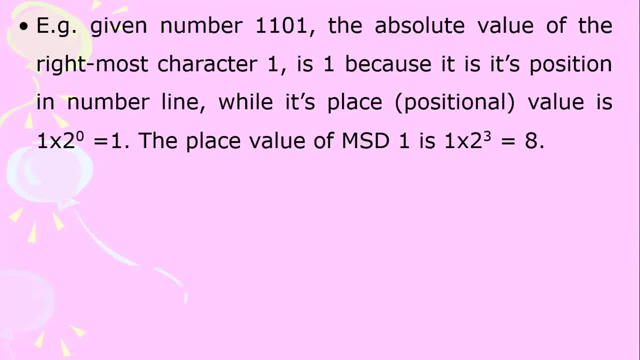 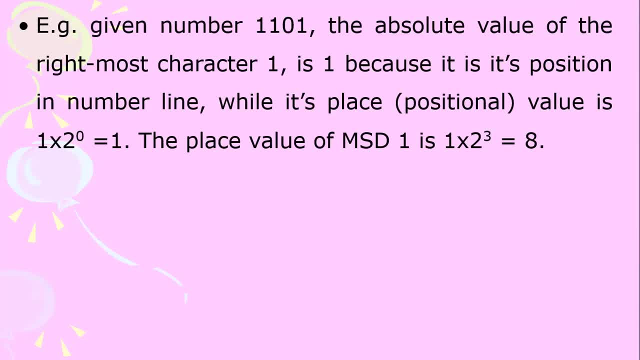 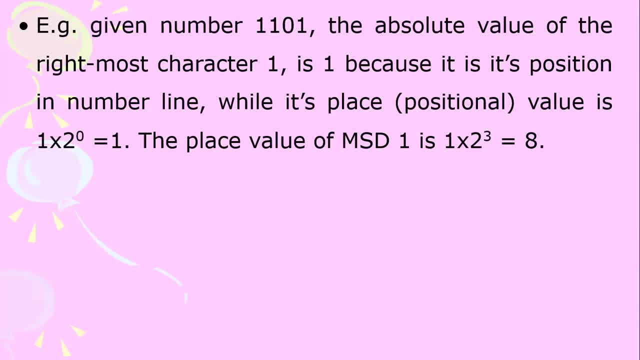 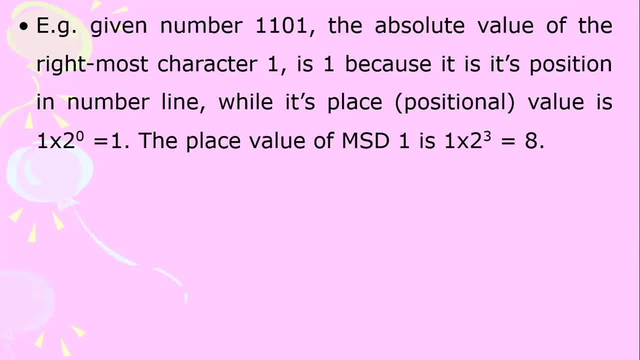 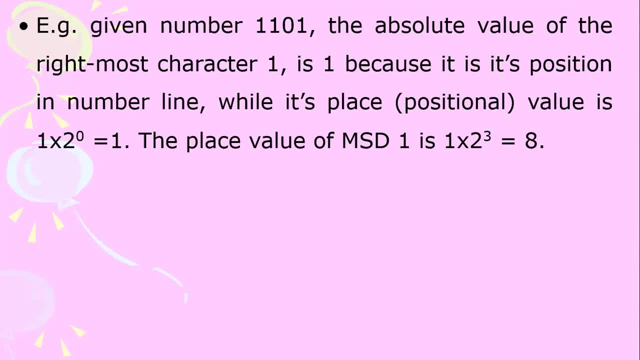 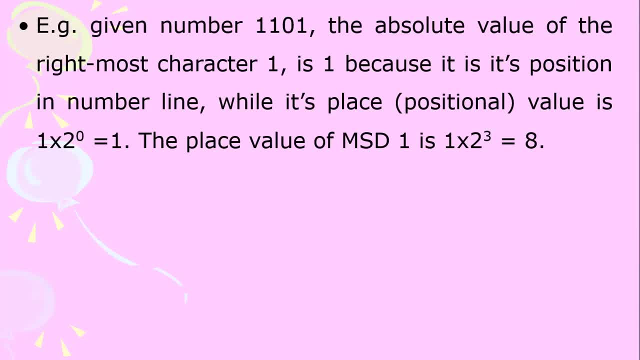 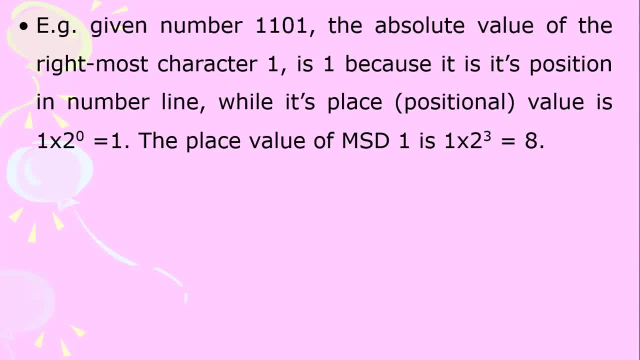 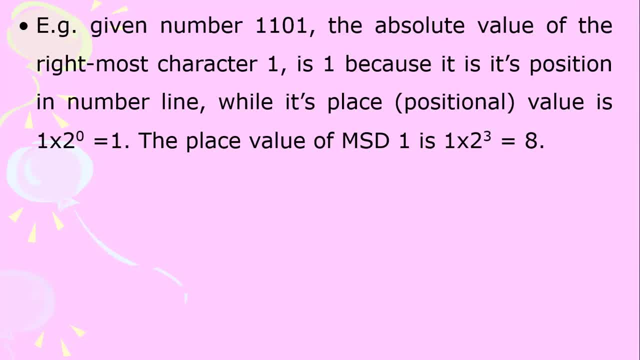 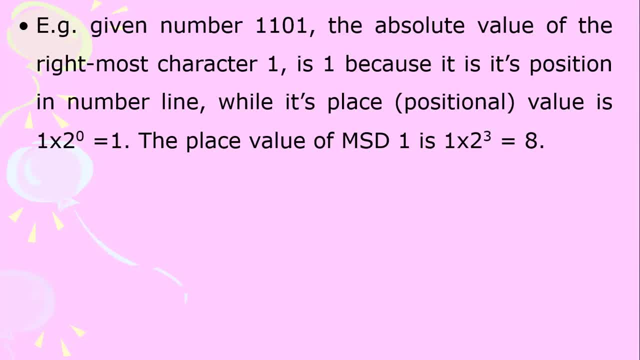 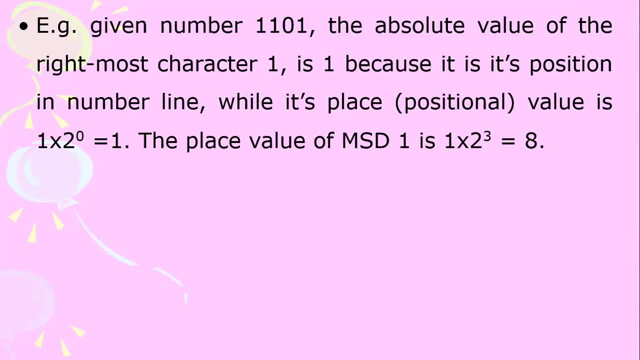 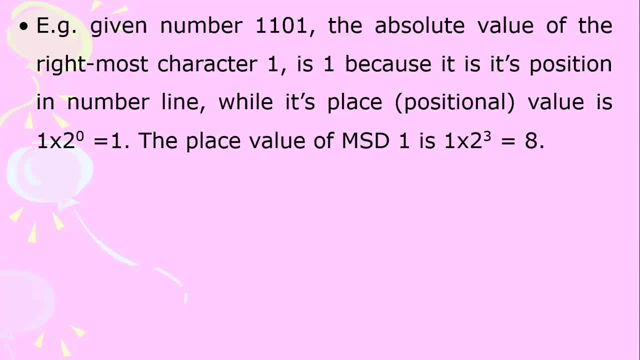 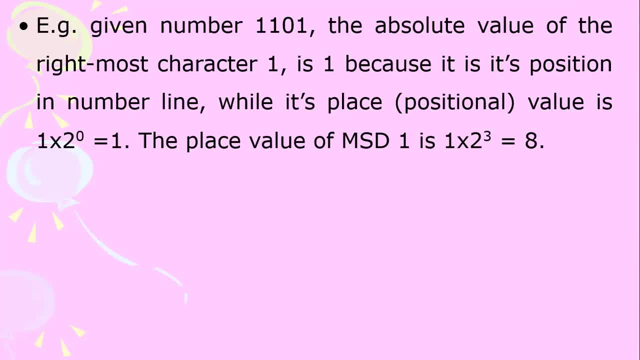 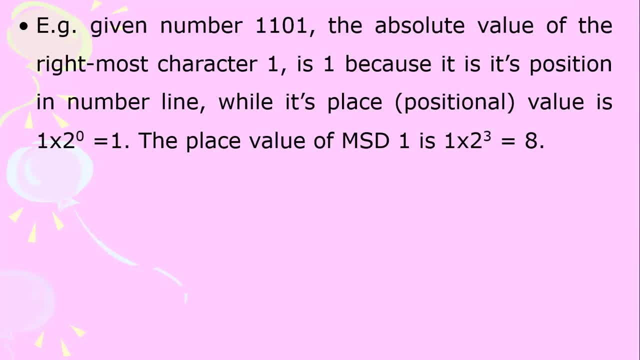 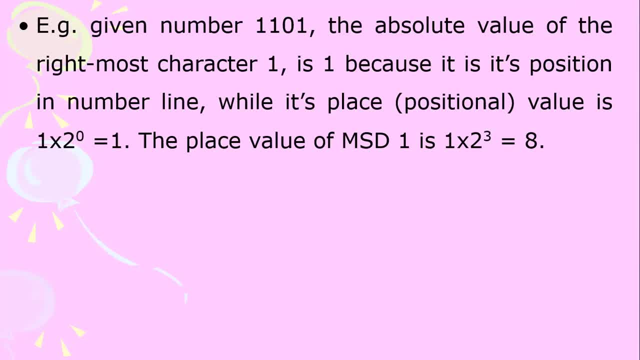 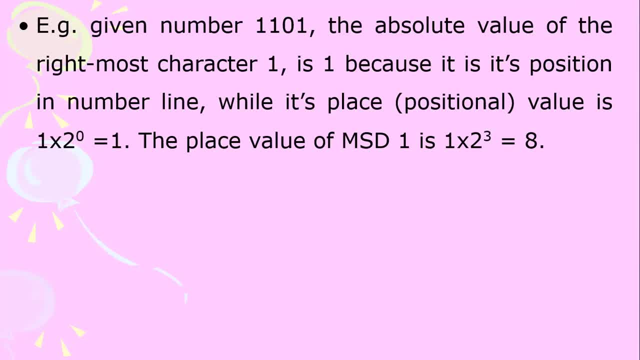 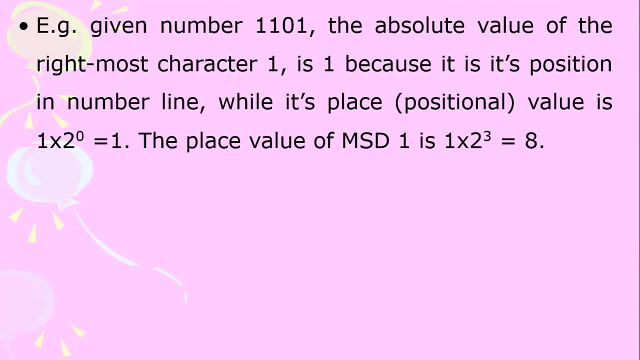 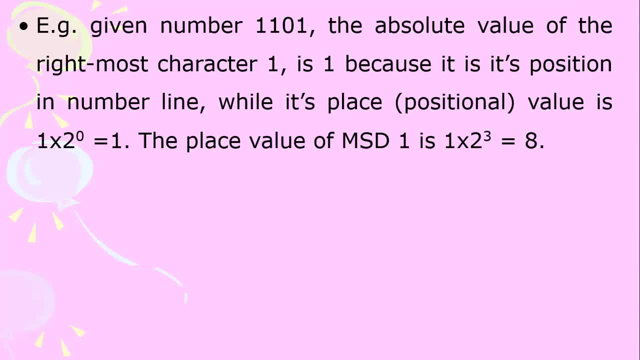 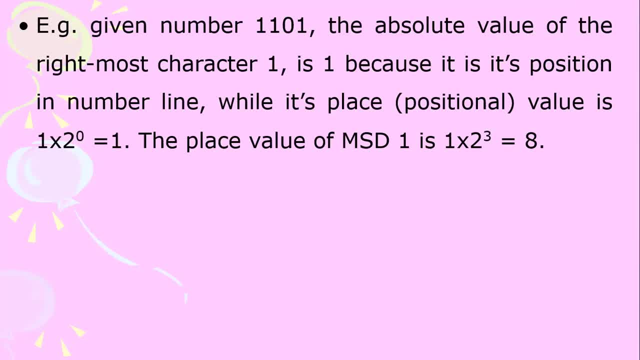 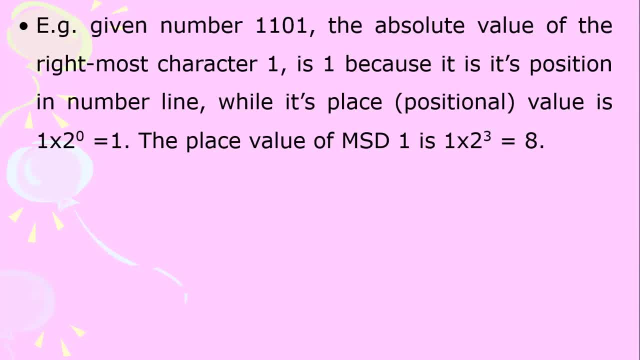 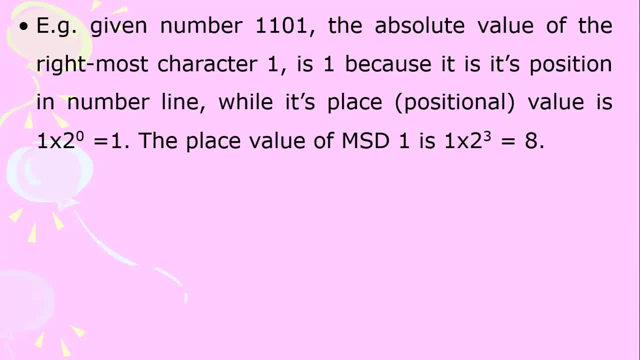 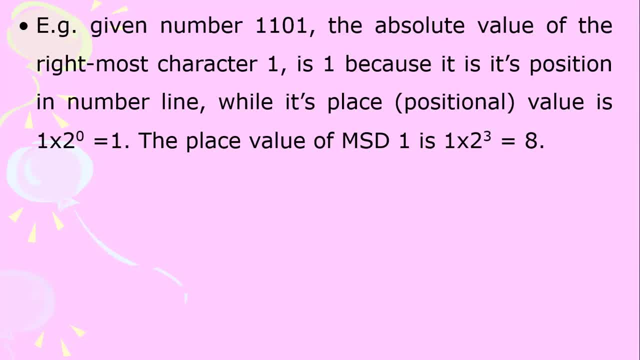 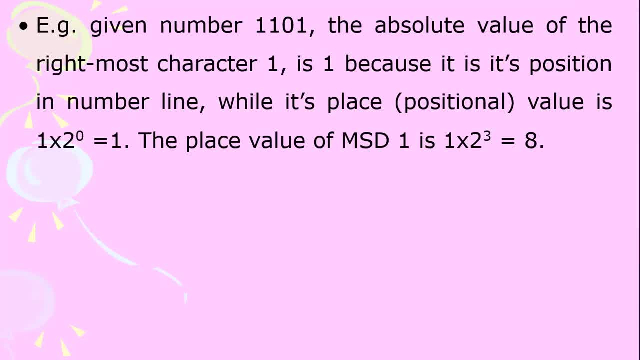 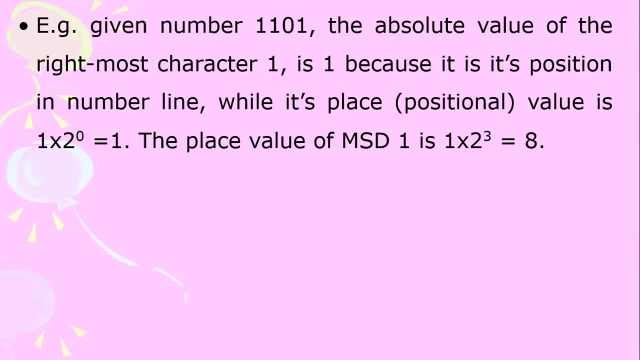 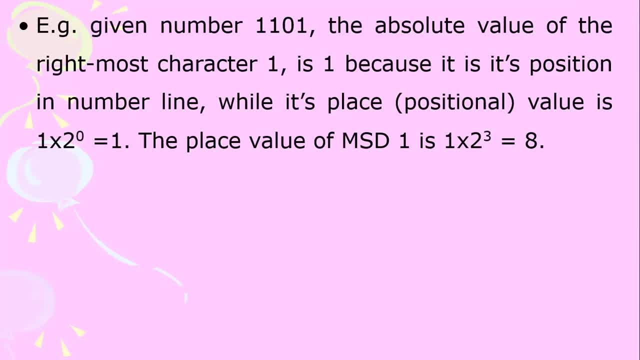 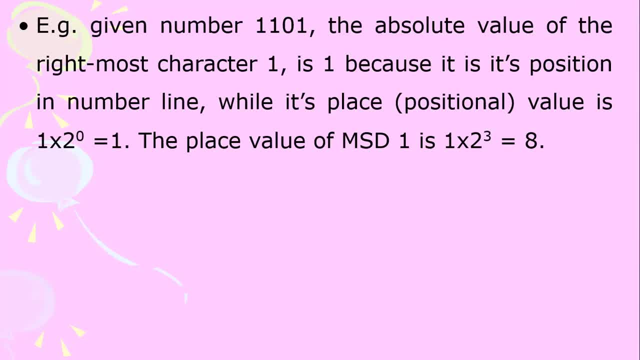 that number with the number which represents the number system, multiplied by or raised with one, etc. So in this case, because we are computing the positional place value of one, which is our least significant digit in the number one, one, zero one, then we get that positional. 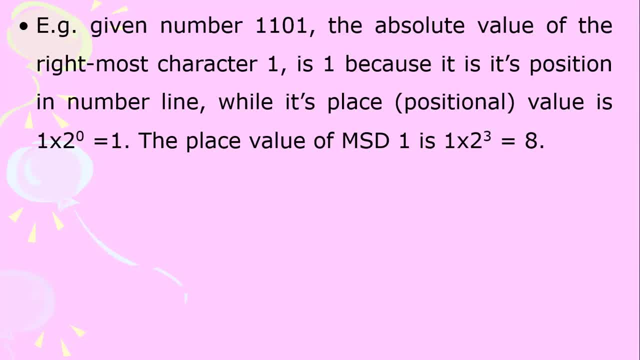 value as one times two. two which of course indicates binary raised to zero, which gives one times one One, Because any number raised to power zero gives one. So it is one times one, which is equals to one. However, the place value of our most significant digit, which is one, on the left-hand side. 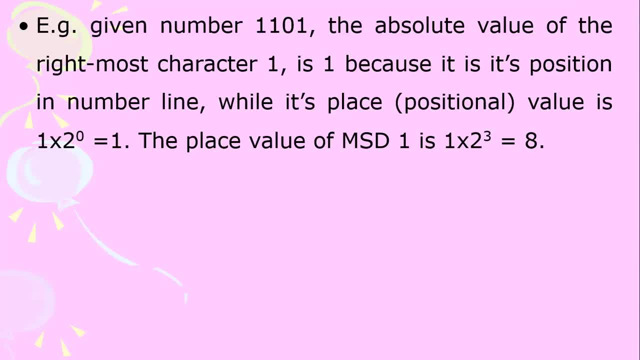 is one, So we raise one times two to power three. Note: just as I have said, we raise our numbers with zero from the least significant digit assigned or position. As we move towards the right or the left-hand side, we raise our numbers. 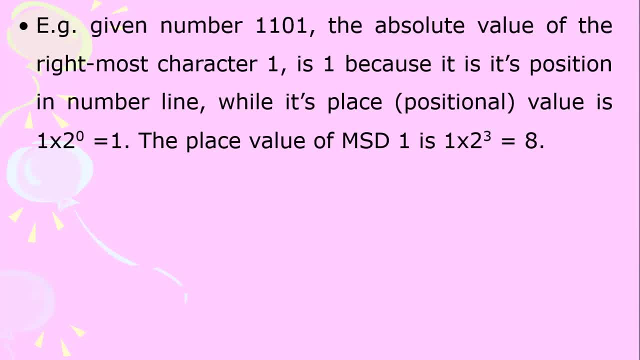 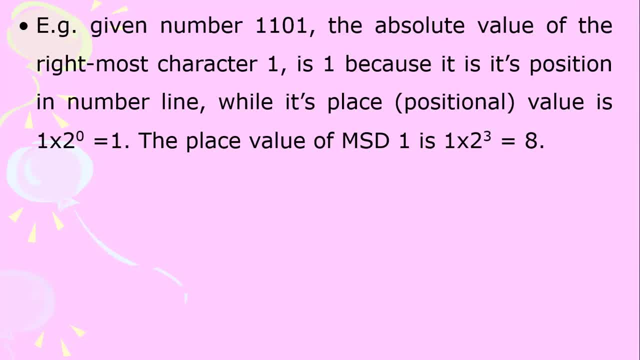 all the way. For example, in our number one, one zero one. then to get the positional value of the least significant digit, one, it is one times two, because it is binary. raised to zero, The positional value is zero. 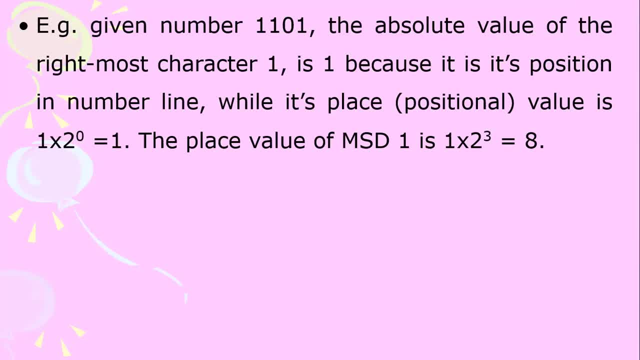 value of zero. in that order, in that number will be zero times two raised to power one. Then our next one, in that order as we move to one, the most significant digit will be one. that is, that number times two represent the number system raised to power two. 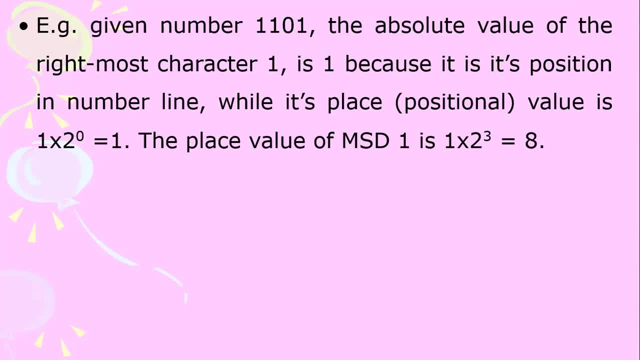 And, lastly, the most significant digit in this case, which is one, and it is our leftmost character, it will be one, that is the number itself times two, Then from the number system, then raised to power three. In other words, we raise numbers using the criteria zero, one, two, three, four, five, six. 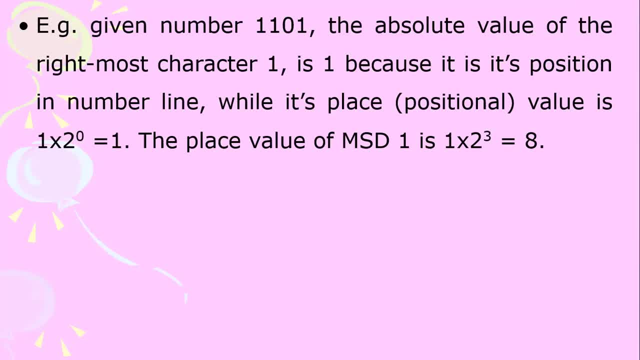 like that, based on the number of characters or the number of digits in our number, In the number we are dealing with. My dear students and the rest of the learners, you will gain more understanding and deeper understanding as you proceed from this presentation and then you visit Emily Sw counterparts. 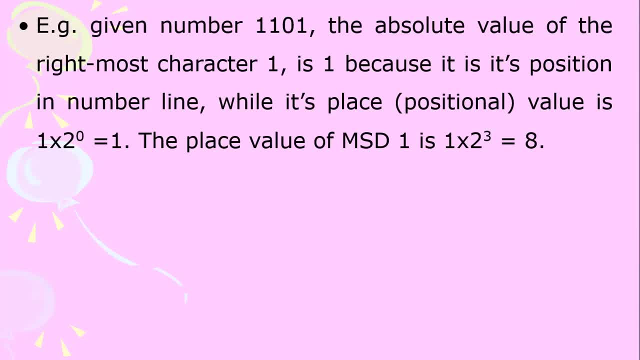 institute YouTube channel for part two or three of this presentation and then part three of three in this series. Therefore, the place value of our most significant digit one will be one. Therefore, the place value of our most significant digit one will be one. Therefore, the place value of our most significant digit one will be one. 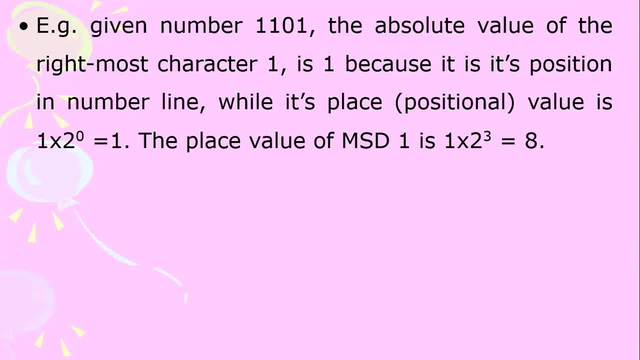 is 1 times 2 to power 3.. 2 to power 3 means 2 multiplied by 2 multiplied by 2.. That is 2 multiplied by itself. 3 times 2 times 1 is 2.. 2 times 2 is 4.. 2 times 2 times 2 is. 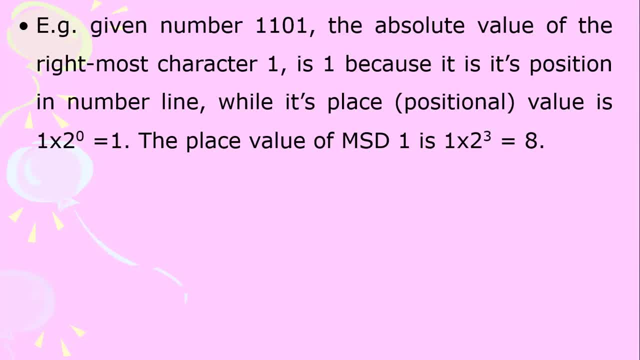 equal to 4 times 2,, which is equal to 8.. 1 times 8 gives 8.. So the base value of 1, 1, 0, 1 is 2.. Why? Because it is, in binary number system, To the left of the binary number. 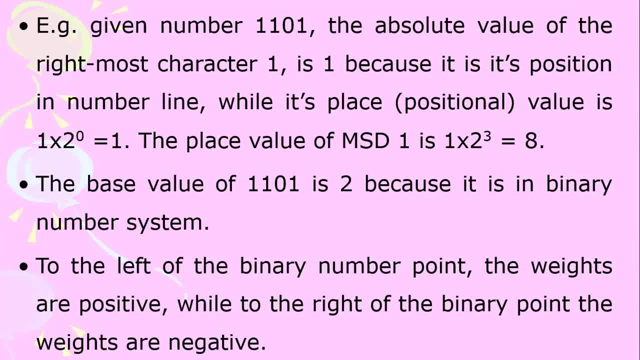 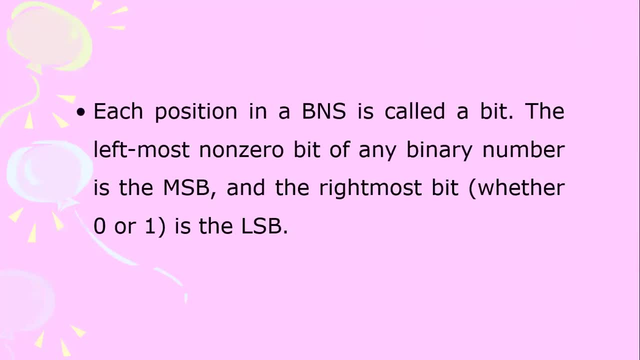 point the weights are applied To the right of the binary point. the weights are normally negative. Each position in a binary number system is called a bit. The leftmost known zero bit of any binary number is the most significant. So the leftmost known zero bit of any binary number is the most significant. So the leftmost. 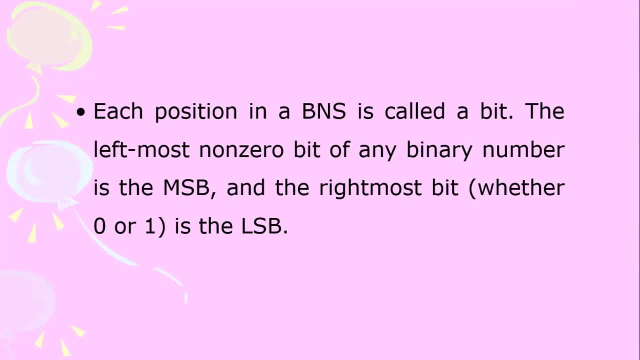 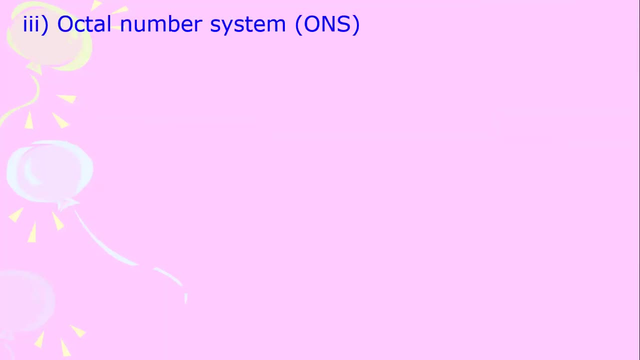 known zero bit of any binary number is the least significant bit And the rightmost bit. whether 0 or 1 is the least significant bit. Let's now pay our focus on octo-number system, ONS. This is a system of representing characters. 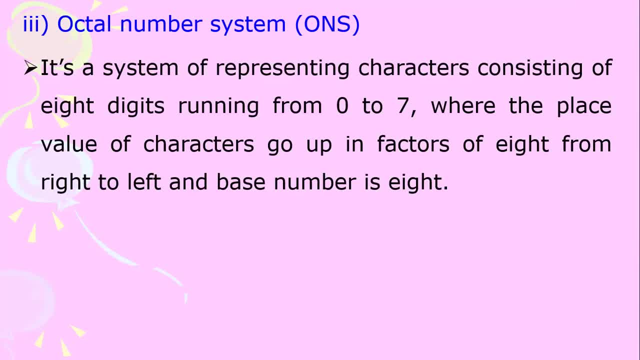 of 8 digits running from 0 to 7, where the place value of characters go up in factors of 8 from right to left and base number is 8.. The place value of 6,, for example, in the following number, is 8.. 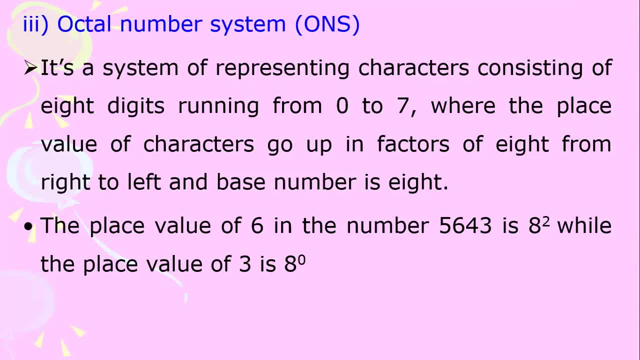 The place value of 7 is 8.. And the place value of 7 is 8.. The combination of the 2 numbers is 6.. What else? The third term, the천th term, is 1. And the fourth term, the turn term, will be 7.. 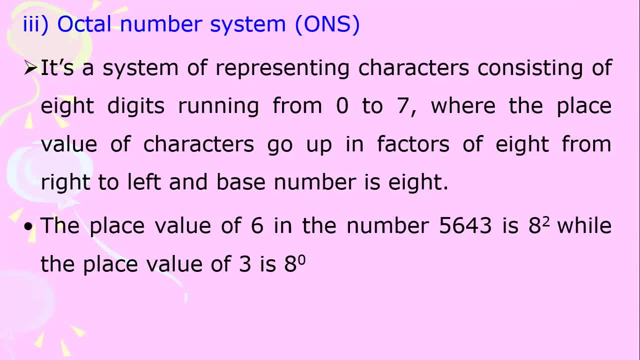 The turning term side term is 2.. The Russian poisoned two of them and then run to the floor and they cross its rhymes again and chase each other until the dot equals 7.. In the last row, the hand is always changed to the last one and the hand is always pressing. 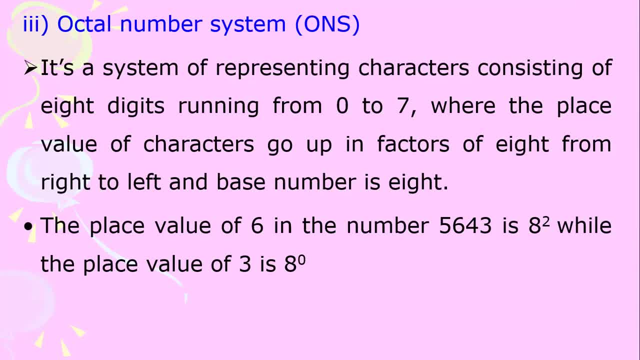 to the left, depending on the position of the biod�들ant digit minus of root two. So the hand always getting other number and you can point the hand as 거� Windows returns to the zero. The hand also punishes a generated value of the rabble for each part of the featured. 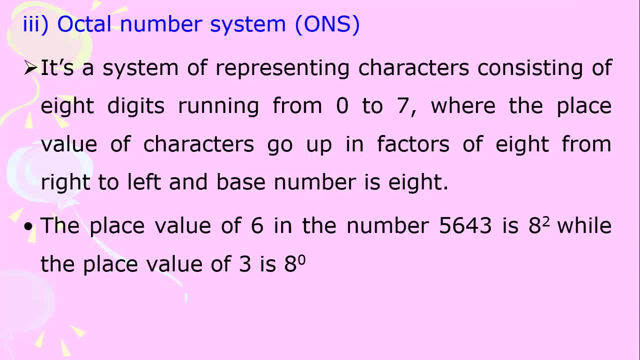 integer will be eight raised to zero, Five, six, four, three in octo. simply indicates that. simply indicates that three, three, that three is the least significant digit in this number system, while five is the most significant digit, While five is the most significant digit. 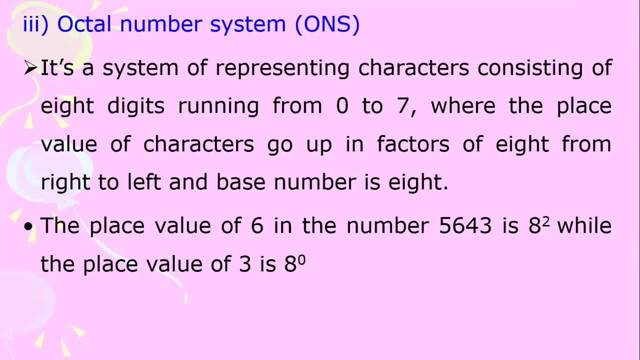 And therefore, to get the place value of our least significant digit, which is three, it simply means we shall multiply eight with eight raised to power zero. So I repeat what I have already said, My dear students and the rest of the learners, 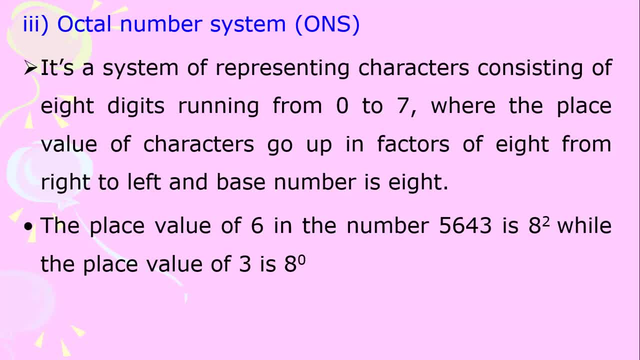 you have already learned how to go about the binary number systems and the decimal number systems. So the formula of dealing with the octo number systems is similar to the one for the octo and to the one that is to the one of decimal and to the one of binary. 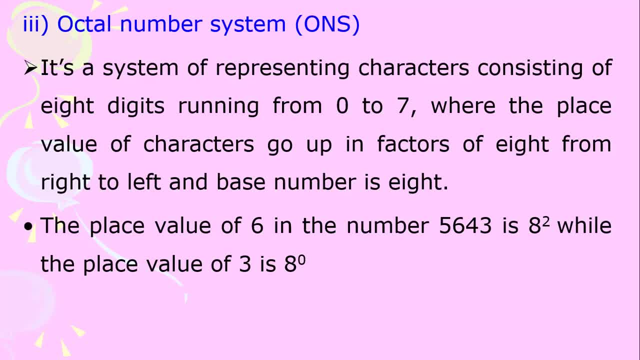 The only difference this time round is that now, wherever we are using two for the base and wherever we are using ten for the base, we are now replacing it with eight, because we are now dealing with an octo number system And therefore I have said: 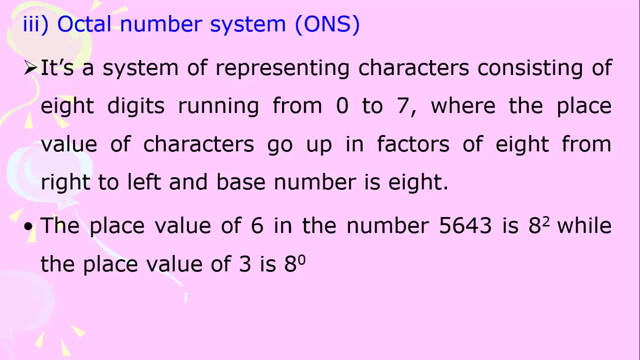 that if, for example, given the number 56 or 5643, 5643, to get the place value of any of those digits, you pick that digit and then, based on its position, you raise that digit and also you pick the base, which is eight, you raise it to the respective power, based on the position. 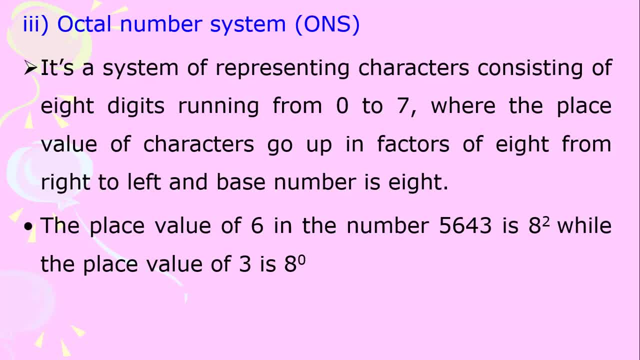 So for three, the place value will be eight raised to zero. For four, it will be eight raised to one. For six, it will be eight raised to two, While for five it will be eight raised to three. So we move from the powers zero, one, two, three, etc. moving from the least significant digit. 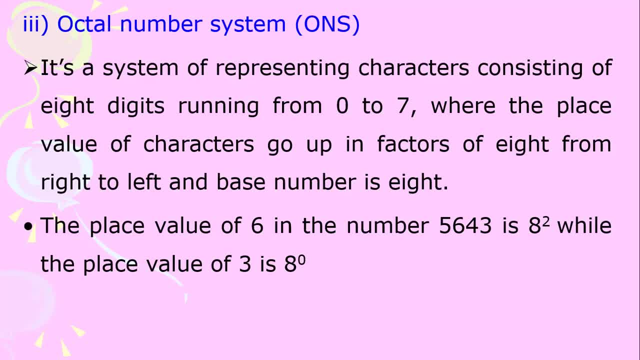 to the most significant digit in that order. That's why we are therefore saying that the place value of six in the number 5643 is eight raised to two, or the place value of three, which is the least significant digit, is eight raised to zero. 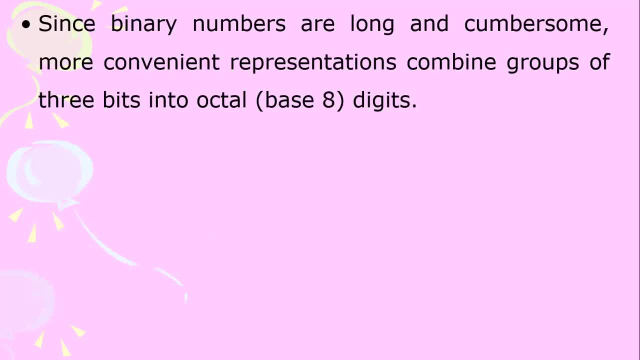 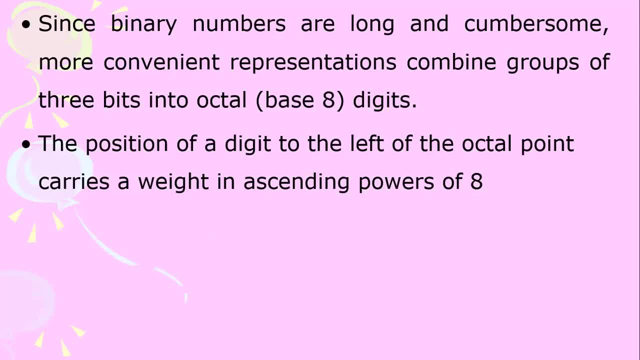 that is, these eight digits. The position of a digit to the left of the octopoint carries a weight in ascending powers of eight. just as I have already explained, digits behind the octopoints are used and are similar to decimal and binary points. 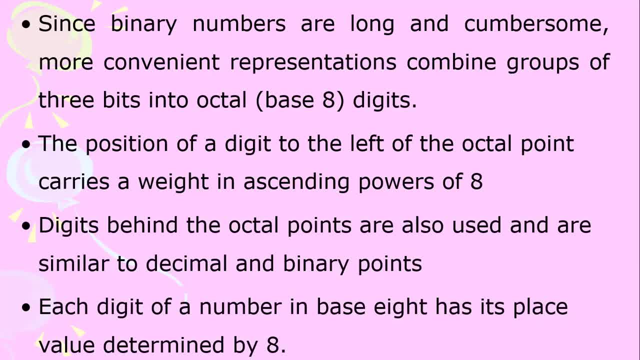 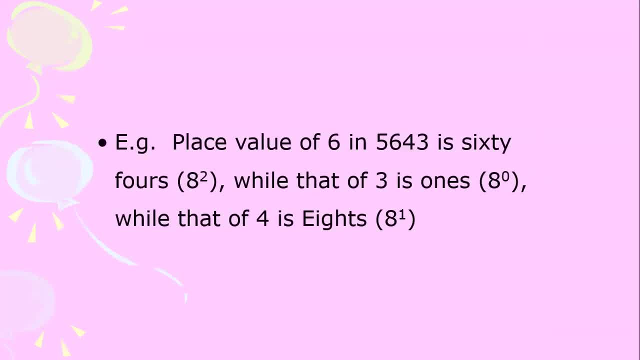 each digit of a number in base 8 has its place value determined by 8. for example, the place value of 6 in 5, 6, 4, 3 will be 64, because it is 8 raised to power 2. well, that of 3 is once, because it is 8 raised to 0. well, that of 4. 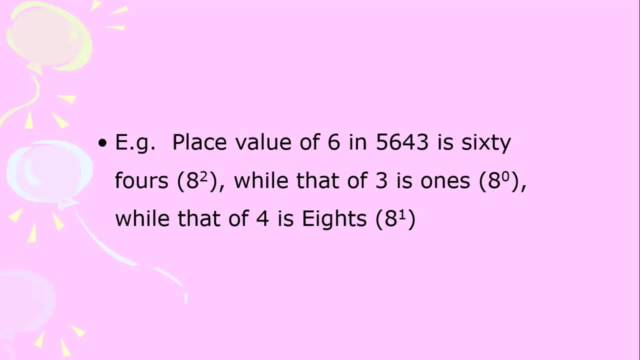 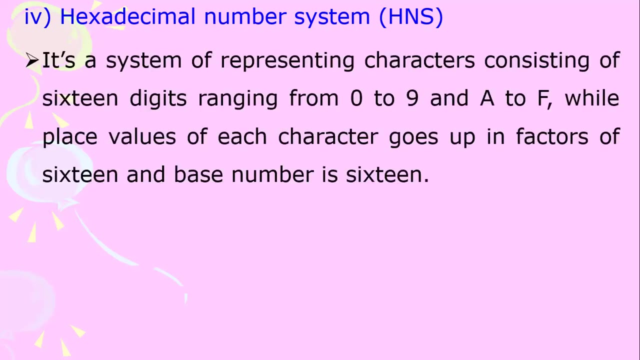 is 8, because it is 8 raised to power 1. let's now look at hexadecimal number system h and s. this is a system of representing characters consisting of 16 digits, ranging from 0 to 9 and a to f, where place values of each character goes up in factors of 16. 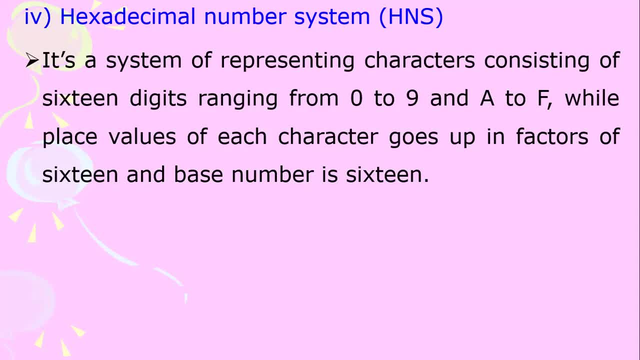 and base number is 16.. my dear students and the rest of the learners, kindly note that whereas we have said that an hexadecimal consists of 16 digits spanning from 0 to 15, the numbers behold 9 are not represented as decimals. in other words, we don't write them as 10. 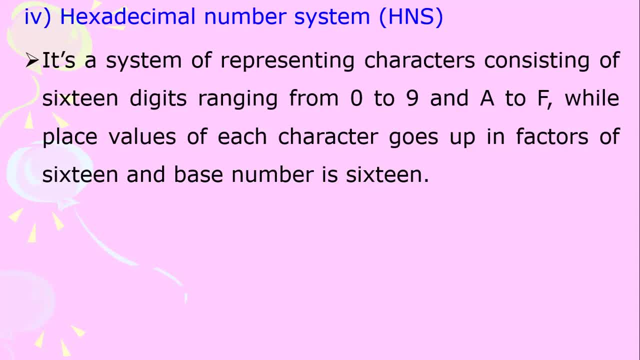 11., 11., 12., 13., 14. and 15.. but we replace any number beyond the 9 with letter a to f and therefore our 16 digits range from 0 to 9 and a to f, that is, 01, 2.. 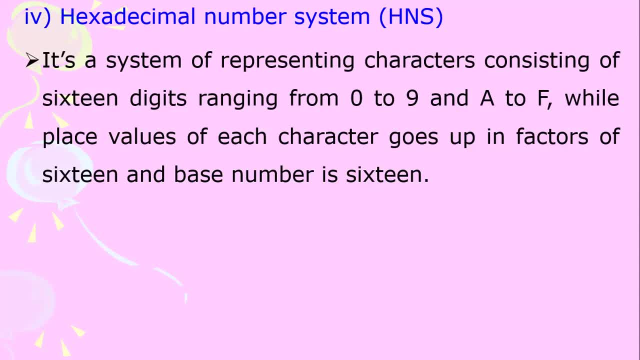 3. 3,, 4,, 5,, 6,, 7,, 8,, 9,, A, B, C, D, E, F. Therefore, 10 is represented as A, 11 as B, 12 as C, 13 as D. 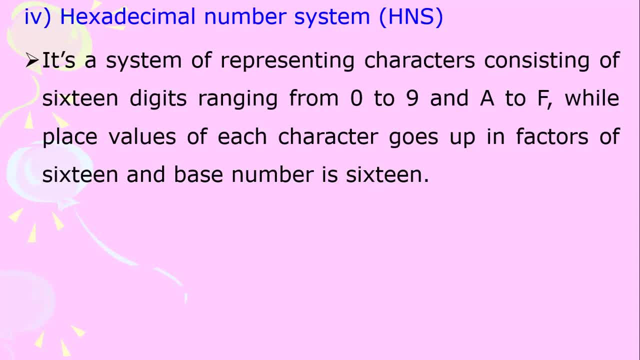 14 as E, 15 as F And therefore A is equivalent to 10 and F is equivalent to 15 in this 10 system. This therefore informs you that 11 is equivalent to B, 12 is equivalent to C, 13 is equivalent to D, 14 is equivalent to E and 15 is equivalent to F. 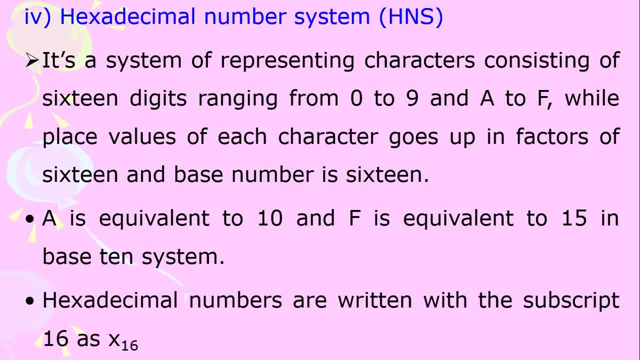 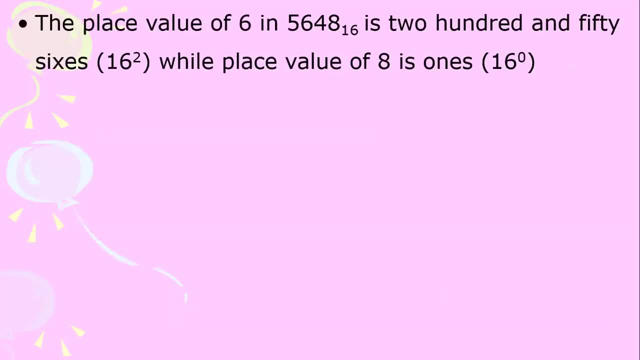 Exandesimal numbers are written with the subscript 16 as X to be 16.. The place values of 6.. For example, in the same example I've been giving, but now in base 16, that is, 56, or 5,, 6,, 4,, 8.. 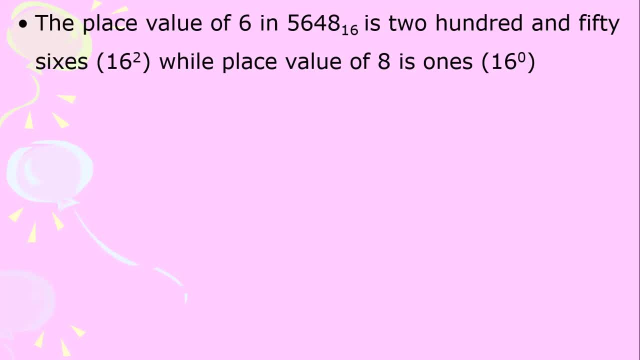 My dear students and the rest of the learners, kindly listen to the way I am reading my numbers, Except for the decimal, where I write it as 5, 648. for the octo binary and exandesimal, I am reading them in a different way. 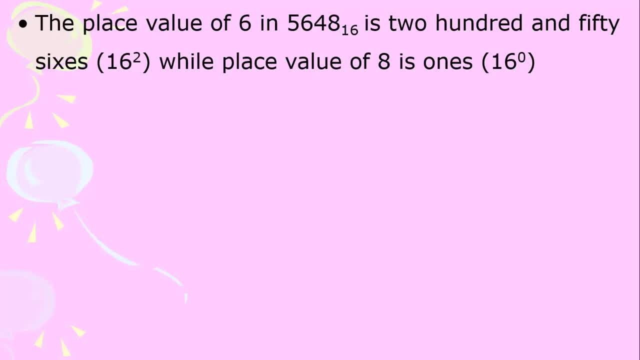 I am not saying 5, 648 to base 16.. No, I am saying 5, 6,, 4, 8 to base 16.. 5, 6, 4, 8 to base 16.. 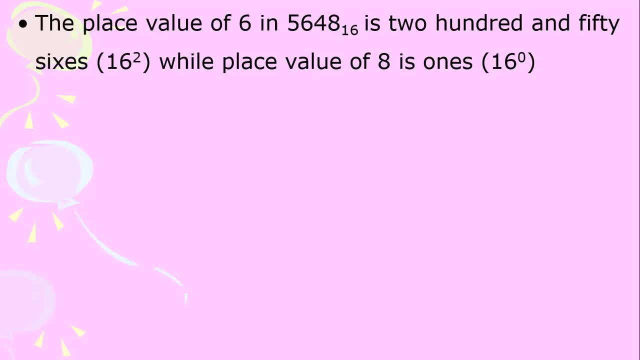 Why? Because 5,, 6,, 4, 8 to base 16.. Is not equivalent to 5, 648 in decimal, That is, to base 10.. Those are different numbers. Neither is it equal to 5,, 6,, 4, 8 in octo. 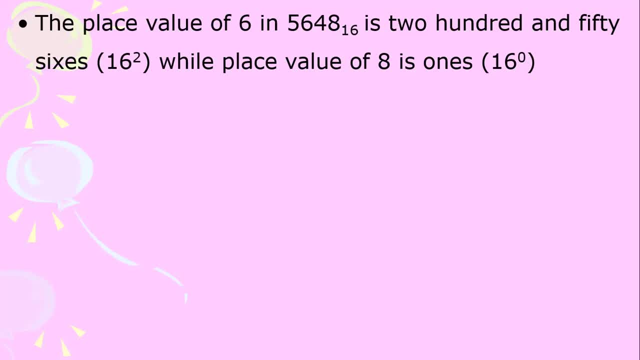 So the place value of 6 in 5,, 6,, 4, 8 exandesimal is 256.. Why? Because it is 16 raised to power 2.. For 8, it is 16 raised to 0.. 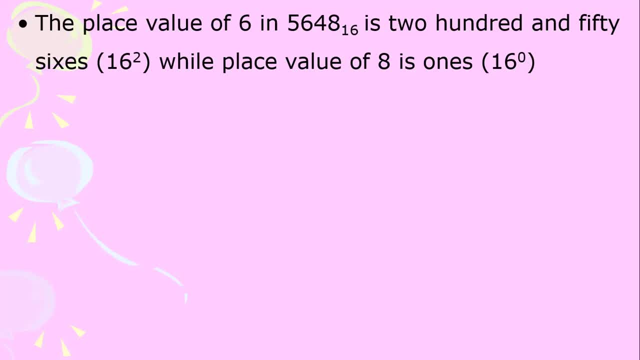 For 4, it is 16 raised to 1.. For 6, it is 16 raised to 2.. For 5, it is 16 raised to 3.. The difference between The exa in this case and the octo that we have dealt with is we are replacing 8 with 16.. 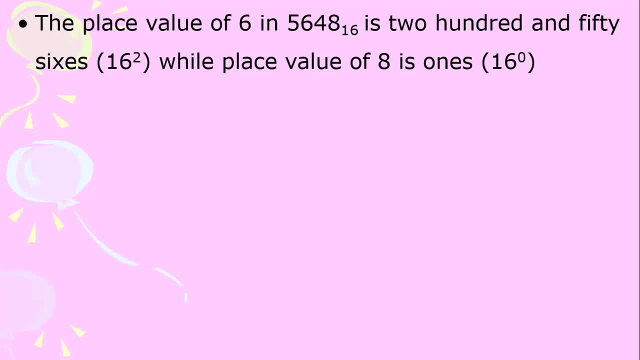 So the place value of 6 in 5,, 6,, 4, 8 exandesimal is 256.. Because it is 16 raised to 2.. While place value of 8 is 1.. Because it is 16 raised to 2.. 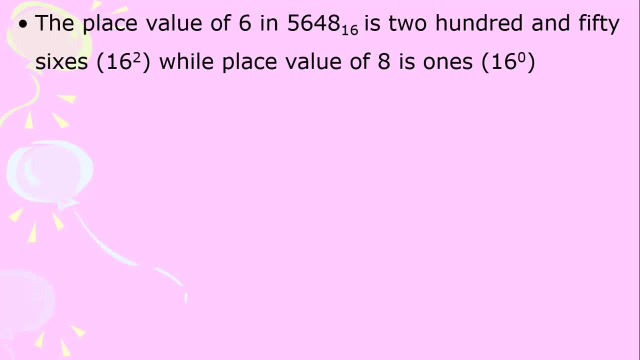 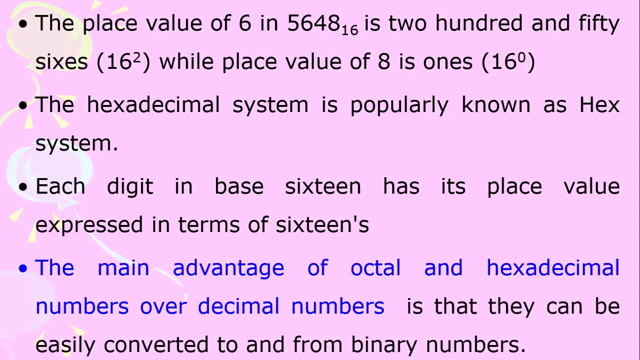 Because it is 16 raised to 0, which gives a 1.. The exandesimal system is popularly known as hex system. Each digit in base 16 has its place value expressed in terms of sixteenths. The main advantage of octo and exandesimal numbers over decimal numbers: 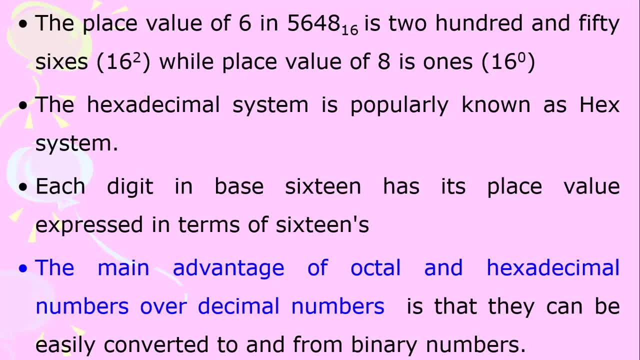 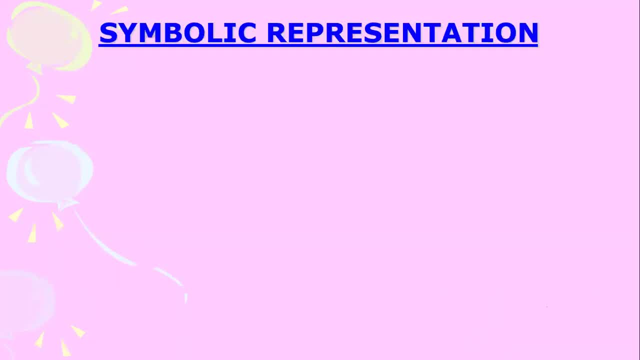 is that they can be easily converted to and from binary numbers. Let's now look at what we call symbolic representations. in data representation In computing, a single character, such as a letter, a number or a symbol, is represented by a group. Inijeơ's example. you see it. 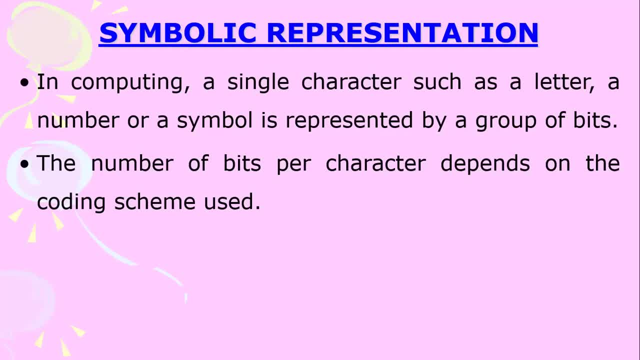 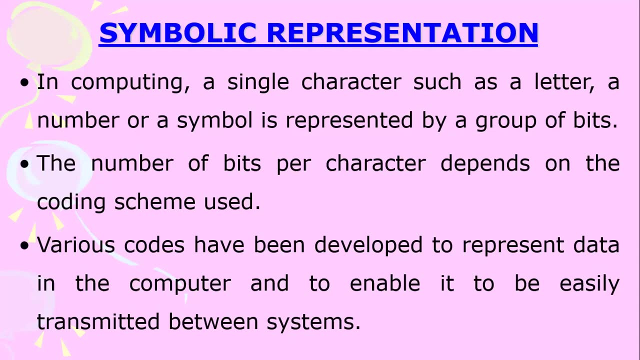 The tree is a few bit and it connects to the number of bits. The number of bits per character depends on the coding scheme that is used. Various schools have been developed to represent data in the computer And enable it to be easily transmitted. 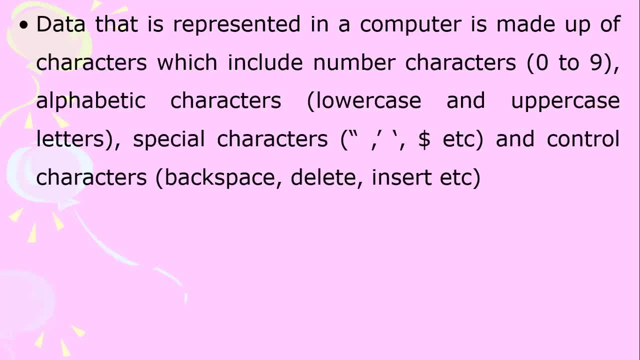 between systems data. thately is made up of characters, which include number characters 0 to 9, alphabetic characters, that is, lowercase and uppercase letters. We have special characters and control characters, such as backspace, delete, insert, etc. And all these characters. 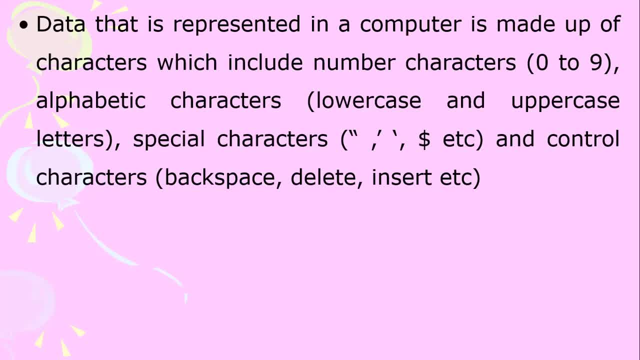 need to be represented in the computer, not in using the normal binary, the normal octos, the normal hexadecimals, but using now a special or a set of special symbols, A set of special symbols, What we are calling special or what we are calling 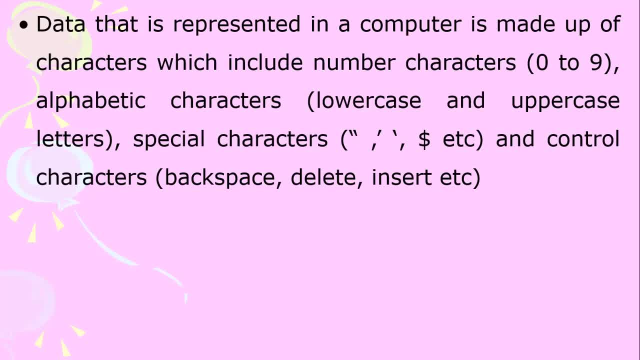 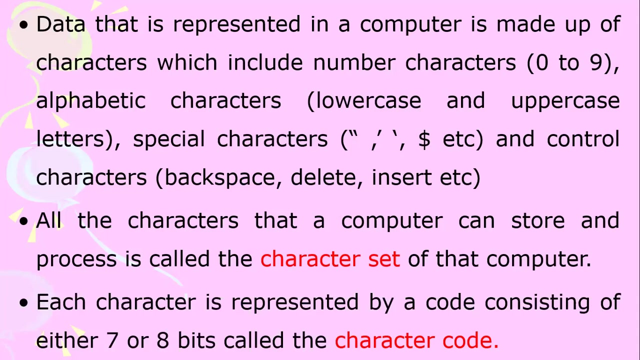 symbolic representations. So all the characters that a computer can store and process is called the character set of that computer. All the characters that a computer can store and process is called the character set of that computer. Each character is represented by a code consisting of: 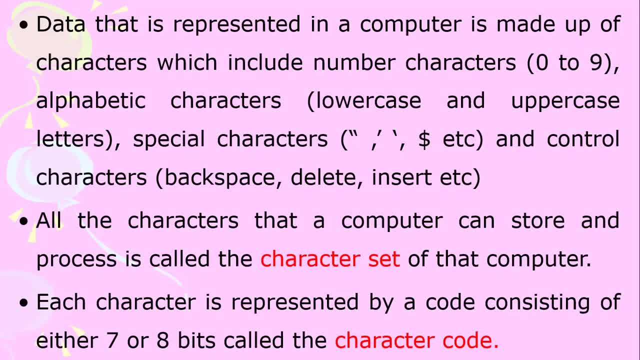 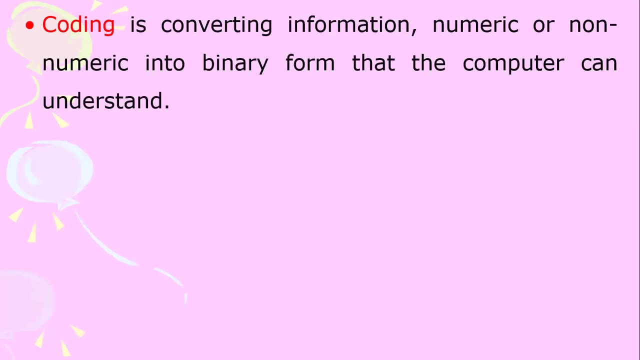 either seven or eight bits called the character code, But the most common one is the eight bits, which are equal to a byte. Coding is converting information, numeric or non-numeric- into binary form that the computer can understand. Therefore, coding is the process of converting. 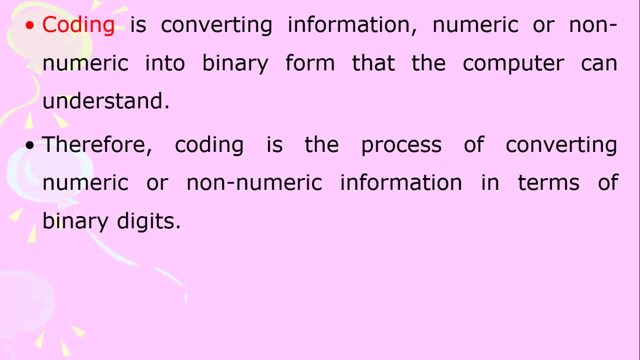 numeric or non-numeric information. in terms of binary digits, The most common coding schemes are BCD, FCD and ASCII. The most common coding is BCD, MCD and ASCII. Let's look at BCD. This is a. 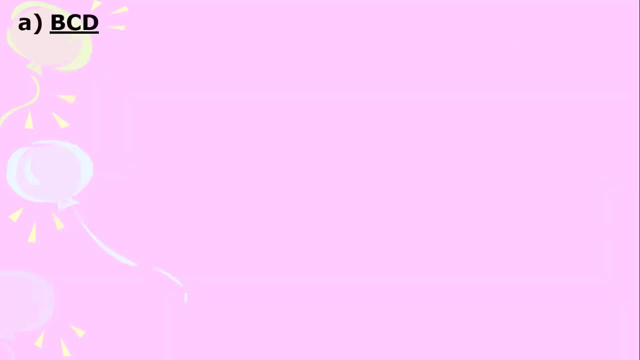 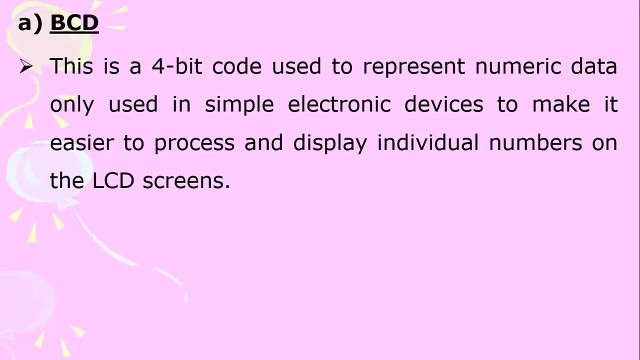 four-bit code used to represent numeric data only used in simple electronic devices to make it easier to process and display individual numbers in the computer. This is a four-bit code used to represent numeric data only used in simple electronic devices to make it easier to process. 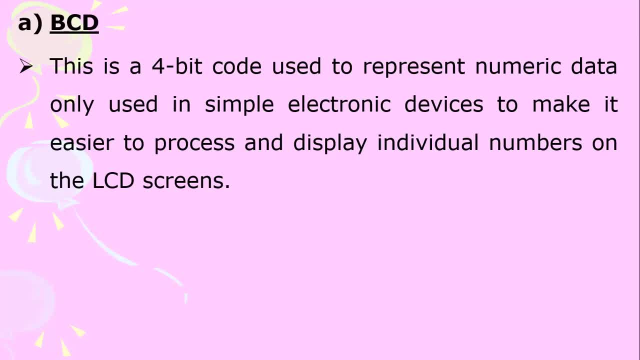 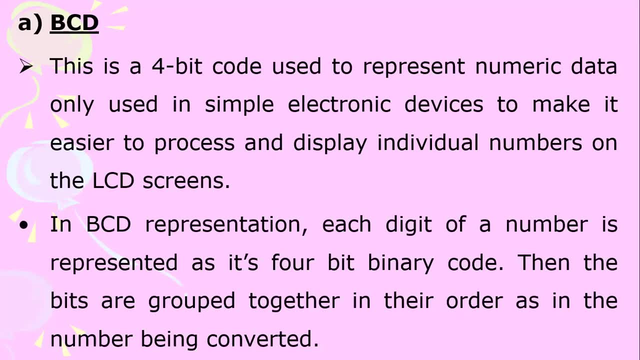 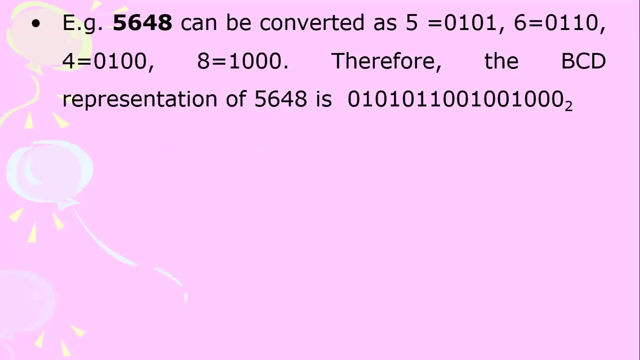 and display on the LCD screens. In BCD representation, each digit of a number is represented as its four-bit binary code. Then the bits are grouped together in their order, as in the number being converted. For example, 5, 6,. 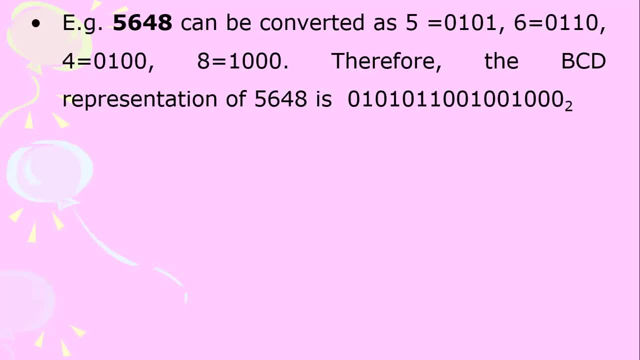 4, 8 can be converted as: 5 is equals to 0, 1, 0, 1.. 6 is equals to 0, 1, 1, 0.. 4 is equals to 0,. 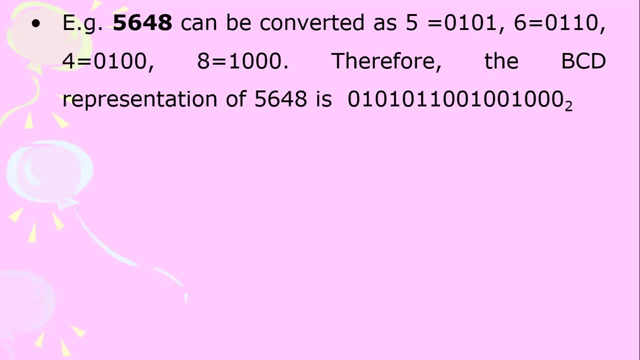 1, 0, 1, 0.. Therefore, the BCD representation of 5, 6,, 4, 8 will be 0, 1, 0, 1, 0, 0, 1,. 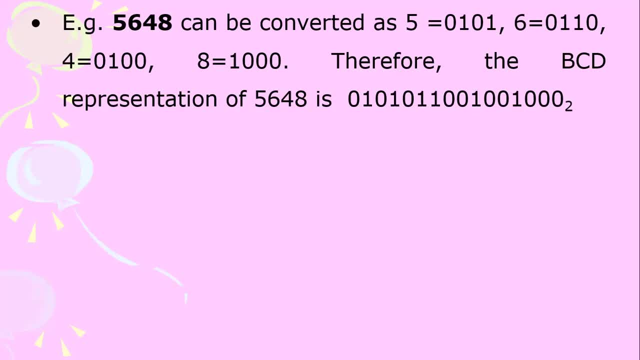 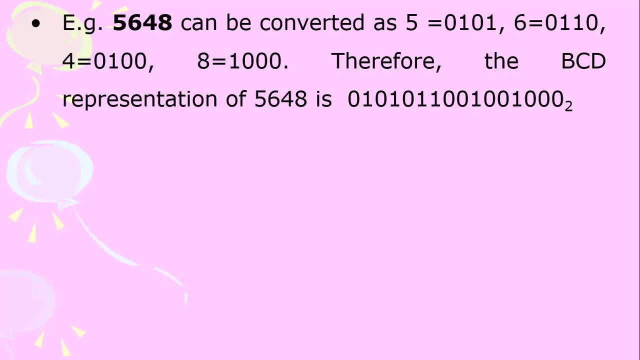 happy to be able to know how we do number combinations from one number system to the next. Kind of visit ML, SWAP I CT YouTube Channel and look and listen to. To represent a signed number, that is integer, which is with a positive or a negative sign. 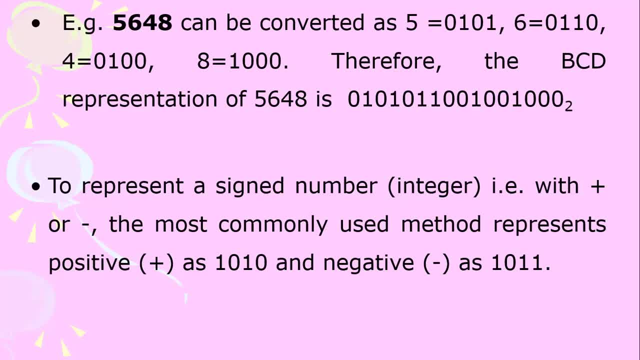 the most commonly used method, represents positive as 1010,, in other words, represents the addition sign or plus sign, that's a positive sign as 1010,, while the negative sign is represented as 1011.. So if you have a number that commences with plus or minus, that is a dash negative or positive number. 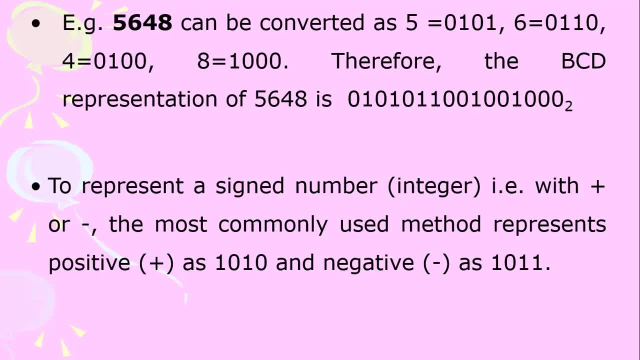 a number indicates positive. So if you have a number that indicates whether, or a symbol, a symbol that indicates whether the number is negative or a positive, either addition sign or the subtraction or minus sign or negative sign, then we replace or we indicate the positive sign with 1010 and the negative sign with 1011.. 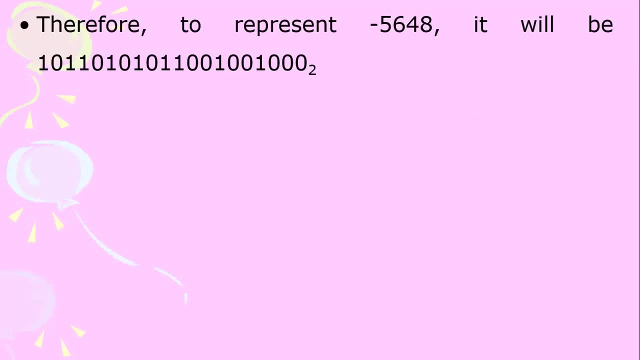 Therefore, to represent the number negative 5648, note I am not saying minus 5648,, I am reading it as negative 5648. It will be 1011.. 1011 represents the negative sign. So it is 1011, 0101, 01, 100, 100, 100, 1000, to base 2.. 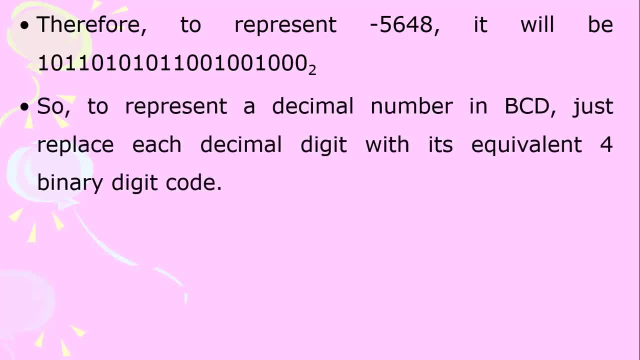 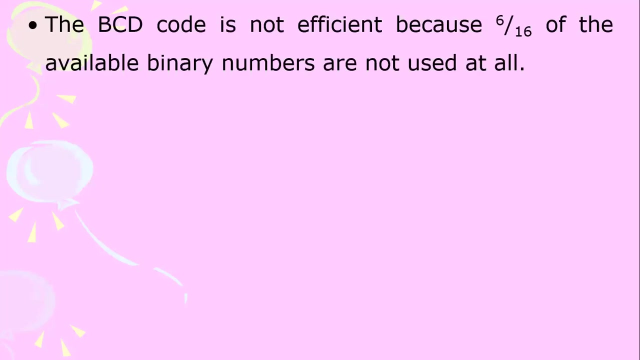 So to represent a decimal number in BCD, just replace each decimal digit with its equivalent for binary digit code. Although the number 10 through 15 could also be coded as four digit binary numbers, this is not done in BCD. The BCD code is not efficient because 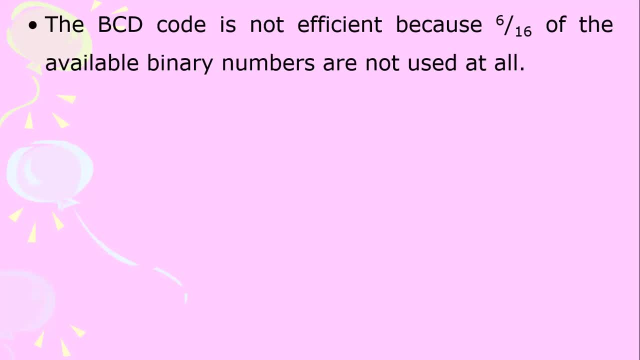 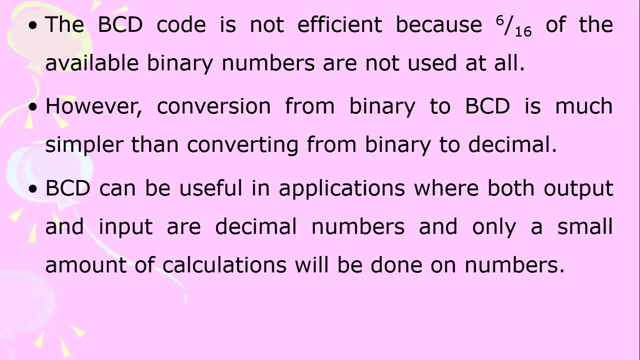 6 over 16 of the available binary numbers are not used at all. However, number or conversion from binary to BCD is much simpler than converting from binary to decimal. BCD can be useful in applications where both output and input are decimal numbers and only a small amount of calculations will be done on the numbers. 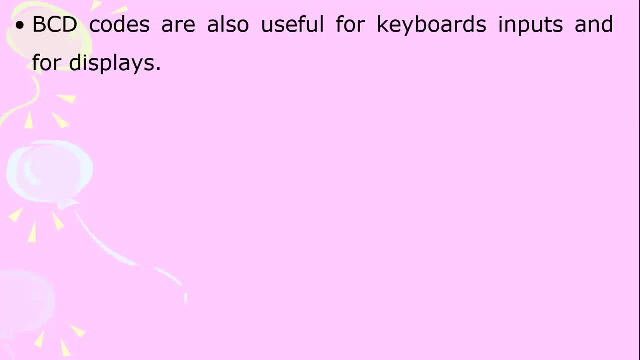 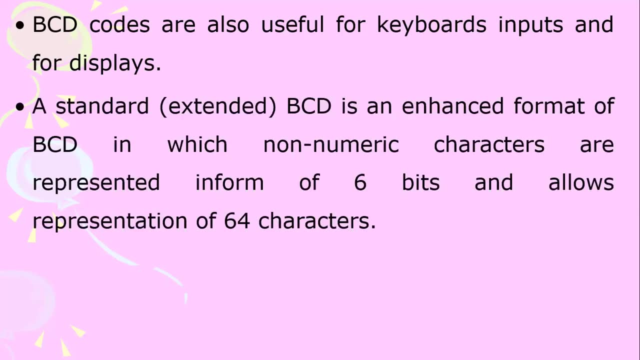 BCD cones are also useful for cables, inputs and for displays. A standard or equivalent of BCD cones is BCD. Extended. BCD is an enhanced format of BCD in which non-numeric characters are represented in the form of 6 bits and allows representation of 64 characters. 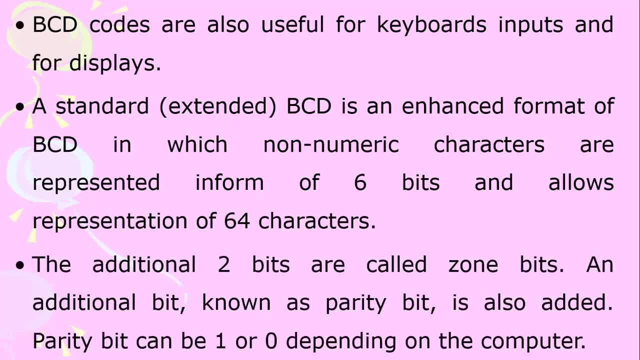 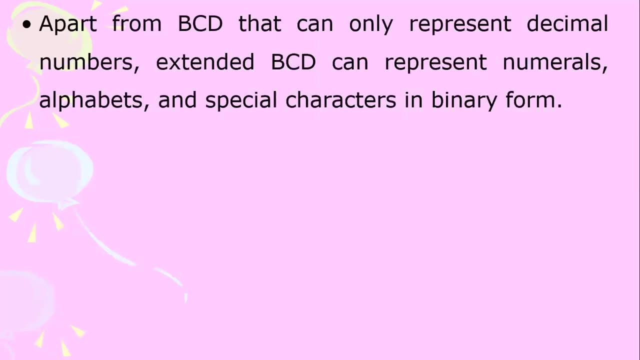 The additional 2 bits are called zone bits. An additional bit known as parity bit is also added. Parity bit is also added. Parity bit can be a 1 or a 0, depending on the computer. Apart from BCD that can only represent decimal numbers, extended BCD can represent numerals, alphabets and special characters in binary form. 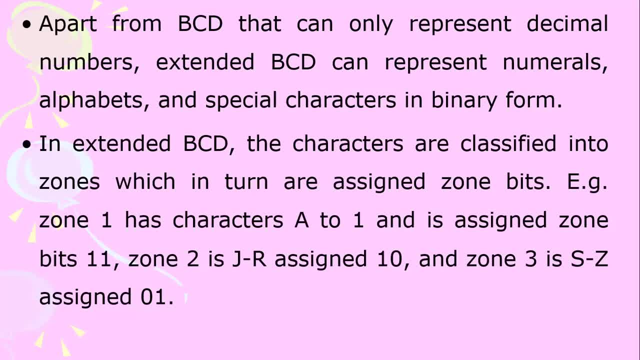 In extended BCD the characters are classified into zones which in turn are assigned zone bits. For example, zone 1 has characters a to 1, and is assigned zone bits 1, 1.. Zone 2 is characters j to r. 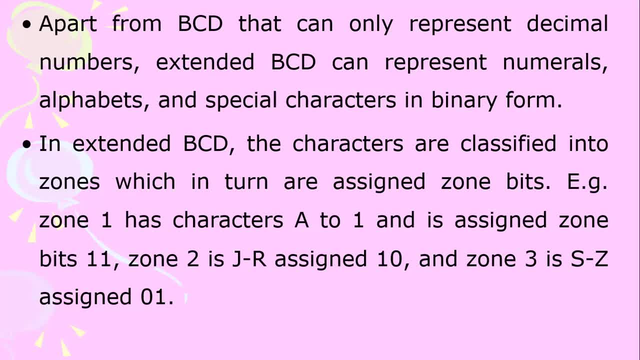 assigned 1, 0.. And zone 3 is characters s to z, assigned 0, 1.. So if a number in extended BCD begins with or commences with 1, 1,, then you can tell it is within zone A. 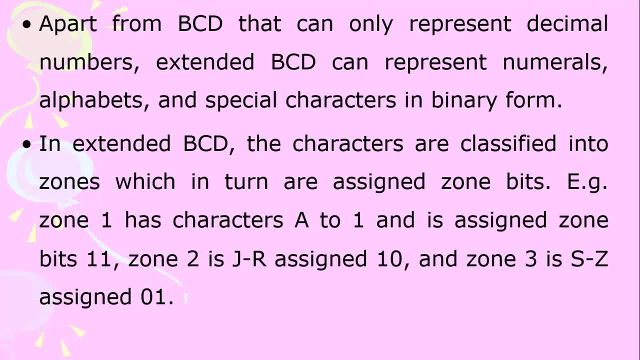 If it commences with 1, 0,, you can tell it is in zone B or zone 2.. If it is represented as 0, 1,, then you can tell that that is zone 3.. And therefore you can easily look at the binary representation of a character. 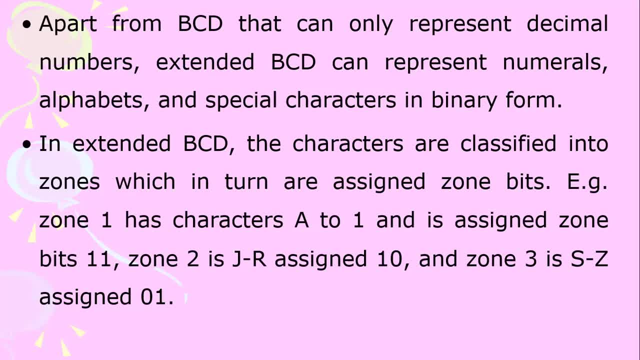 and tell whether it is in zone A Or whether that is A to the character preceding: j, A, B, C, D, E, F, G, H, I. So zone A will span from A to I, Not A to 1, but A to I. 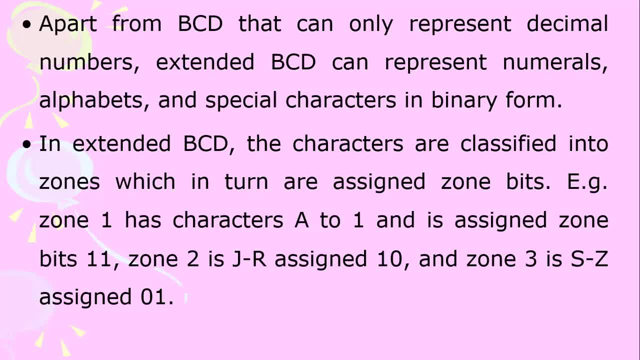 I repeat: For example, zone 1 has characters A to I, Not A to 1,. as I had said before, It is A to I. So any character, so any number or any character represented, with the first or most significant digits being 1,, 1,. 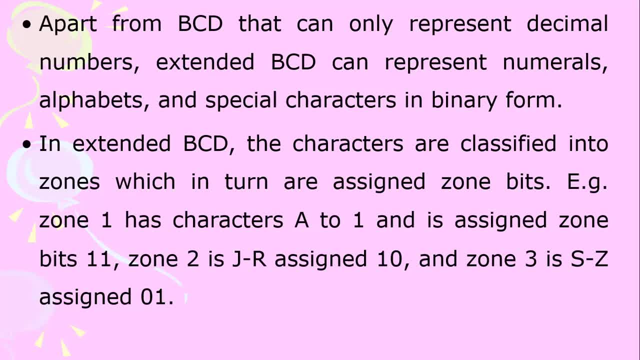 that would indicate or would mean that that character is between or is within the range A to I. While any number represented in binary, with most significant digits being 1, 0,. that would indicate that that character is within the range J to R. 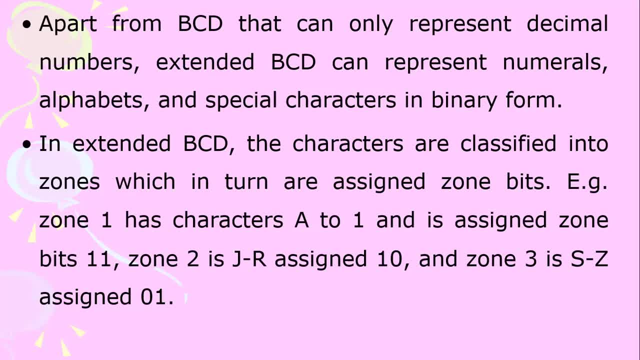 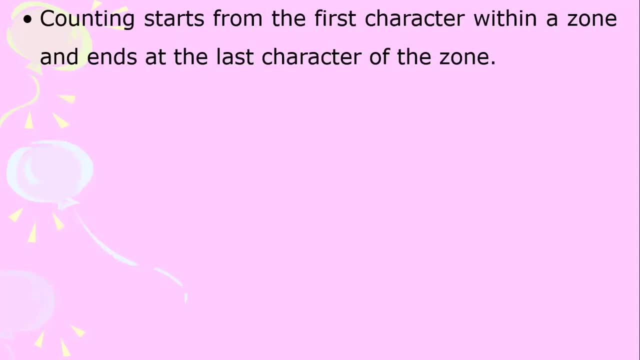 While any that is indicated or commences with the most significant digits, being or starting with the 0,, 1,, that would mean that that character is within the range S to Z. Counting starts from the first character within a zone and ends at the last character of the zone. 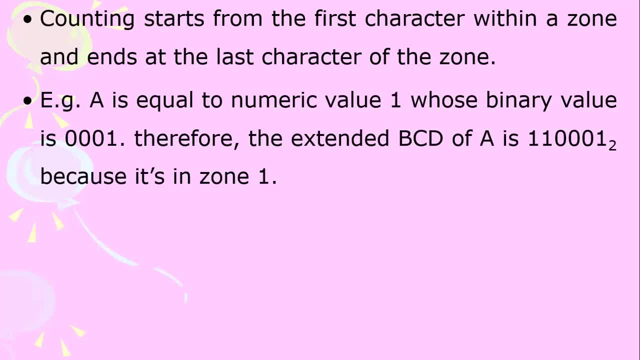 For example, A is equal to numeric value 1, whose binary value is 0, 0, 0, 1.. Therefore, the extended BCD of A will be 1, 1, 0, 0, 0, 1 to base 2.. 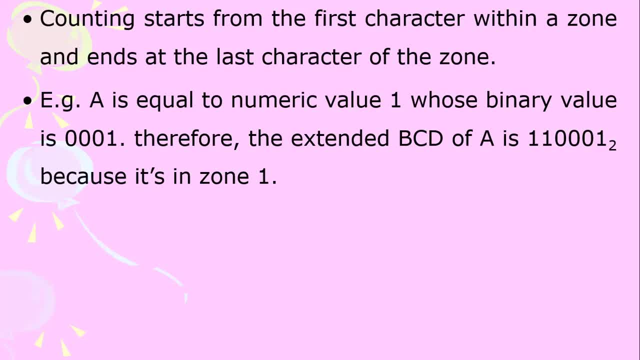 Because it's in zone 1.. Note: I have added 1, 1 on the most significant side, 1, 1, indicating that is in zone 1.. B is equal to numeric value 2, whose binary value is 0, 0, 1, 0.. 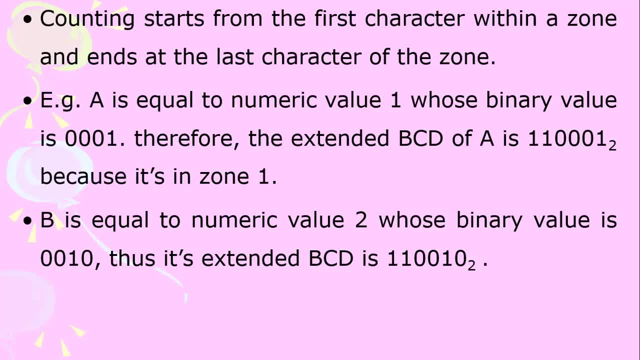 Therefore, its extended BCD will be 1, 1, 0, 0, 1, 0 to base 2.. Therefore, its extended BCD will be 1, 1, 0, 0, 1, 0 to base 2.. 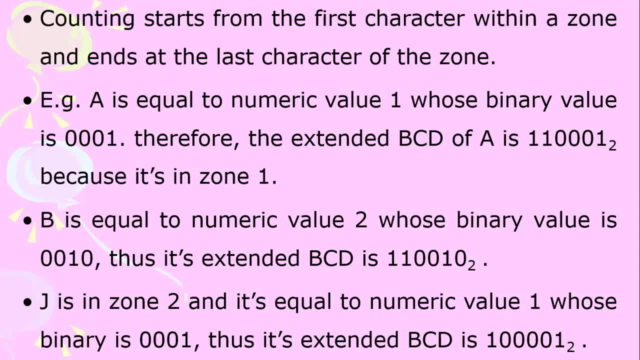 J is in zone 2 and it's equal to numeric value 1, whose binary is 0, 0, 0, 1.. So the first digit within a zone gets 0, 0, 0, 1.. Therefore its BCD is 1, 0, 0, 0, 0, 1.. 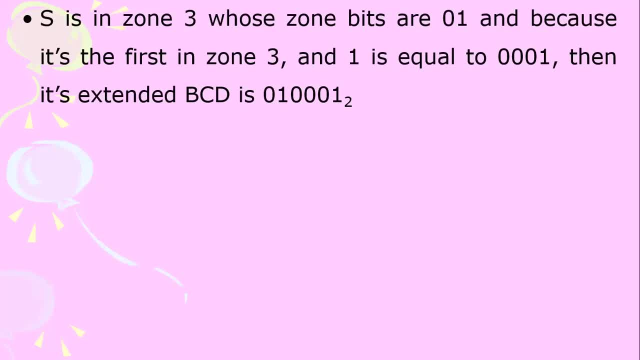 S is in zone 3, whose zone bits are 0, 1.. And because it is the first in zone 3 and 1 is equal to 0, 0, 0, 1, then its extended BCD is 0, 1, indicating the zone. 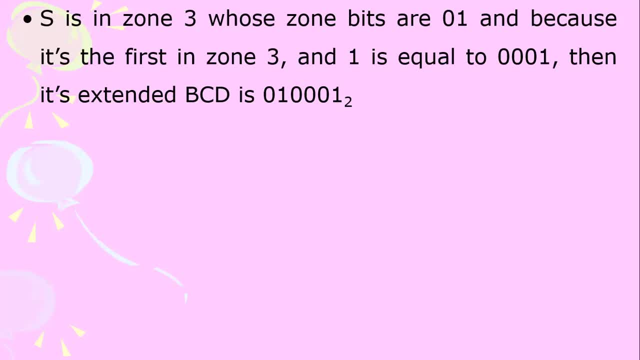 And because S is the first character within the zone, it gets 0, 0, 0, 1, which is normally equivalent to 1 in decimal, And therefore the full number of the binary digits for S will be 0, 1, 0, 0, 0, 1.. 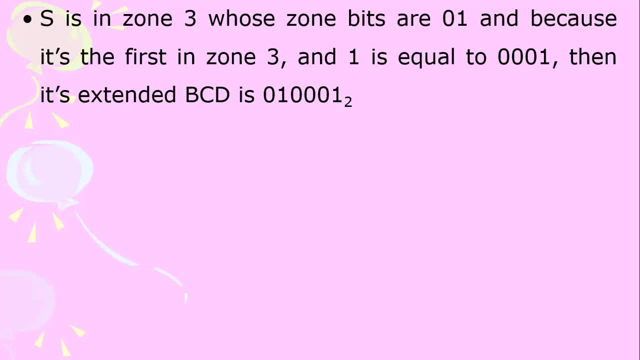 Now I am talking about the first digit in zone 3 being S. In fact, the second one is T. So how will the T be written? It is still the same. It's still the same. The zone is 0, 1.. 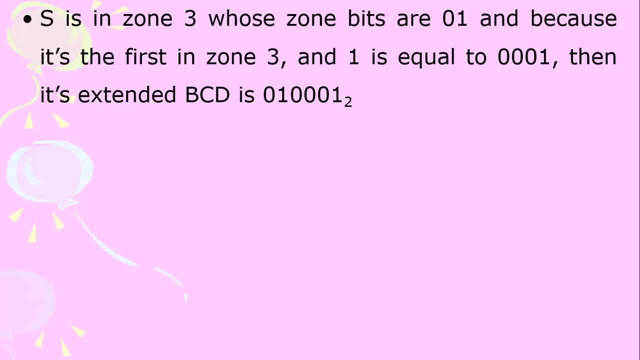 So we have 0, 1.. And then, because T is the second digit in that zone, second digit is equivalent to 2 in decimal And 2 is represented as 1, 0. Therefore, the decimal or the BCD for T will be 0 or 0, 1, 0, 0, 1, 0. 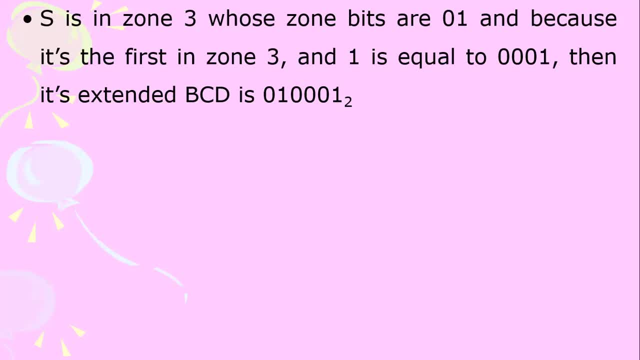 To base 2.. My dear students and the rest of the learners, in my presentation I am giving you the hint on how to get the BCDs for the various numbers. What you need to note or characters. what you need to note or bear in mind is which zone is the character? 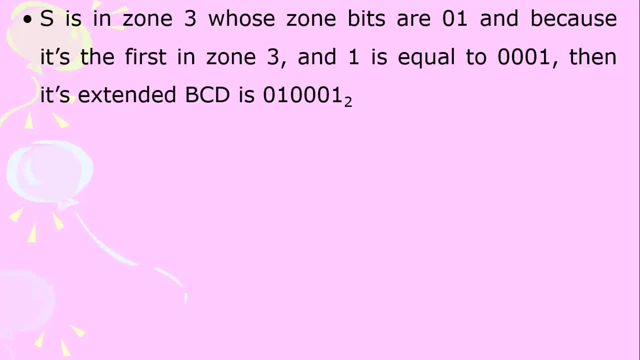 And that zone is represented by which binary values or numbers? And then what is the level of that number within the zone or that character in the zone? Is it number 1?? Is it the first one? Is it the second one? Is it the last one? 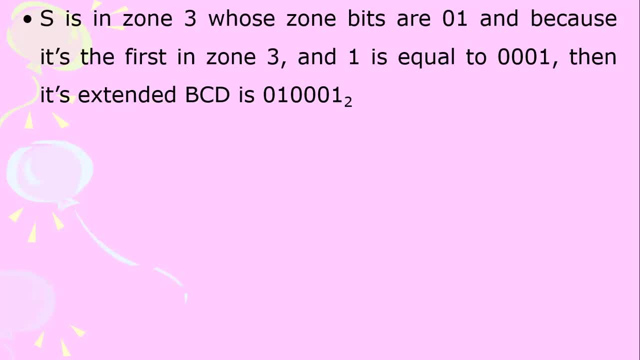 Is it the fourth one? Is it the fifth? If it is the fifth, get the decimal equivalent of 5 or binary equivalent of 5 in decimal. Then combine it with the two numbers that represent the zone When you write it in full. that will be the extended BCD for that character. 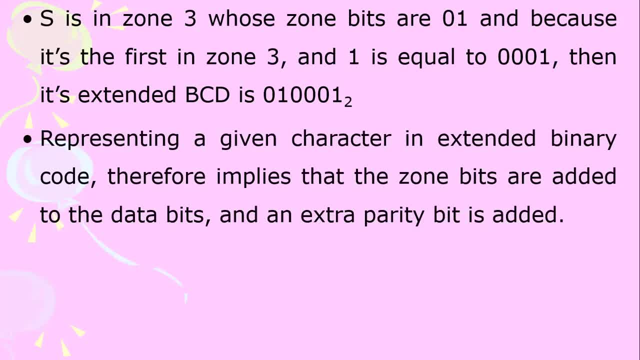 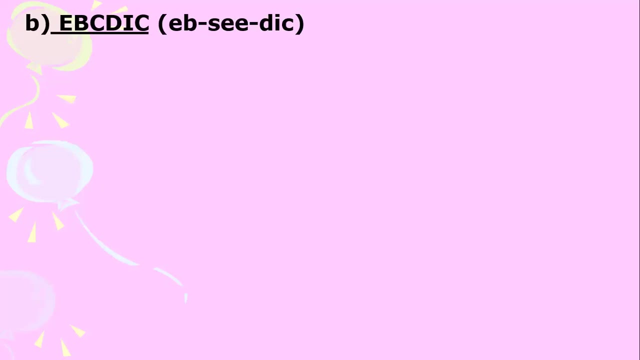 So representing a given character in extended binary code therefore implies that the zone bits are added to the data bits and an extra parity bit is added. Let's now look at FCDIC. This is an 8-bit character coding scheme used primarily on IBM computers and can represent a total of 256 characters. 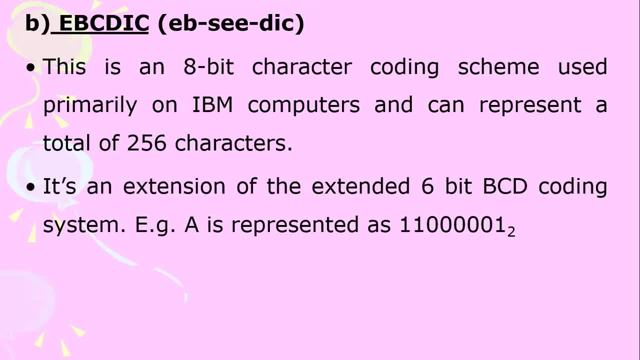 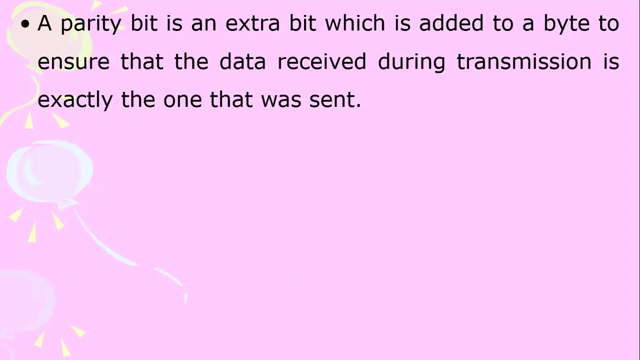 It's an extension of the extended 6-bit BCD coding system. For example, A is represented as 110000001 to base 2.. The 8-bit is used for parity checking. A parity bit is an extra bit which is added to a byte to ensure that the data received during transmission is exactly the one that was sent. 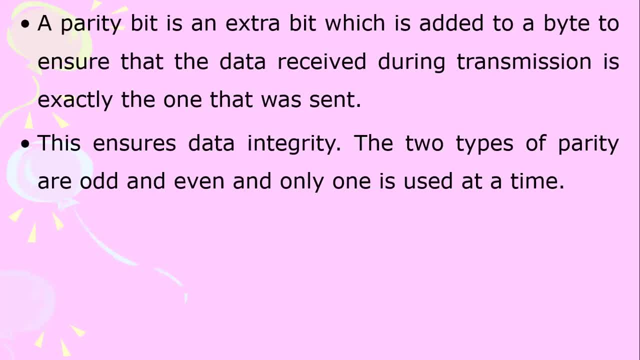 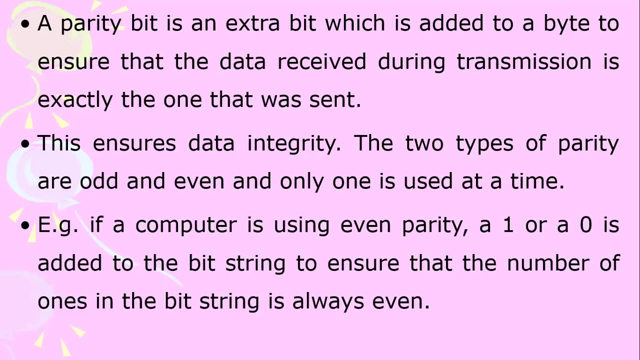 This ensures data integrity. The two types of parity are therefore odd and even, and only one is used at a time. For example, If a computer is using even parity, a 1 or a 0 is added to the bit stream to ensure that the number of 1s in the bit stream is always even. 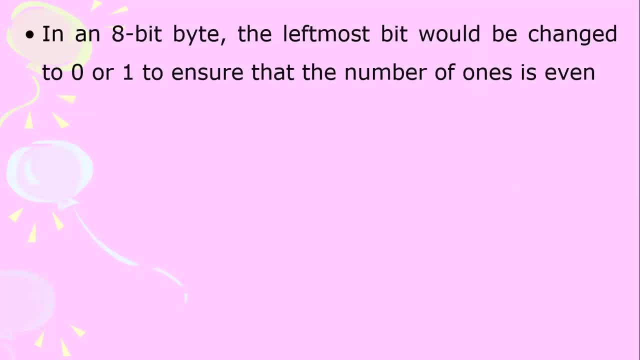 In an 8-bit byte, the leftmost bit would be changed to 0 or 1 to ensure that the number of 1s is even. For example, If you want to transmit 1100001, a 1 can be added to make the number of 1s even as 1110001 to base 2.. 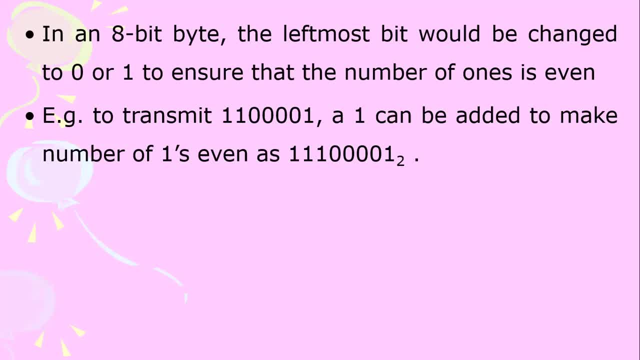 Note. Note Including the first 1. the data to sure is handed over. the suggestion would be to aren one on the most significant side, the most significant bit. So we arn 1 as the first bit on the most significant side. 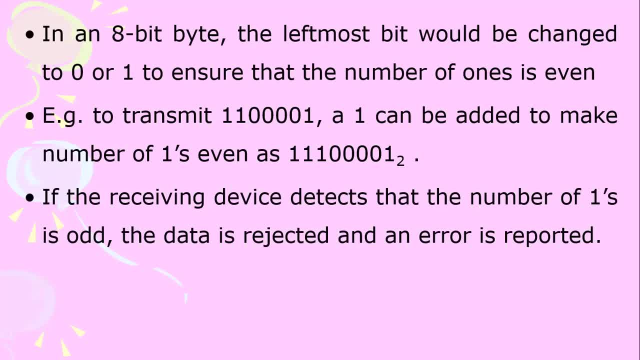 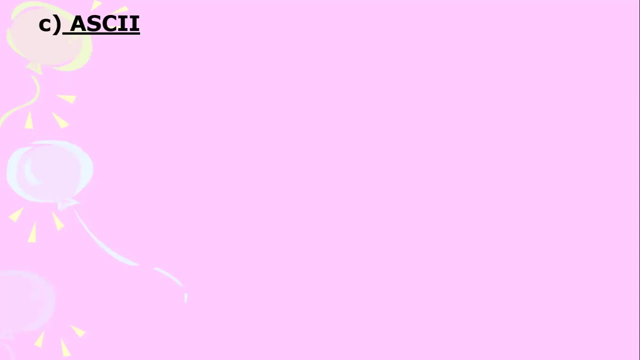 If the receiving device detect that the number of once is odd, The data is rejected and an end is hailed. error is reported. the process is similar for all parity, but done in the opposite way. let's now look at ascii. this is a 7-bit coding scheme that represents letters a to z with binary digits similar to. 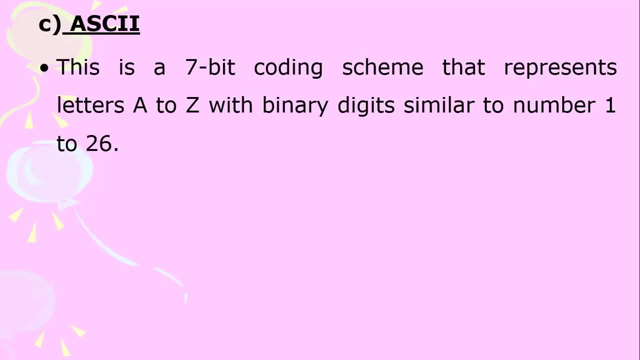 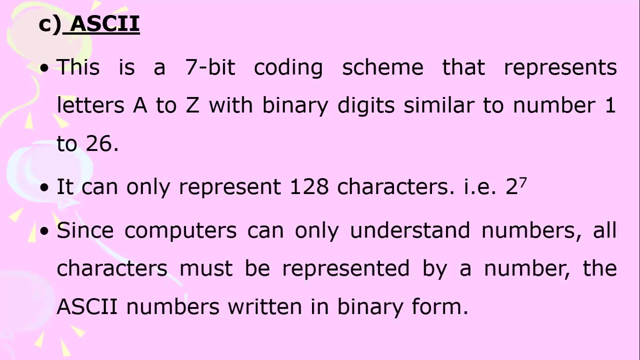 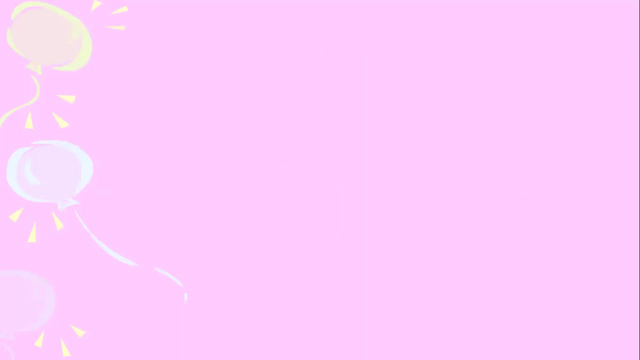 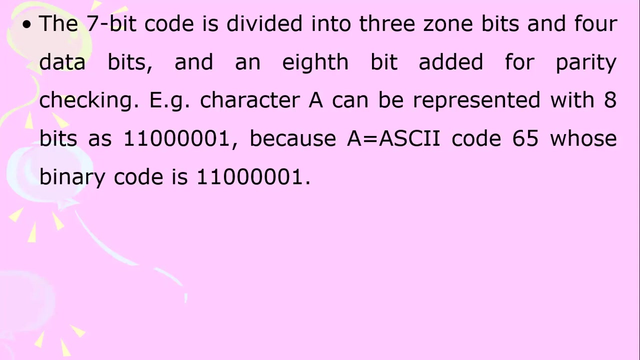 number 1 to 26.. it can only represent 128 characters, that is, 2 raised to power 7.. since computers can only understand numbers, all characters must be represented by a number: the ascii numbers written in binary form. the 7-bit code is divided into three zone bits and four data bits and an 8-bit. 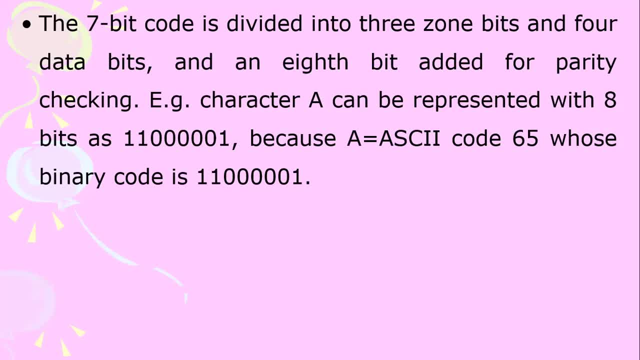 handed for parity checking. for example, character a can be represented with 80 bits as one one: zero, zero, zero, zero, zero, zero one. because a is equals to ascii code 65, and when you convert 65 decimal to binary, it gives you one one: zero-zero, zero-zero, zero one. 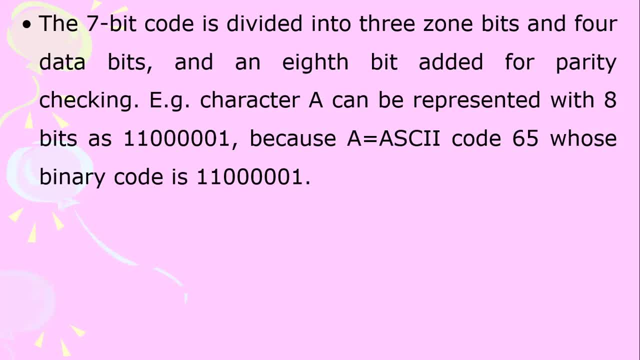 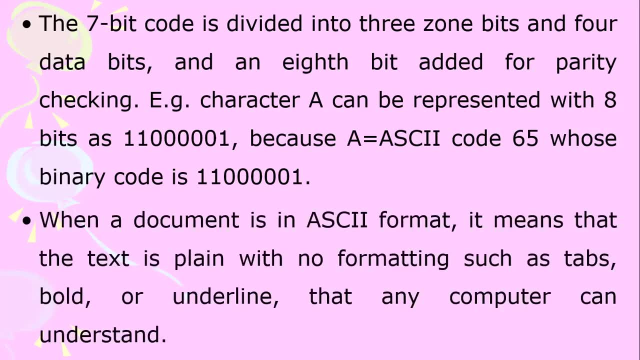 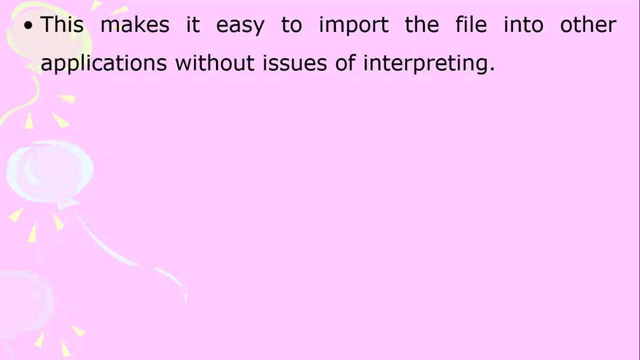 so a is equivalent of to 65 in decimal. When a document is in ASCII format, it means that the text is plain, with no formatting such as tabs, words or underline that any computer can understand. This makes it easy to import the file into other applications without issues of interpreting. 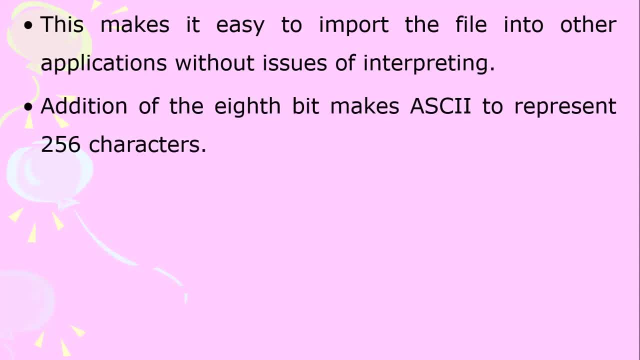 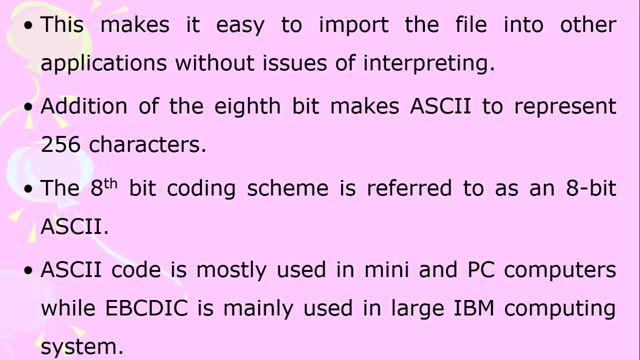 Addition of the 8-bit makes ASCII to represent 256 characters. The 8-bit coding scheme is defined too as an 8-bit ASCII. ASCII code is mostly used in mini and PC computers with Epson DIC mainly used in large IBM computing systems. 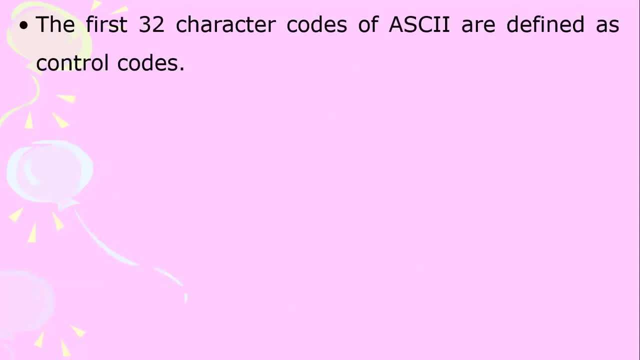 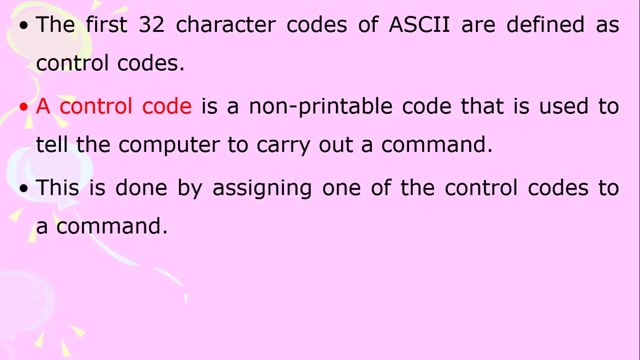 The first 32 character codes of ASCII are defined as control codes. A control code is a non-printable code that is used to tell the computer to carry out a command. This is done by assigning one of the control codes to a command. Control codes give the programmer the opportunity to assign commands to actions. 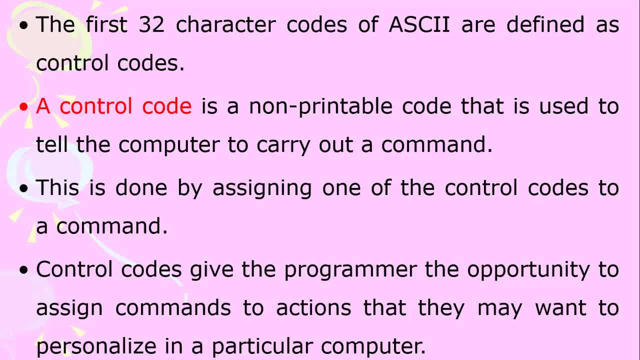 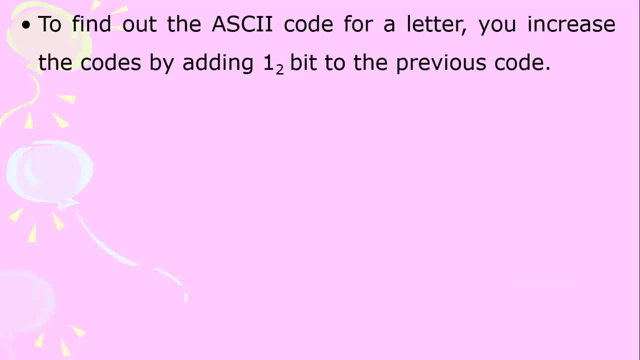 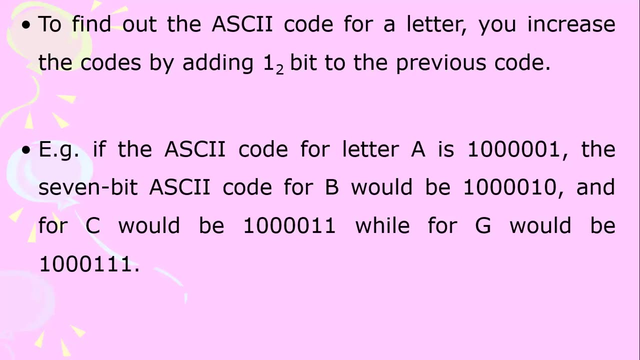 that they may want to personalize. in a computer To find out the ASCII code for a letter, you increase the codes by adding 1 to the previous code. For example, if the ASCII code for letter A is 1, 0, 0, 0, 0, 0, 1,, then the 7-bit ASCII code. 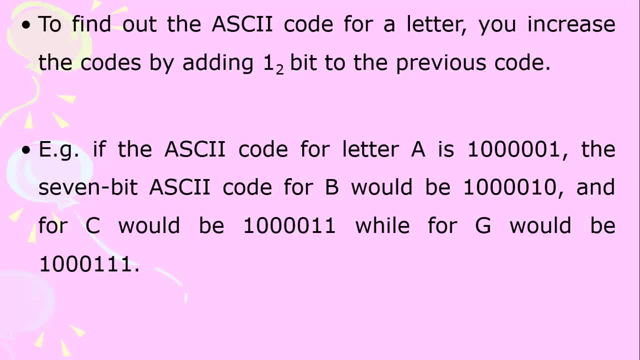 for B could be 1 0 0 0 0, 1 0.. Because 1 0 0 0 0 0 0, 1 plus 1 will give you 1 0 0 0 0, 1 0, according to the rules of binary addition that we are. 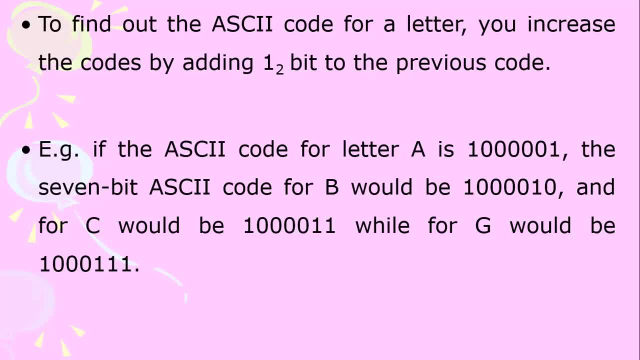 going to discuss in depth, or that I have discussed in depth in Part 2 and Part 3 of my presentations in this series that are already posted in MLSwap ICT YouTube channel. And for C would be 1, 0, 0, 0, 0, 1, 1 because it is the ASCII code. for B, added binary 1, while 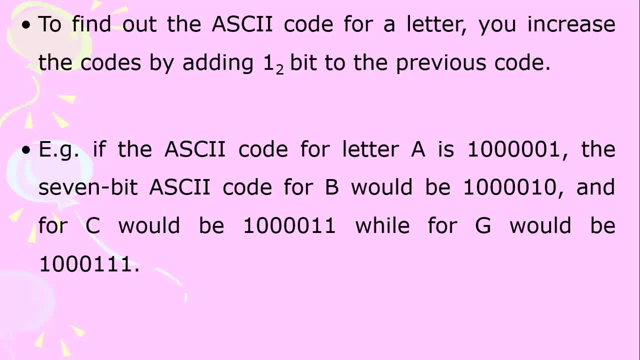 for G would be 1 0 0 0, 1.. So the sign-on code for C is 1 0 0 0, 1 1, 1.. So let's take a look at the thing right now. 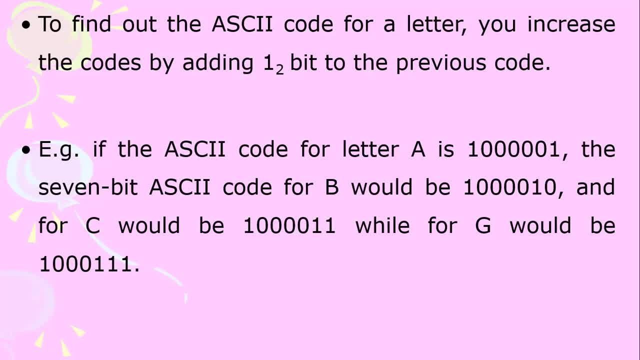 It's 1 0 0 0, 1 1 1 3 0 0 0, 1 1 1 0 0 0. 1 1 0 0 0 0 1 1. 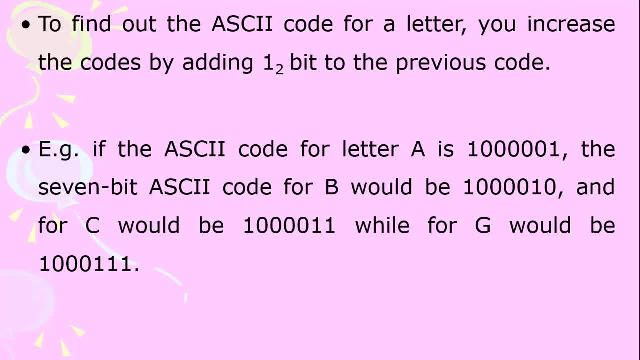 0 0 0 1 1 1 00. 0 0 0 1 1. My dear students and the rest of the learners, for you to get deeper understanding about these addition and these representations, make sure you have listened to Part 2 of 3 and Part 3. 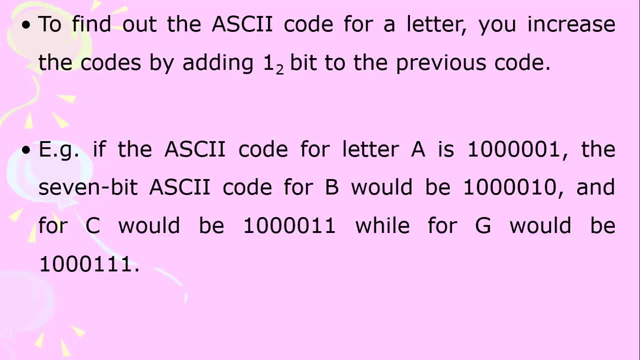 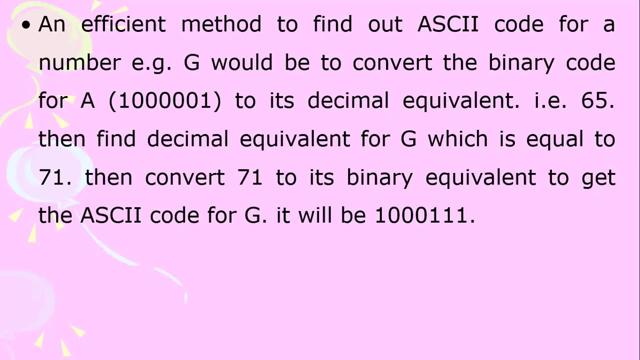 three of my presentations under this topic, or data representation in the computer. An efficient method to find out ASCII code for a number, for example G, would be to convert the binary code for A, that is 1, 0, 0, 0, 0, 0, 1, to its decimal equivalent. 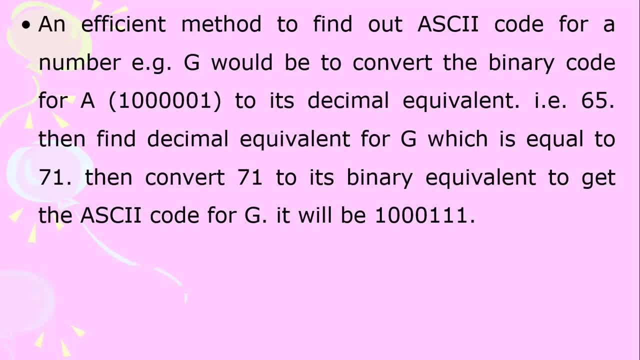 that is 65.. For B, it is 66.. For C, 67.. For D, 68.. For E, 69. F, 70., G, 71. So once you have known the equivalent of A in terms of decimal, 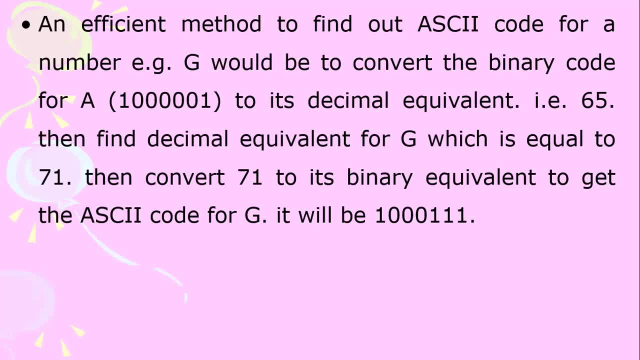 and you know it is 65, convert 65 decimal to its binary equivalent And that will help you to be able to get the ASCII code for a character. Then you find decimal Equivalent for G, which is equal to 71. Then convert 71 to its binary equivalent. 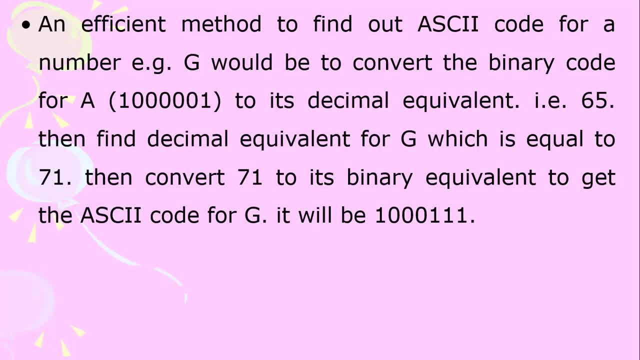 to get the ASCII code for G. In other words, I'm simply saying that because you know that the equivalent of character A is 65, just count those numbers of decimals, or decimal numbers from 65 upwards to represent, to be able to know the decimal number that is equivalent to the. 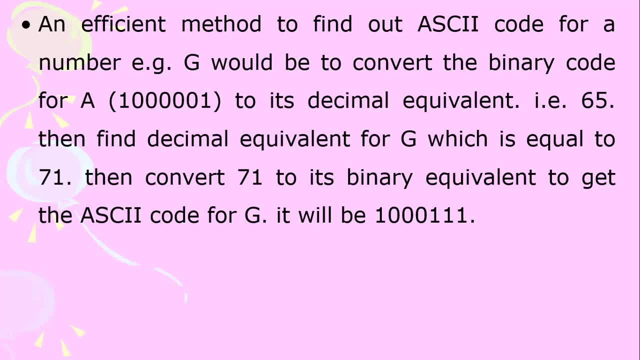 character that won't represent. If, for example, you want to get the equivalent binary equivalent in ASCII for character G, for example, and you know A is 65. So just count from 65 to G: 65 equals to A, 66 to B, 67 to C, 68 to D, 69 to E, 70 to F, 71 to G. 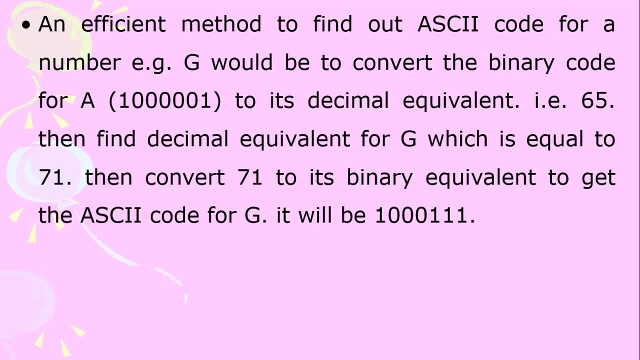 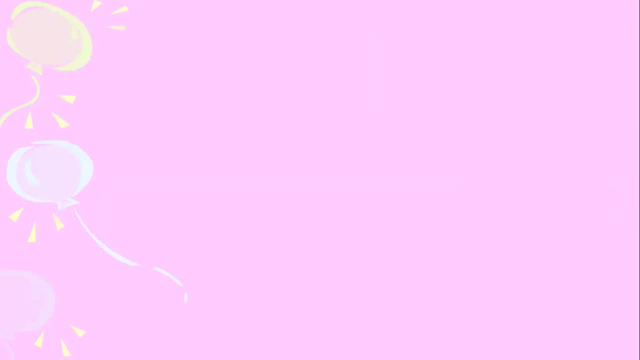 Then convert that 71 to its binary equivalent and you'll be able to get the ASCII code for G, which in this case will be 10.. 00111.. Let's now test our brain a little. Represent meme, In other words, represent meme, which is my name, using ASCII code. 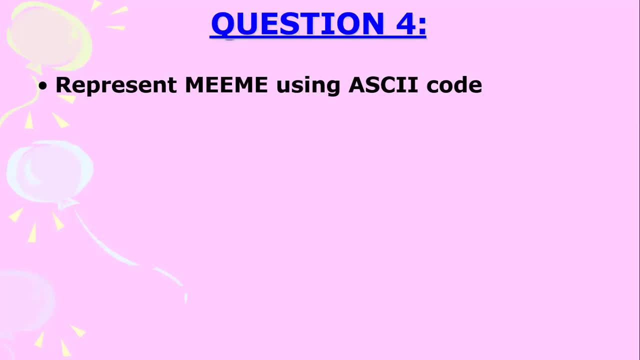 Represent meme using ASCII code. How do we go about it? This is what to do. If A equals to decimal equivalent of 65, then decimal equivalent for E is 69 and M is 77. So you count from A being equal to 65.. 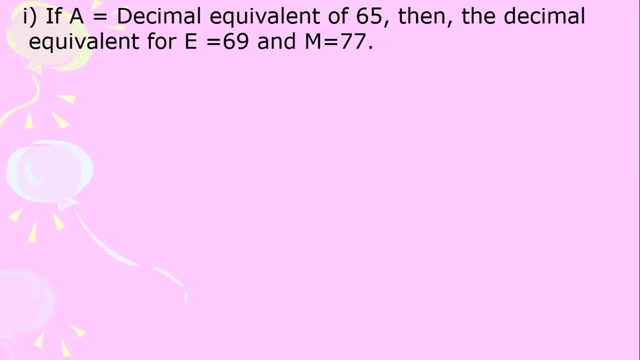 B 66.. E 67. All the way: 001.5.. the way when you get the equivalent for E, that's 69, you note it down. And then equivalent of M is 77, note it down. Once you have noted them down, then get the undecimal or binary. 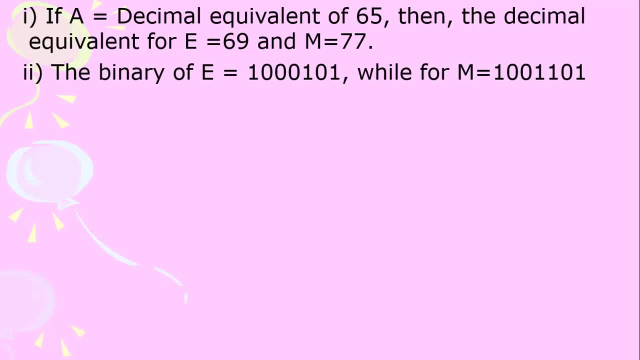 equivalent. So the binary equivalent of E is 1 0 0 0, 1 0 1.. That is, you convert the decimal number 69 to its binary equivalent and that binary equivalent will be equal to the ASCII letter that we want to represent, which is E, while for M is 77.. 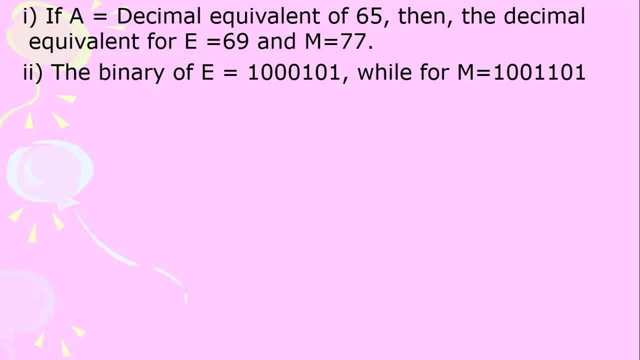 Represented in its binary equivalent, which will be 1 0 0. 1 1 0 1.. My dear students, just as I've said, don't worry, Access my Part 2 of 3 in this topic from MLSwapIC YouTube channel and Part 3, and you'll be able to. 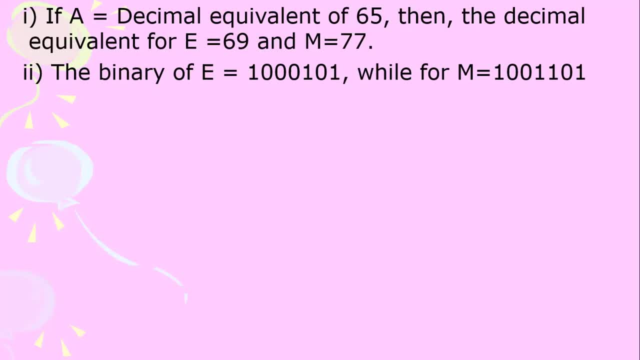 know how to convert one number system to another, including the decimal that we're talking about, to its binary equivalent and then to its equivalent ASCII character. Therefore, MEME can be represented in ASCII as follows: M is equal to 1 0 0, 1 1 0 1.. 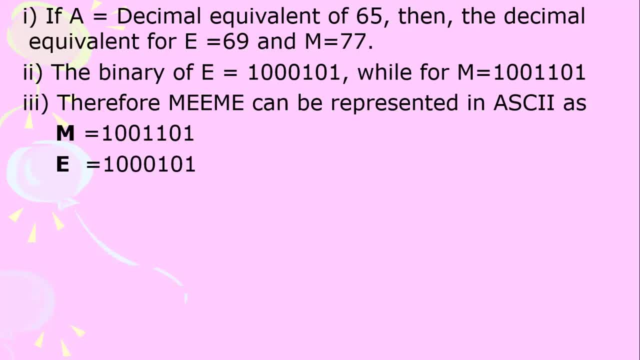 The first E is equivalent to 1 0 0 0, 1 0, 1.. The next E is equivalent to 1 0 0 0, 1 0, 1.. Then M or M is equivalent to 1 0 0, 1, 1 0, 1.. 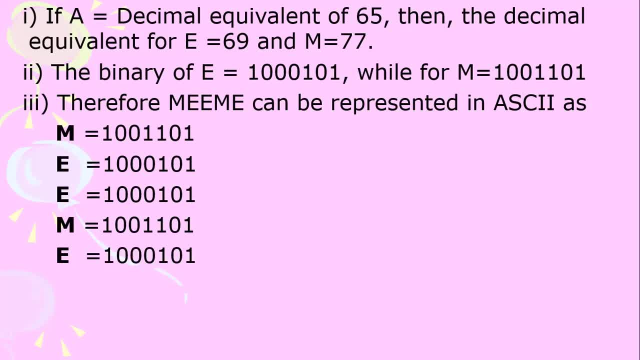 And the last E is equivalent to 1 0 0 0, 1 0 1.. And therefore Meme will be represented as follows in ASCII: 1 0 0.. 0 1 0.. 1 0 1, 1 0 0 0.. 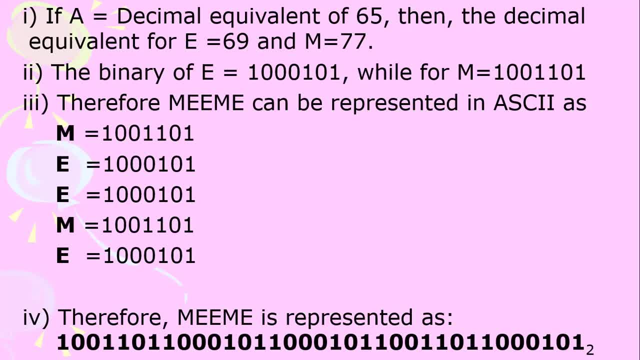 1 0 1 1 0 0 0.. 1 0 1 1 0 0. 1 1 0. 1 1 0 0 0 1 0 1.. This too. 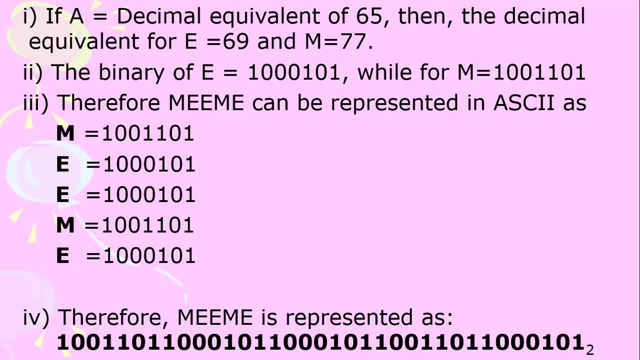 I repeat, Meme. That is the combination of those characters and arranged in that order, Starting with the first letter M to the last letter E. you represent it as, or you join those bits as follows: 1 0 0. 1 1 0.. 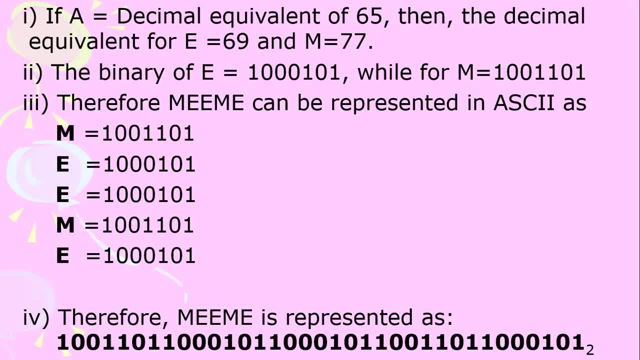 1 1 0, 0 0.. 1 0 1 1 0, 0.. 0, 1, 0, 1, 1, 0, 0, 1, 1, 0, 1, 1, 0, 0, 0, 1, 0, 1..